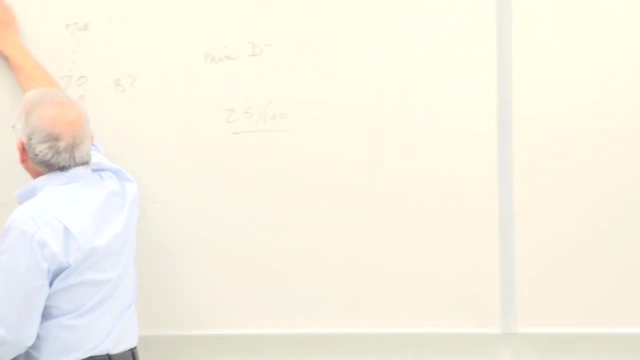 What subjects you want reviewed? Finding stresses from strain values, In other words, the stress-strain diagram. Is that what you're talking about? Very simple, We'll do that, Okay. What else? More circle, More circle. Okay, Let's write that That's always one of the choices. 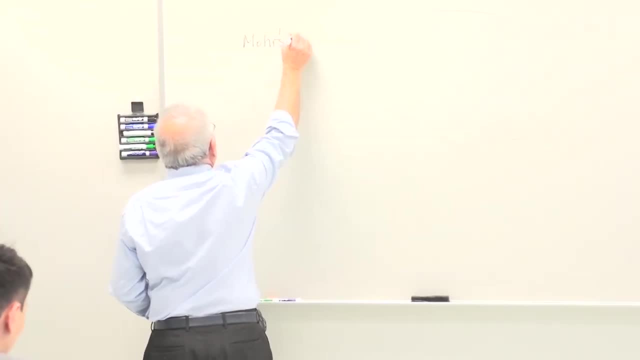 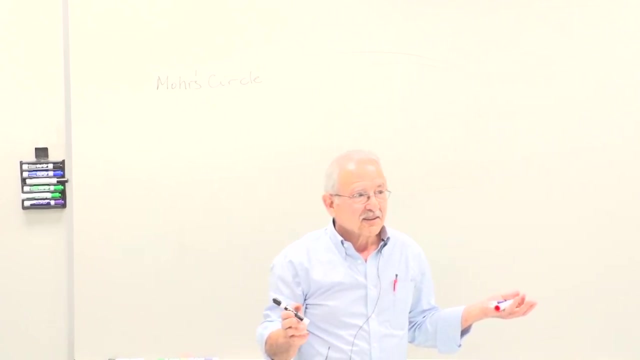 Okay, Give me two more options. What else? So, if you don't want any other subject reviewed, if I give you a quiz right now on combined loading, it's okay. I doubt that. So again, Again, don't be bashful. 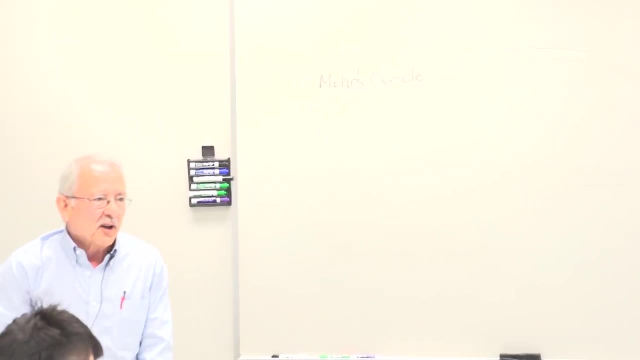 You have to answer my question. You don't have to, really. I mean, you can just sit there and look at me, But remember, if you don't answer my question, I don't know what you don't know. You have to tell me what you don't know, what you got questions on. 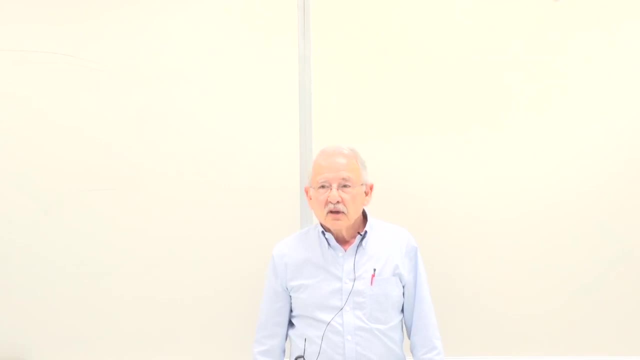 And we'll answer those questions. So anybody else want to be brave enough to say something? I'm sorry. Combined loading okay. Anything else, Castigliano's theorem. we will do in this class independent of what you studied. In fact, the emphasis will be on Castigliano's theorem. 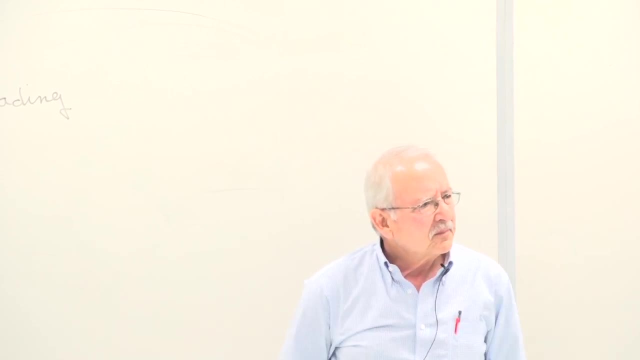 Anything else- Transverse, shear and bending, okay? Okay, let's take a look at these and then, if we have more time, you can come up with other subjects as well. Take these one by. actually, I'll answer your question first, because that's simple enough. 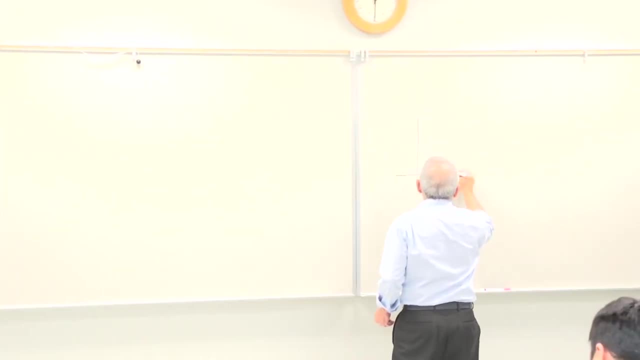 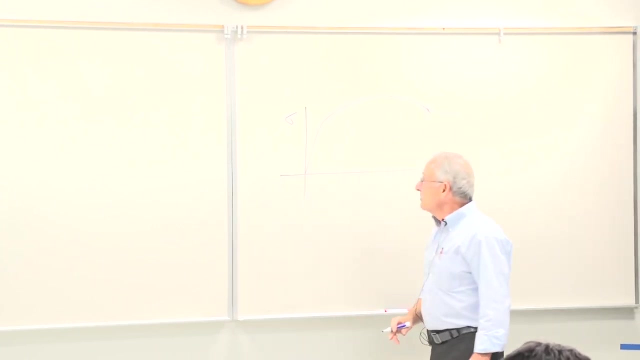 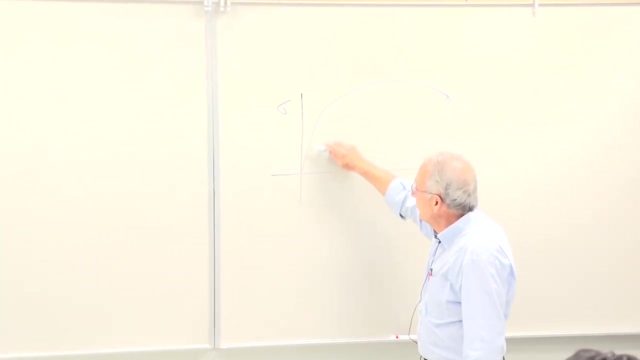 If you're asking how we find stresses from strains and if I have misunderstood your question, please let me know. That's a stress-strain diagram for a ductile material. A part of that diagram is linear and elastic. In other words, when you load the material in this section to some value, 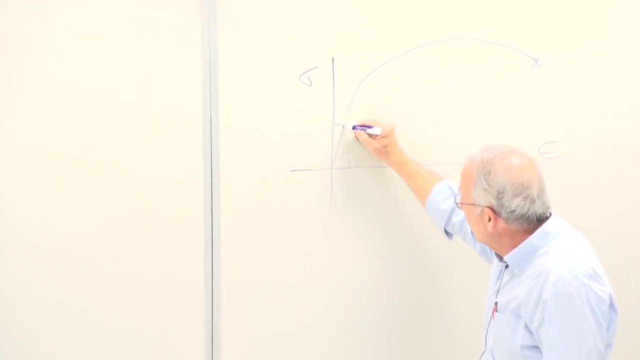 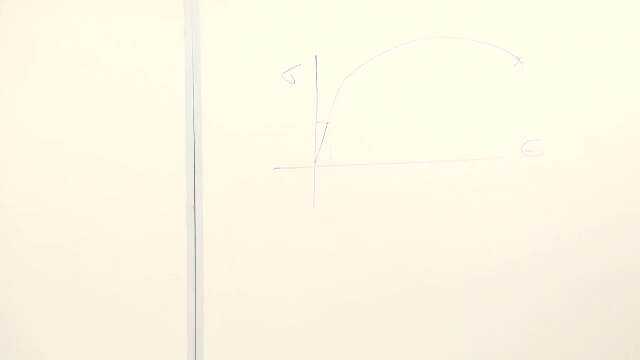 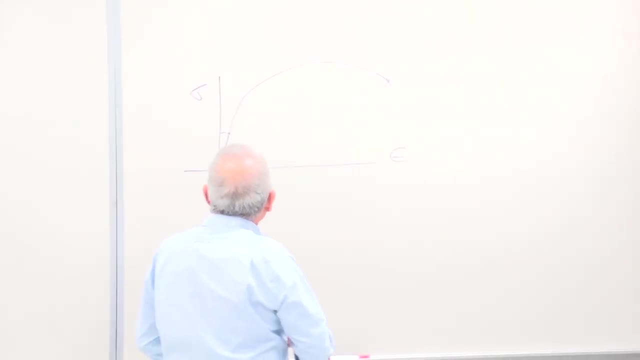 Okay, Okay, Okay, Okay, Okay, Okay point. Actually, there are three points. One is called proportional limit, The next one is called elastic limit, And then we define this third point as the yield point, And it is in a stress-strain diagram such as the one that I have on the board. it is conventional. 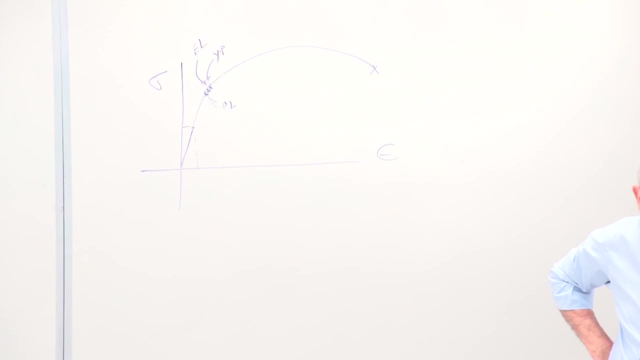 It's arbitrary- Well, not arbitrary, but conventional- In that we say that the yield strength of the material is a stress for which the strain is two-tenths of a percent- 0.002.. It's called two-tenths of a percent offset yield strength And that's what we use: The stress-strain. 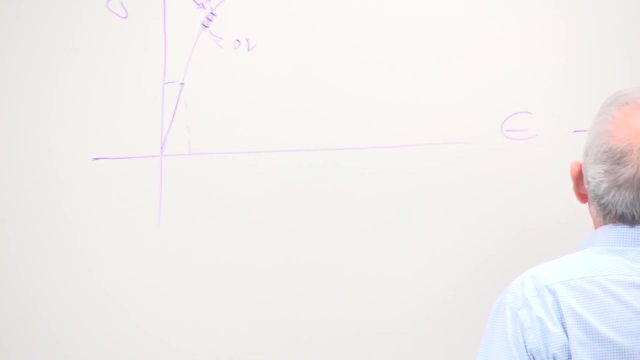 diagram in the material may look like this as well. If you're in this, you just passed that point. You have definitely passed the 0.002 mark. So we say this is the yield point of the material And there's a little upper yield point and 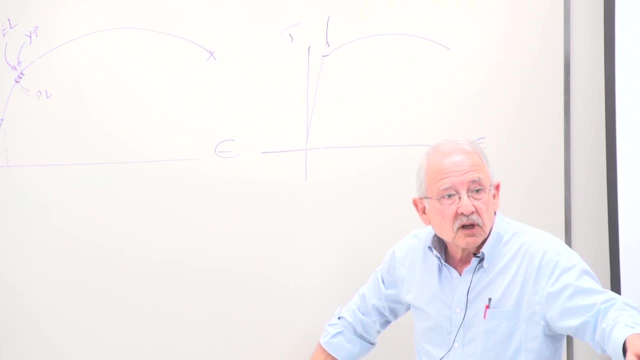 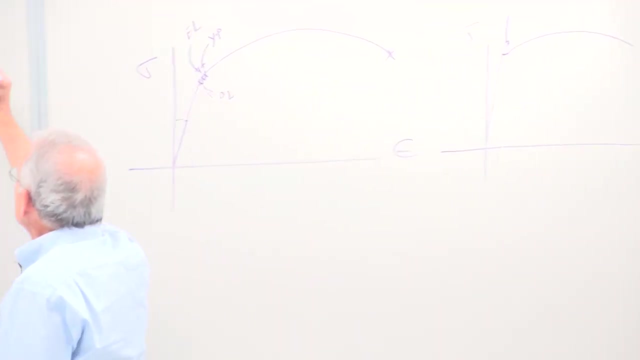 lower yield point. Those of you who have taken materials ME315, probably saw that in your studies. If the stress or strain is in the linear elastic region, then you can use this equation. Where E is the slope of that line, That's where stress and strain are proportional. So if you have strain you can use that equation. 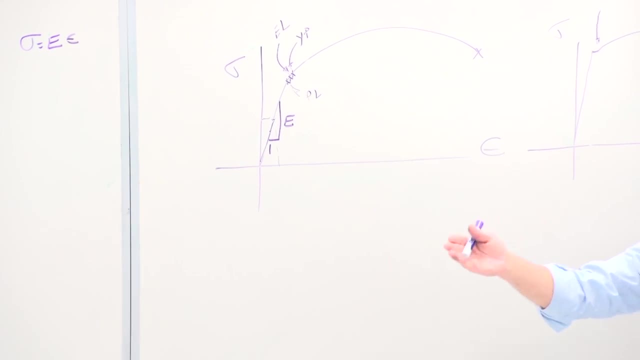 and find stress, and vice versa. Alternatively, if you know the value of the strain, you can put it in here. come up and read the value of stress. Either of the two will give you the answer. Okay, Okay, probably with some approximation, because you're 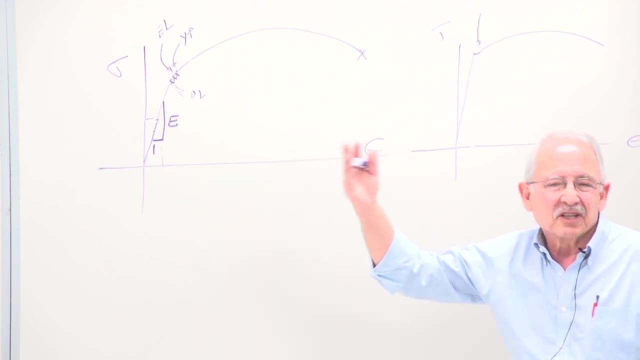 going to have to read a curve, That one, I don't want to say it's more accurate, but you'll get a number that matches the equation. If, however, the strain is not in the elastic region, you have strained the material past the elastic limit. 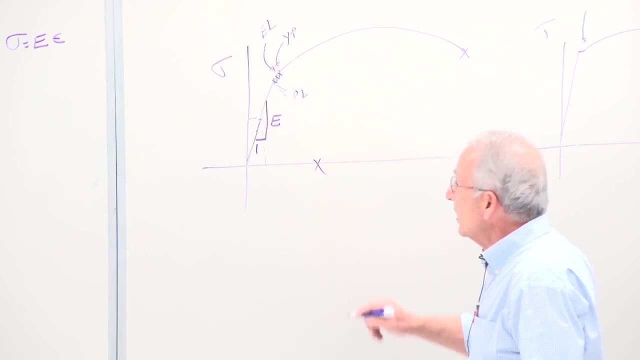 and the yield point, and you're out here somewhere. that equation is no longer valid. You cannot use that equation anymore. The only way to do it, if you have the stress-strain diagram, is go up here, come in here and read the value of. let's say: 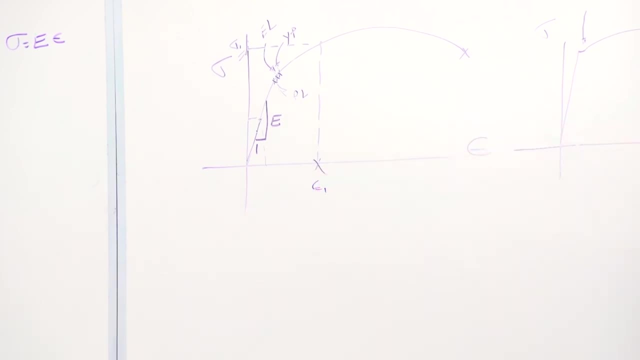 sigma 1, epsilon 1.. Is that your question? Yeah, that's what I'm trying to say, Are you sure? OK, All right, But that's about it. Just make sure you don't use that equation in an inelastic region. 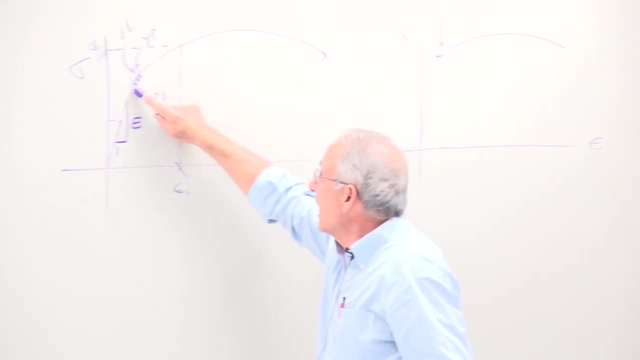 You have to use the graph, or sometimes you find actual equations for that part. Then you can use that equation. Of course it will not be linear, It will be a nonlinear equation, But you can use that equation. OK, So more circle. 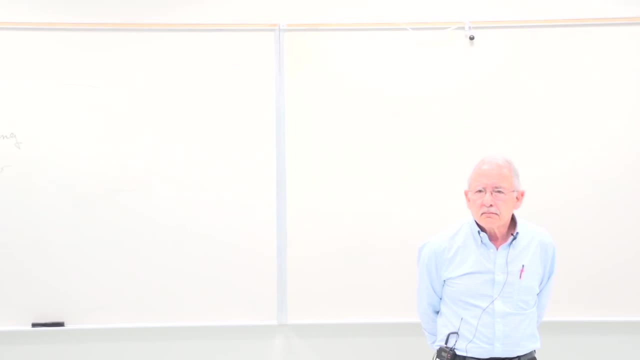 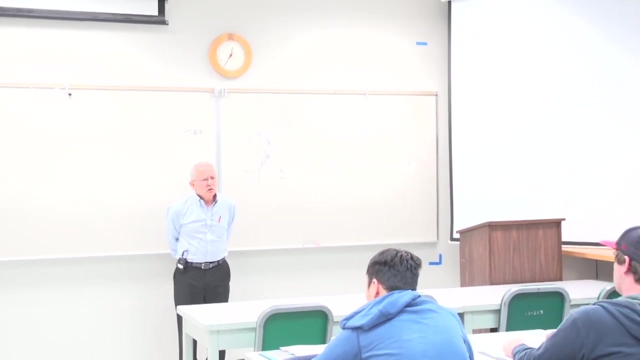 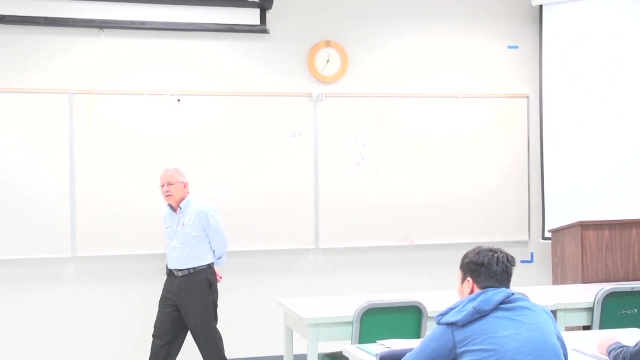 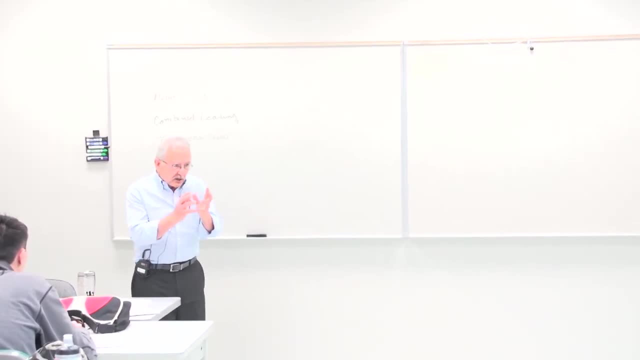 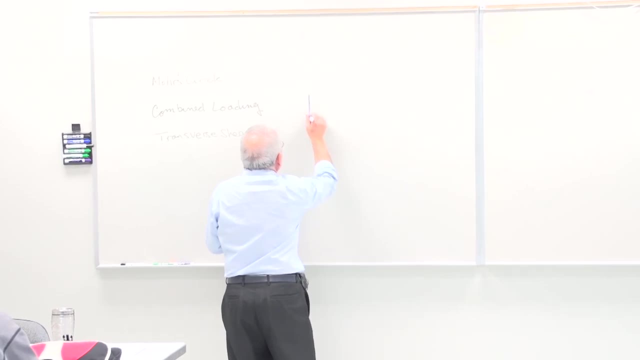 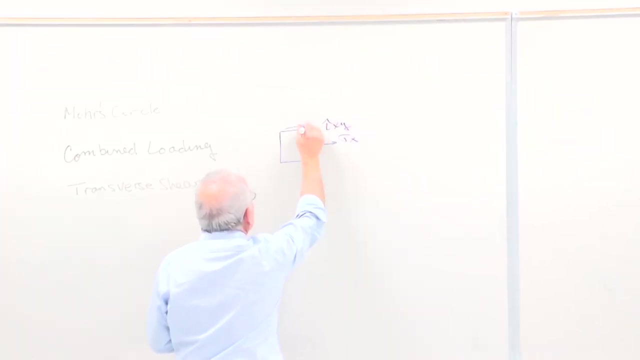 That's right. Yes, That's correct. So let me- and both answers are very correct, very good, Let me. let me show you something You're familiar with, this Regular stress element, right? You've had that in 218 and 219 and all of that. 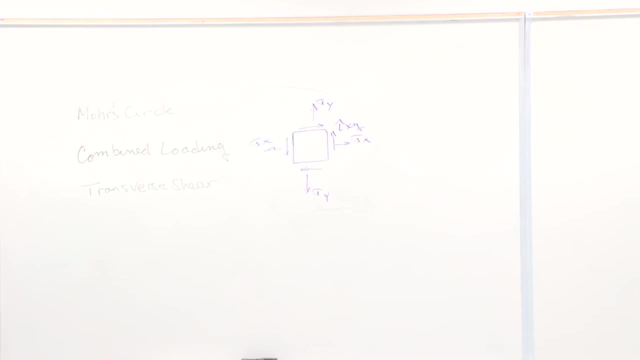 And that's the starting point for drawing more circle. These are stresses where, At the point, you've solved the problem Point, That's at the point where you want to solve the problem, whatever Structural point if you will. These are stresses at one point in the material. 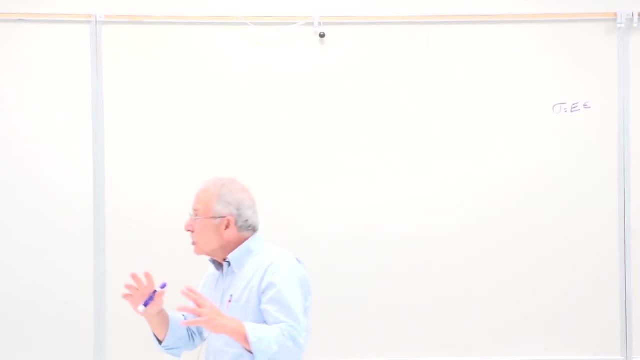 This is not an overall stress, One point in the material. So this square here shows you a point, For example, similar to this: Let's say you have all these forces acting on this object, whatever it is. we pick this point and we represent that point. 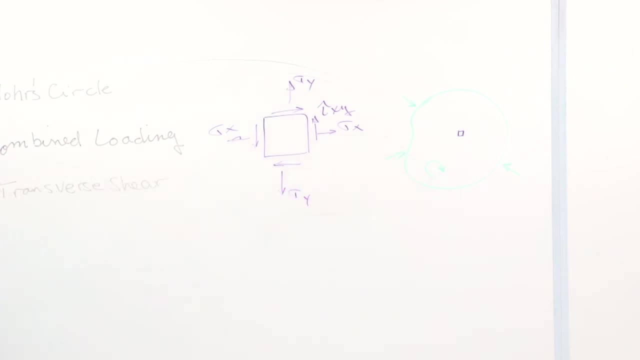 by this little square. The stresses on the sides of this little square are shown here. These dimensions are very, very small. This is a point. So, apparently, having this, we've taken our x and y axes like this agreed: Horizontal x-direction, vertical y-direction. 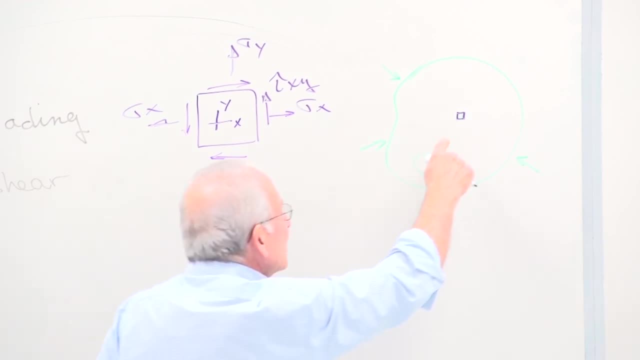 But what if, instead of drawing a square like that at that very same point, I draw the square like this? I don't want to draw it right Right on top of that point, but this is for the same point. What if, instead of that, I draw a square like that? 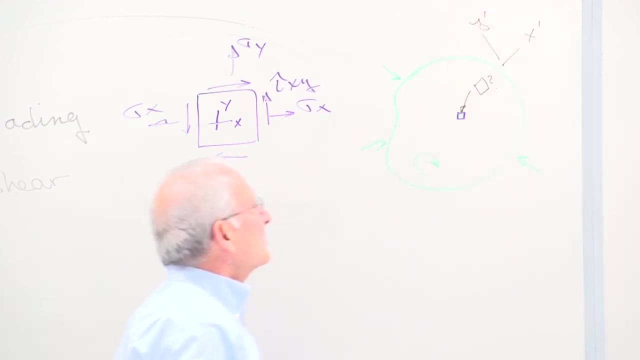 And here are my axes: x prime, y prime. That's at this, that very same point. I'll give you a simple example that you're all familiar with. If this is 10 ksi stress- And I make a cut here- 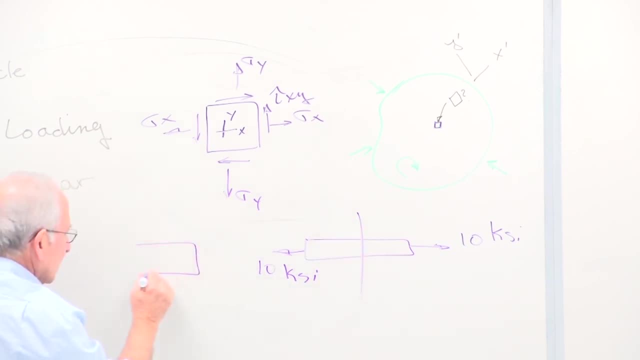 And I take a look at this cut section. What's this stress here? 10 ksi, Because assuming that the dimensions have not changed- I know I didn't draw it to the same size, But assuming that the dimensions have not changed, it's the same force being transmitted. 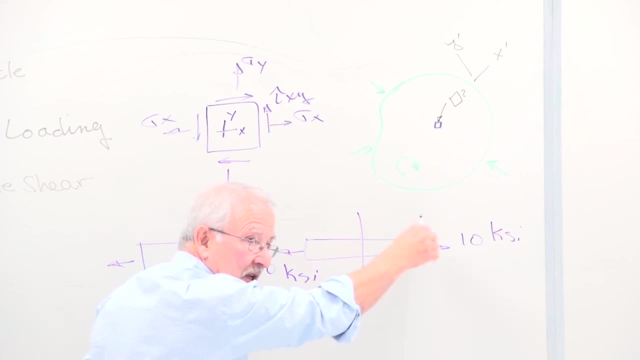 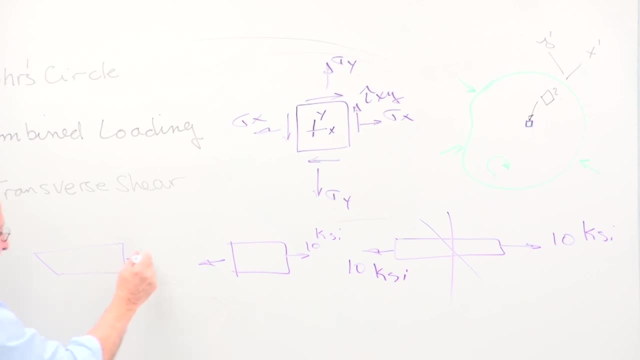 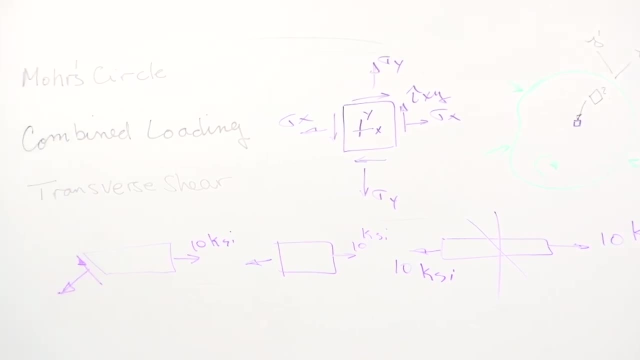 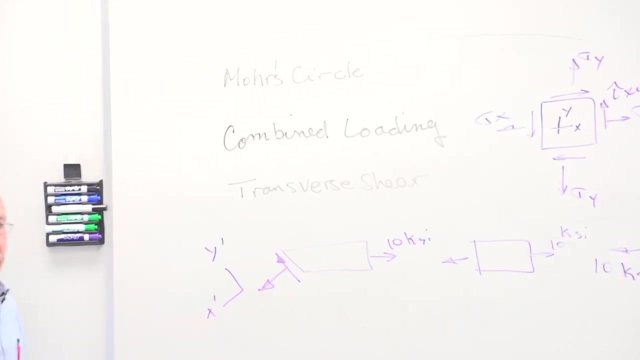 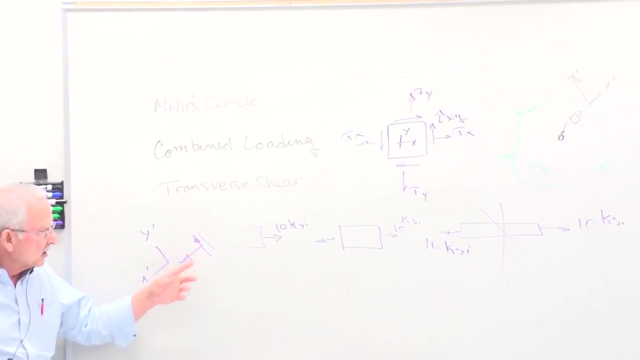 I'm looking at this, I have these two stresses- This is my x prime and y prime direction that I have shown there, This stress, the normal stress here, call it sigma prime, tau prime. Coming to this point, The flow is critical. 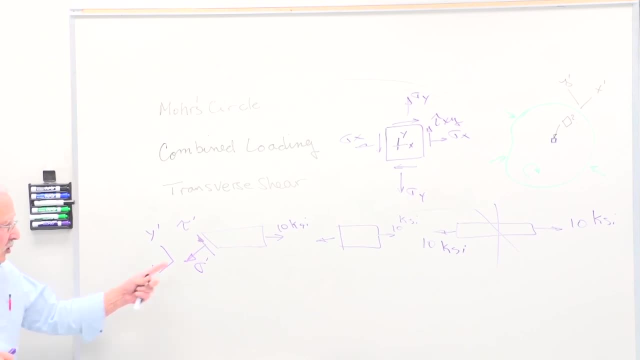 tau prime. The normal stress here is no longer equal to 10 ksi. It's something else, And as I change this angle of cut, this angle, theta, that stress changes. Therefore, the normal stress and the shearing stress are functions of this angle, If we can go from. 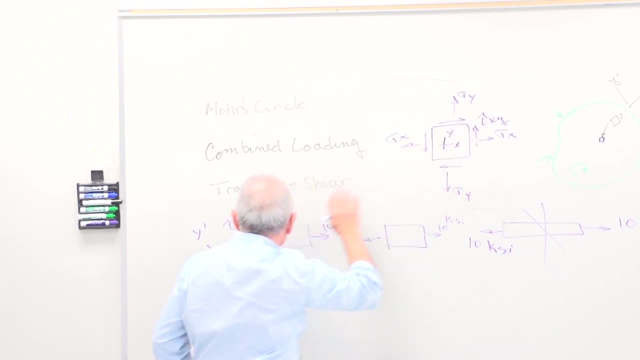 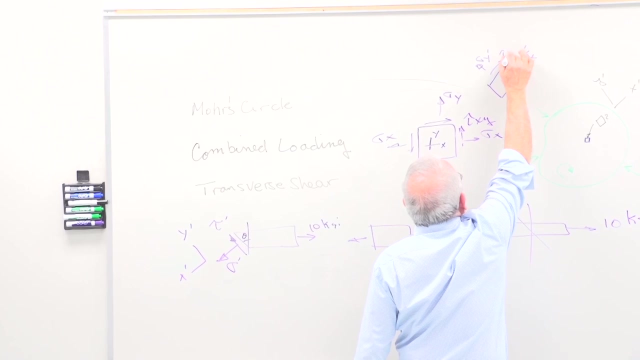 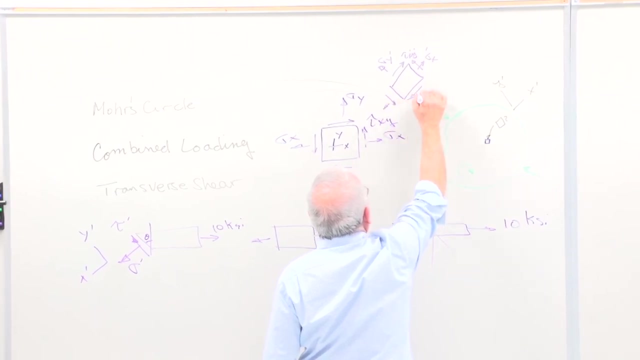 this set of stresses to that set of stresses, in other words something like this: Sigma x prime, sigma y prime and tau xy prime, And the same on these sides, of course. If I can come up with a set of equations, that will take me. 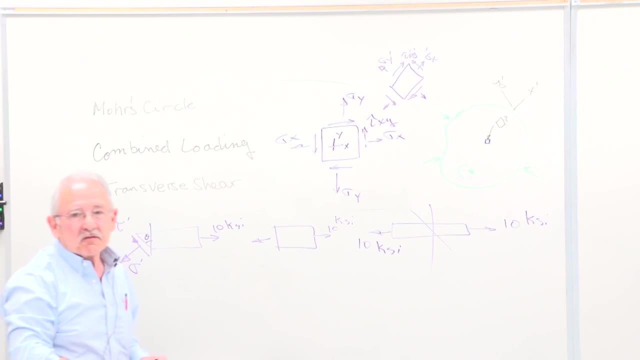 from this set of stresses to this set of stresses, mu sigma x prime and tau xy prime, and the same on these sides. of course, If I can come up with a set of equations, that, And from this set of stresses to that set of stresses, I will have found the transformation. 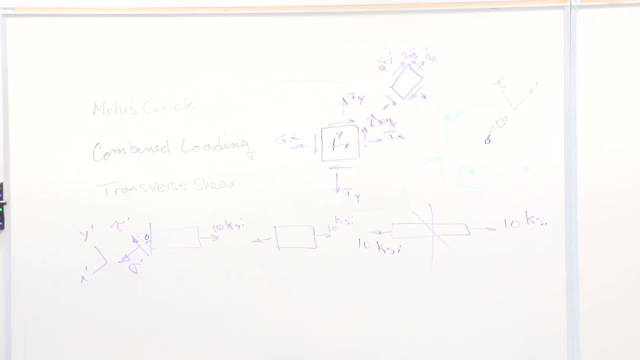 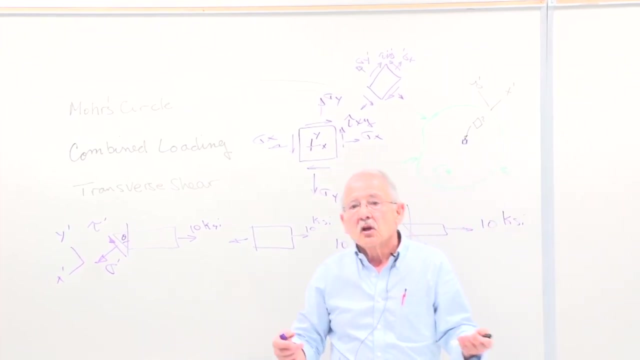 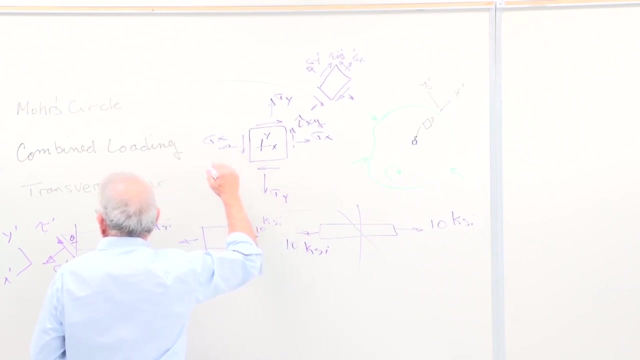 equations for stresses. So these are all stresses at the same point at various angles, And the transformation from one set to the other set is called stress transformation. How do you do that? Well, pretty simple. What you do is you take that element and you say: what is this angle here? theta with: 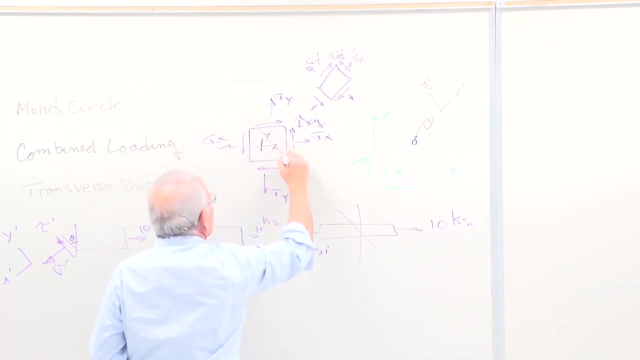 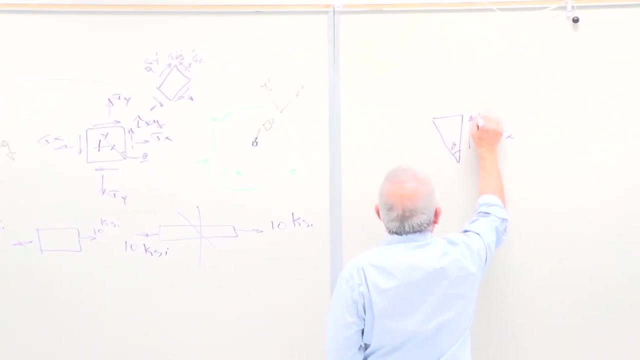 the vertical. So there's the angle theta And we take a look at this little triangle. we have sigma x, tau xy, tau y, tau y, tau y. sigma y, sigma x, prime, tau x, prime y, prime. 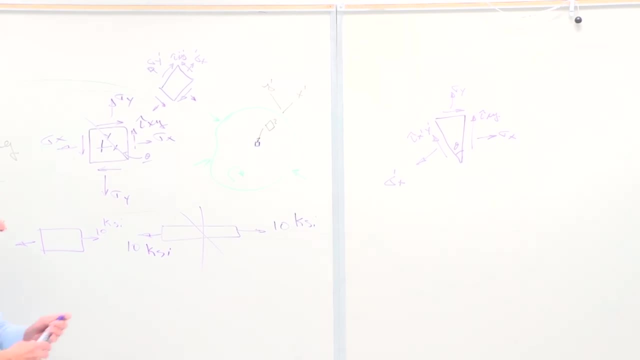 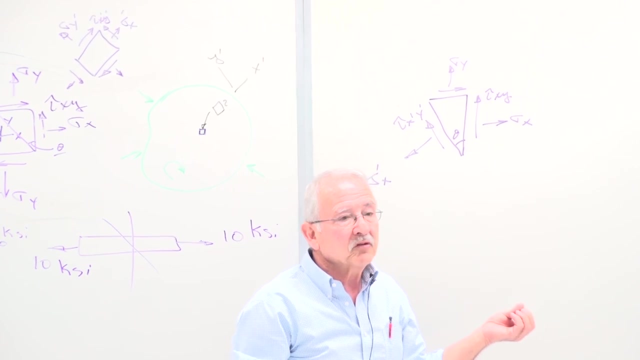 This is all at one point. Once we look at it like that in these directions, once we look at it like that in those directions, But it's all at the same point. To get to the transformation equations, All you have to do is use equilibrium equations. 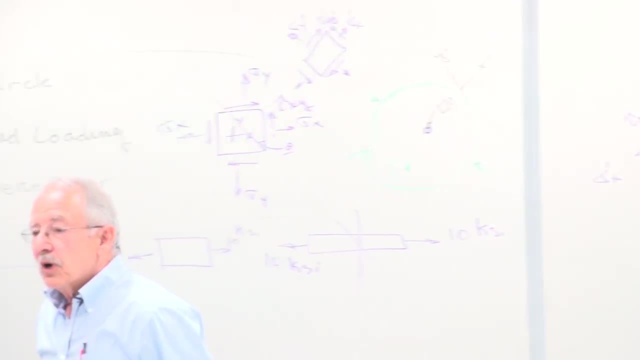 This tiny body here which is at a point must be in equilibrium. Remember that equilibrium means that the summation of forces are zero, not stresses. Don't add stresses, Okay, You must add forces, meaning that if you want to use equilibrium equations, you have to. 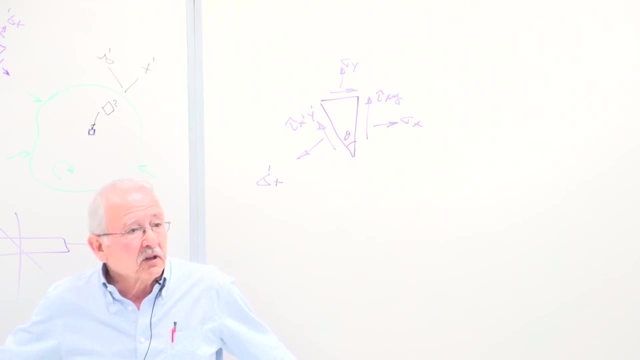 multiply each stress by its respective area on which it acts. So, for example, to find the force that acts on this area, you multiply sigma x by this area. Remember that this is an area into the board. You say: well, what are those areas? 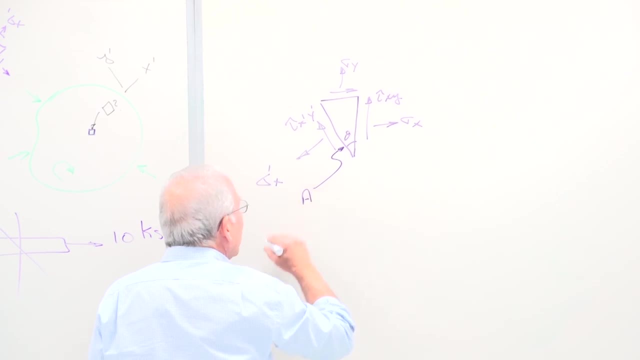 Well, it really doesn't matter that much. I can call this area A, Then that area would be A cosine theta. That area would be A sine theta. The thickness is the same in all cases. You multiply them by their respective areas. 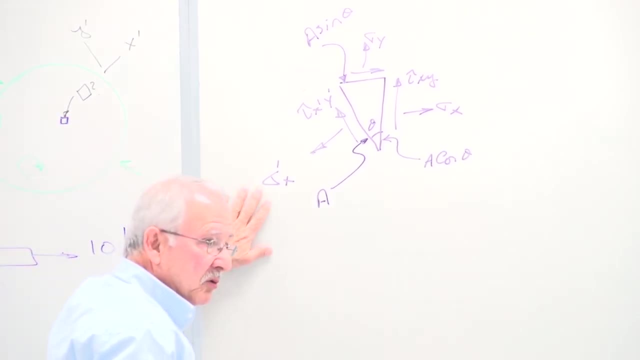 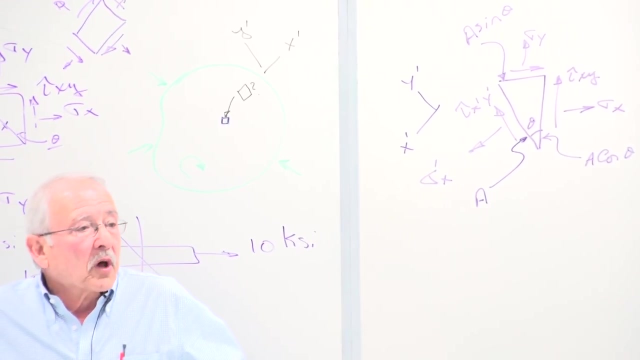 Write an equilibrium equation in the expression: Okay, Okay, In the x prime direction. write an equilibrium equation in the y prime direction: Some of the forces in the x prime and y prime. In each of those two equations there will be one unknown. 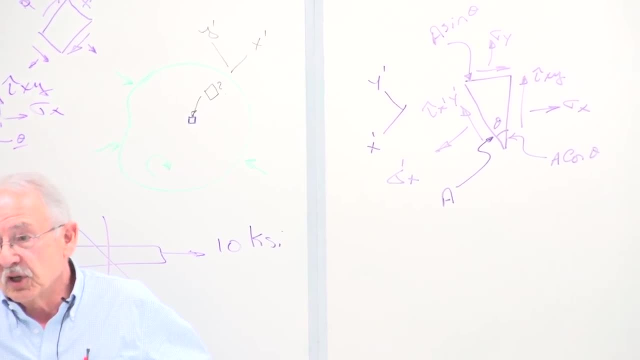 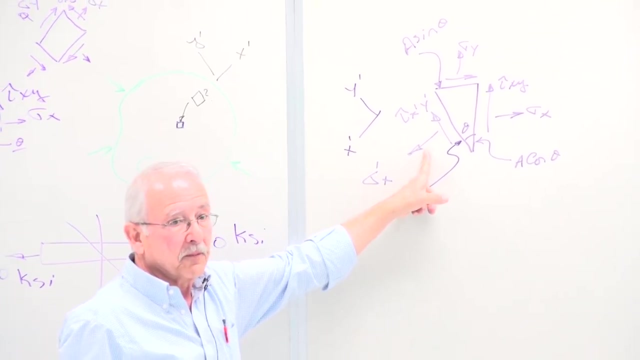 In the summation of forces in the x prime direction, you'll have sigma x prime as the only unknown, and that unknown stress will have no component in that direction. Summation of forces in the y prime direction: We'll only have that as the unknown. 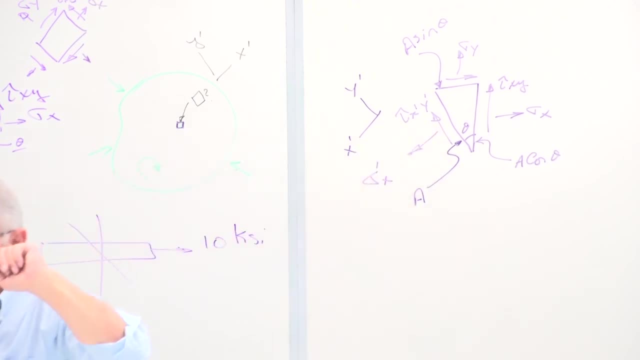 And this will not have a component in that direction. So when you write these equilibrium equations and you square them and add them together and simplify them trigonometrically, what you will find is the equation of a circle. That circle is called Mohr's circle. 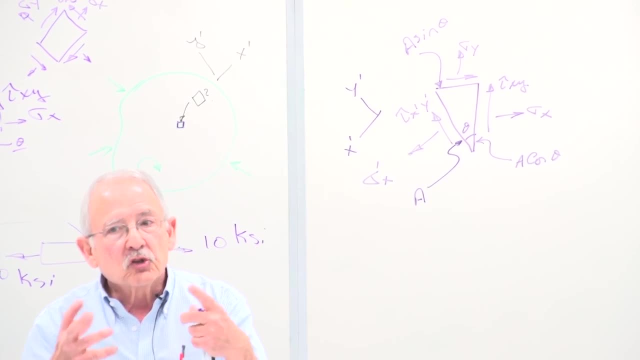 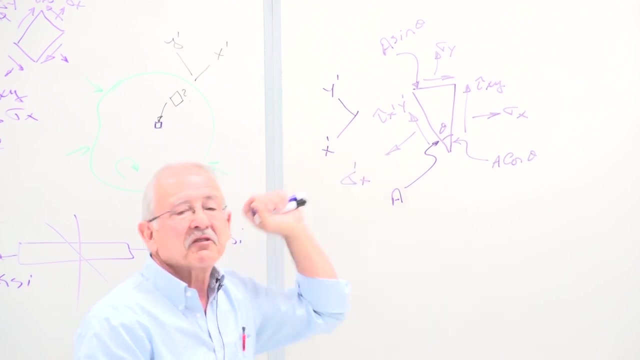 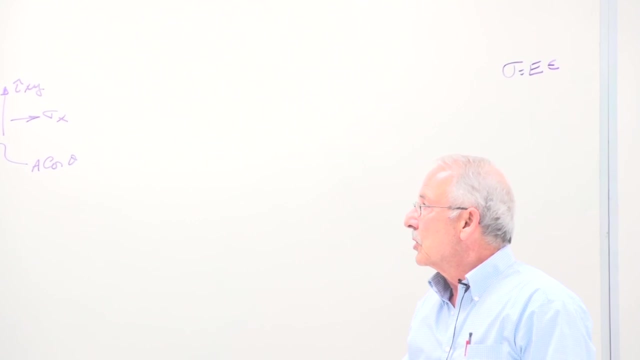 Okay, All that it does. it represents the results of these equations, called transformation equations, graphically and makes their solution of the problems a little bit simpler. Rather than using those equations, we use Mohr's circle. So any questions so far. 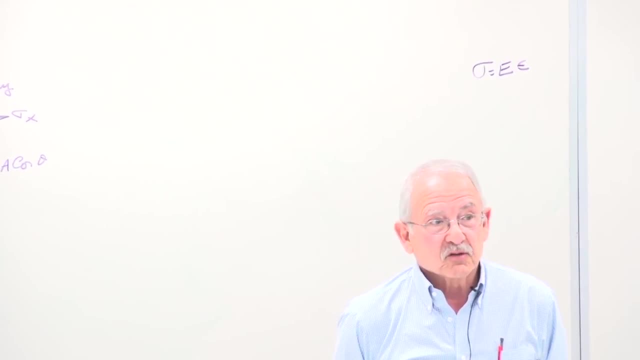 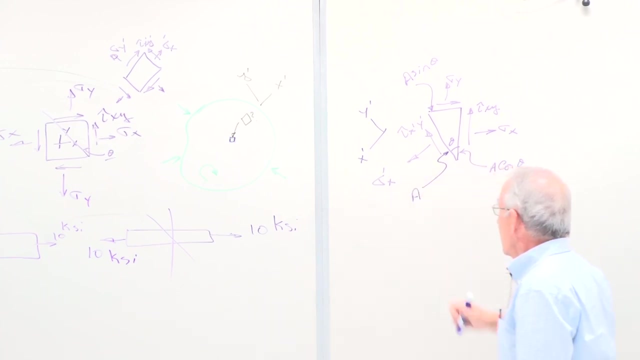 Please do. Please do ask your questions. if you do have them, Don't let them go unanswered. So if we have a set of stresses like that and we want to find these, this is what we do. Take a set of axes, sigma and tau. 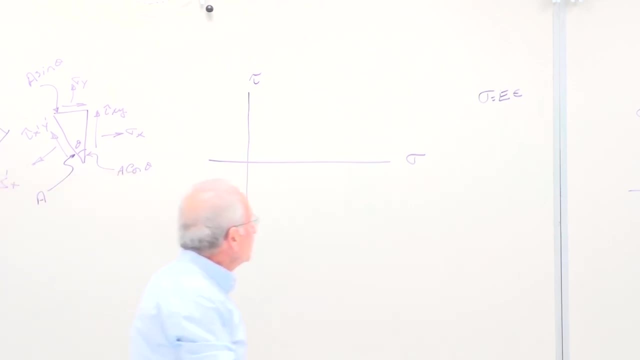 Okay, Okay, Okay, Okay, Okay, Okay Okay. We plot the stresses at this point on the vertical plane and on the horizontal plane. On the vertical plane there's a normal stress- sigma x- and a shear stress- tau xy. Normal stresses are positive if they're tension. 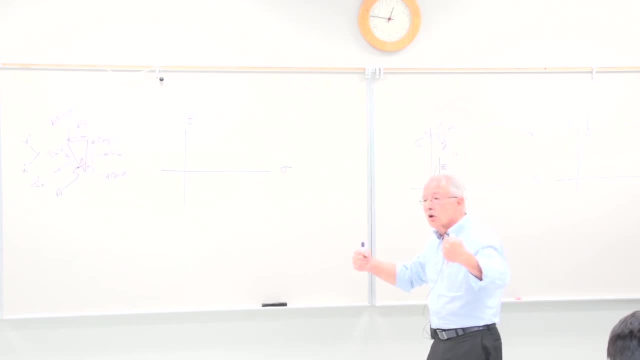 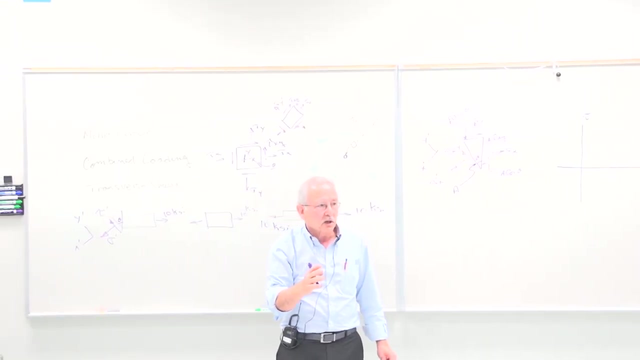 They pull on the material. Okay And negative if they're compression Shear stresses and remember once again, this is all at one point, So there has to be only one shear stress at this point. There can't be very many, two or three, just one shear stress. 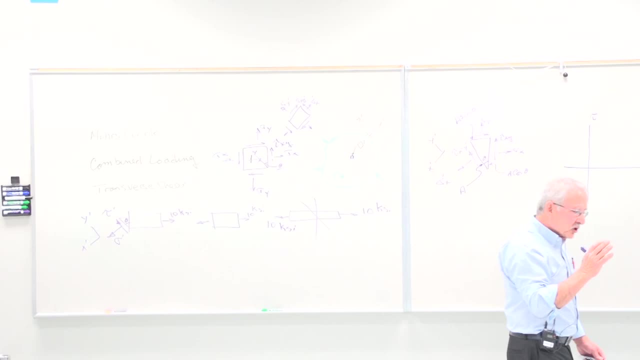 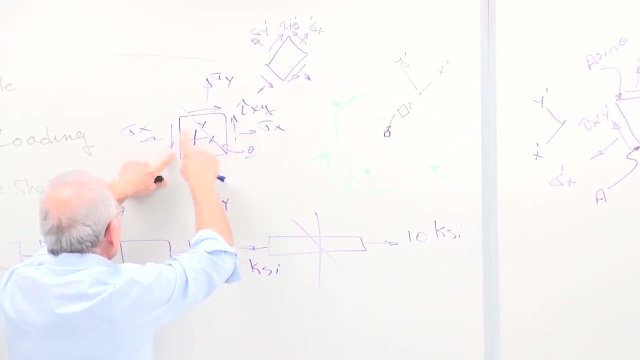 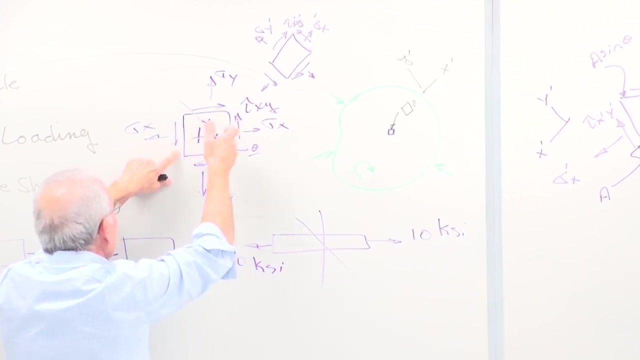 But for the construction of Mohr's circle we have a special convention whereby we think of these two shear stresses as two forces and say: if they produce, these are both on vertical planes. remember, If they produce about the center of this, a counterclockwise moment, then they're negative. 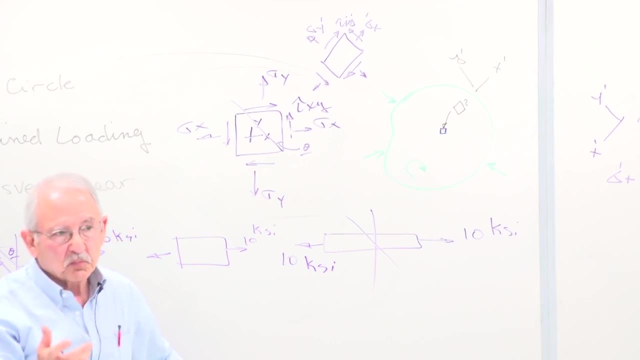 If they produce a clockwise moment, then they're positive. By that convention this is a negative shear stress And that's a positive shear stress. And that really doesn't make sense, Because at one point you should only have one shear stress: positive or negative period. 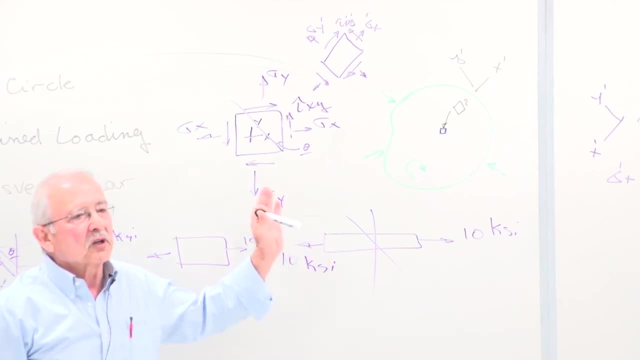 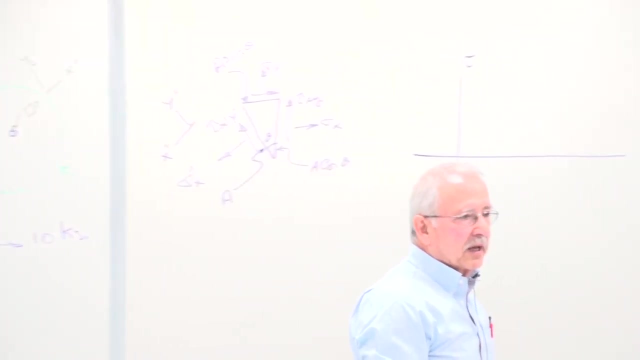 But in order to draw Mohr's circle, we use this convention and it works: The sign of shear stresses as well as normal stresses. I'll talk about that, probably next week sometime. There is a way to find the sign of shearing and normal stress. 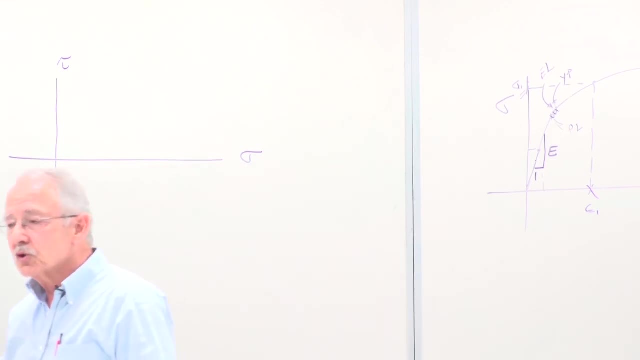 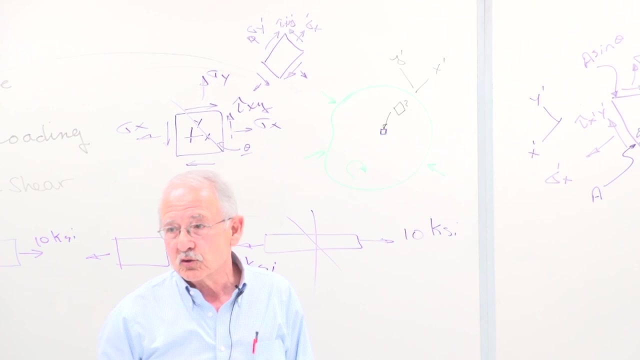 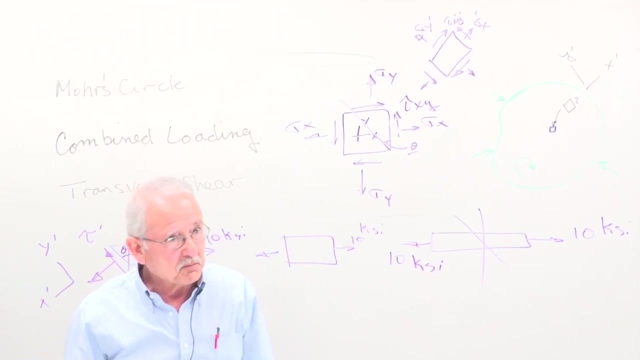 And the way to find the sign of shear stresses is by using the same approach, And you don't have to worry about clockwise and counterclockwise. And if you do use that approach, both of these shearing stresses will be either positive or negative, as the case may be. 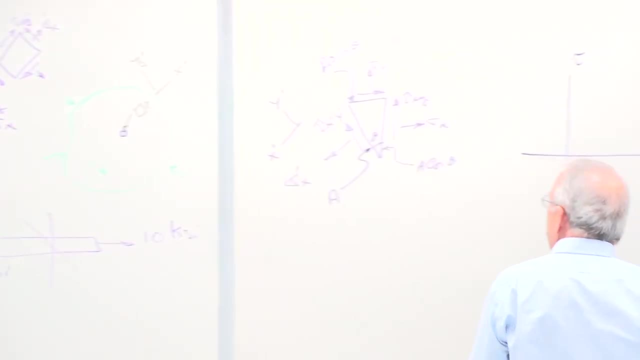 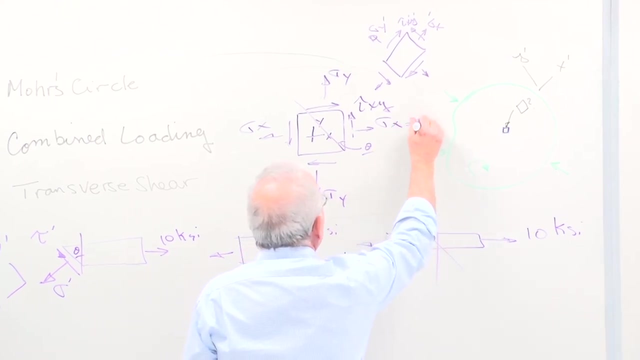 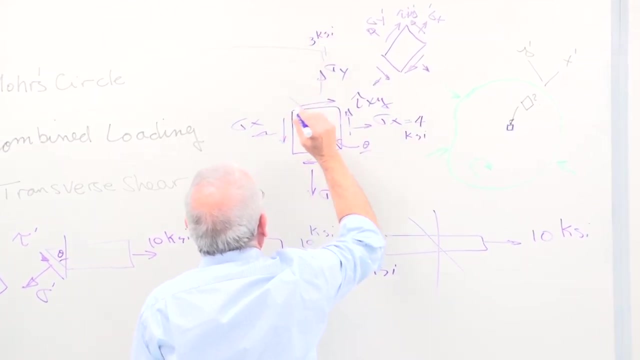 But for Mohr's circle we use this convention. Okay, So let's just give these some numbers. So let's say this is equal to 4 KSI, that's equal to 3 KSI and my shear stress is equal to 2 KSI. 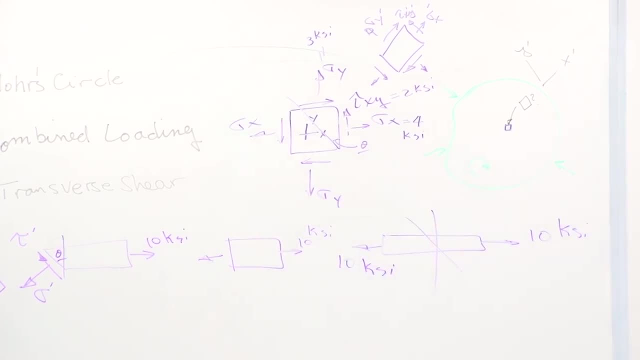 Let me erase the top elements so these will not be so clogged, And this too, Okay. So let's do this. So let's do this, Let's draw Mohr's circle. for that, We'll draw Mohr's circle and take a break. 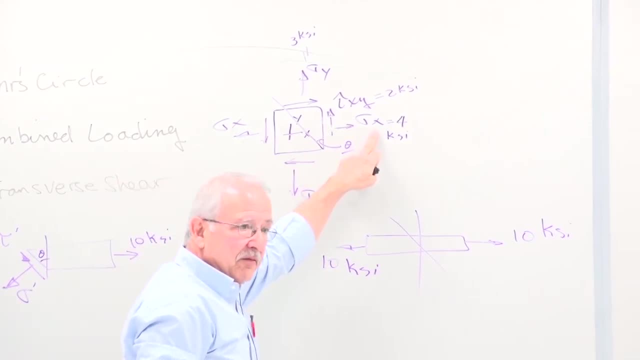 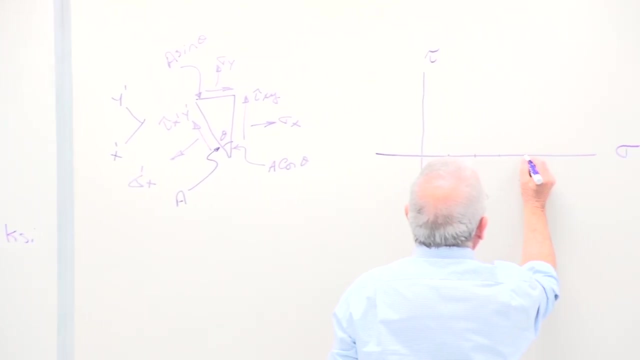 On the vertical plane we have a normal stress of 4 KSI And a shearing stress and according to our convention, it's negative, counterclockwise, Oh sorry, Negative. This point, which is a point on Mohr's circle, represents the stresses on the vertical plane. 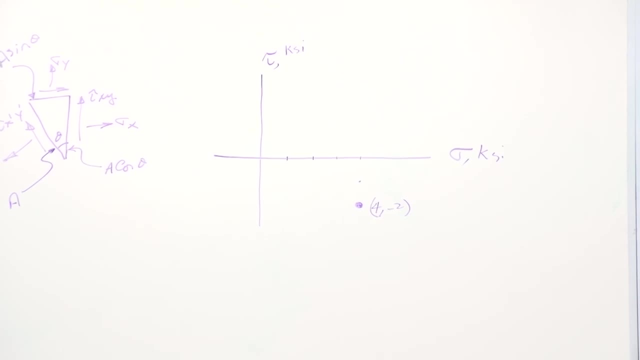 It is sigma x. yes, but sigma x is acting on a vertical plane, on a plane parallel to the y-axis, So we'll call this the vertical plane. Similarly, on the horizontal plane, we have 3 KSI and 2 KSI. 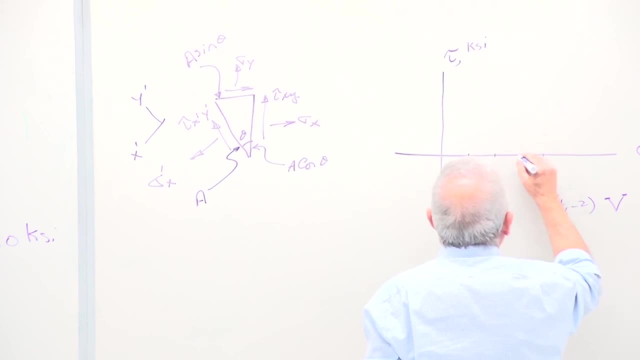 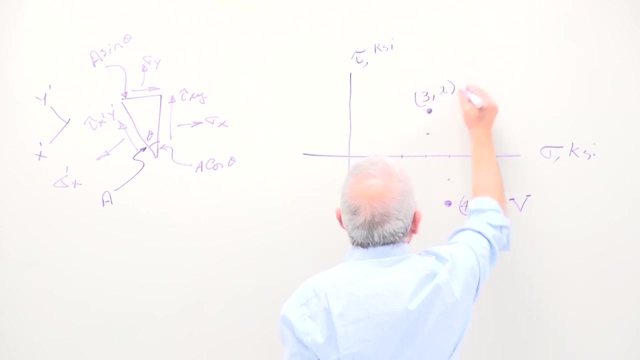 This is going to be tight, but that's okay. So 3 KSI and that time positive 2,. so 1, 2.. 2. Stresses at these points: 3 and 2, they represent the horizontal plane. 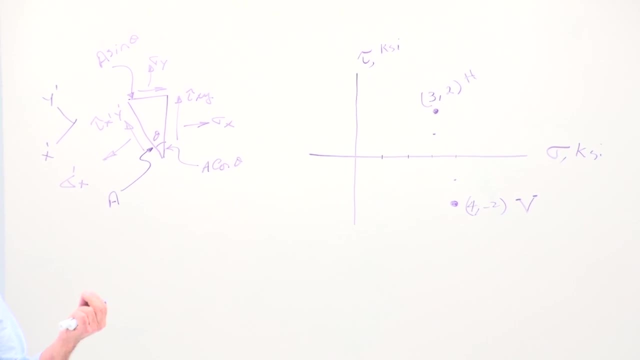 These two points are the endpoints of a diameter of Mohr's circle. So if I connect these two and if I draw a circle like that, that's Mohr's circle, Just like these two points represent the stresses on the horizontal and vertical planes. 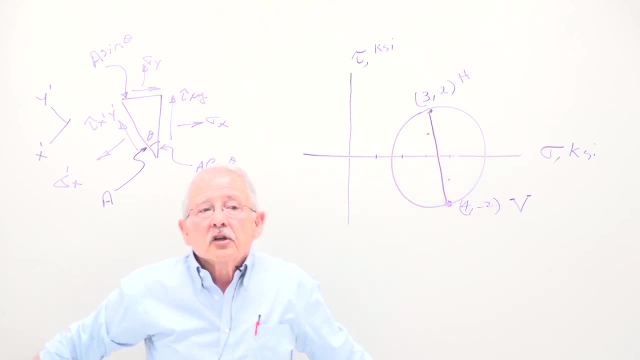 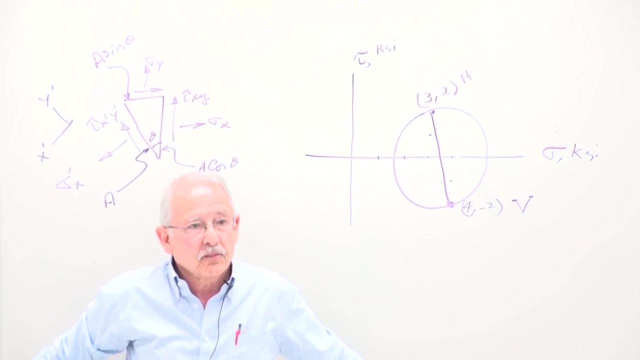 all other points on Mohr's circle represent the stresses on all other planes passing through that point And therefore, if we know the orientation of those arbitrary planes, we can find the stresses on them by using Mohr's circle. Now let me do the maximum and minimum here, and then we'll take a break. 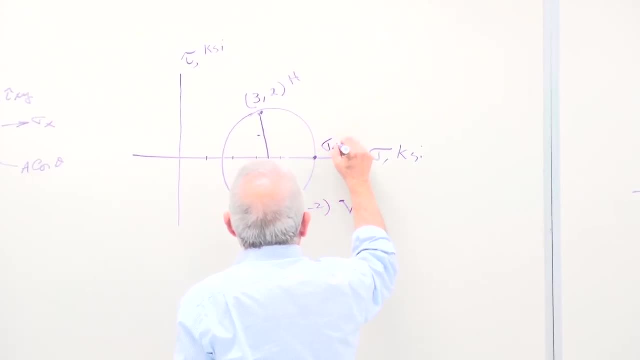 Thank you. You can see that if I calculate the radius of Mohr's circle- and it's not very difficult to calculate- it's the hypotenuse of this little right triangle, The distance from the center of Mohr's circle to the tau axis. 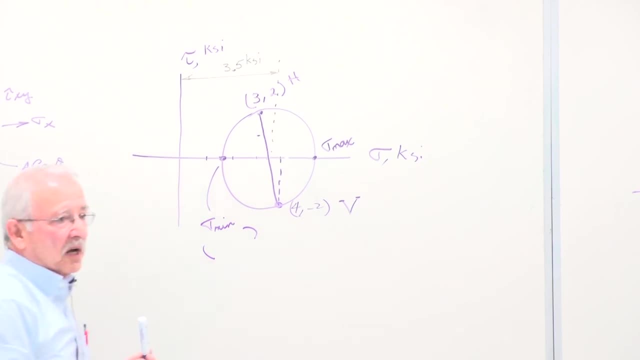 is 3.5 KSI The max stresses. those are for this plane. correct, Correct, I'll get to that. I'll get to that. Are we going to learn a plane stress, plane strain later, or this is part of it? 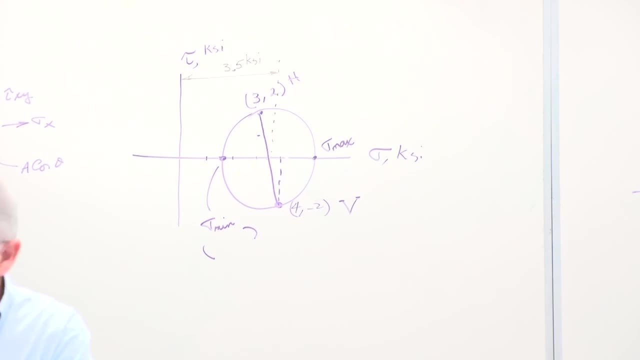 This is plane stress, Or I mean a three-dimensional. You mean three-dimensional? Yes, I'll talk about that. today, I'll extend this Mohr's circle to three dimensions. That's why I have parentheses here. These parentheses are for in-plane. 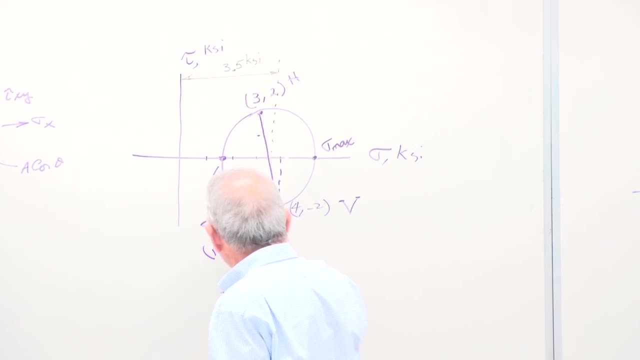 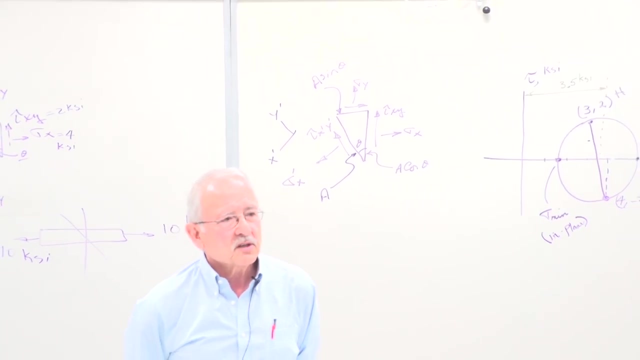 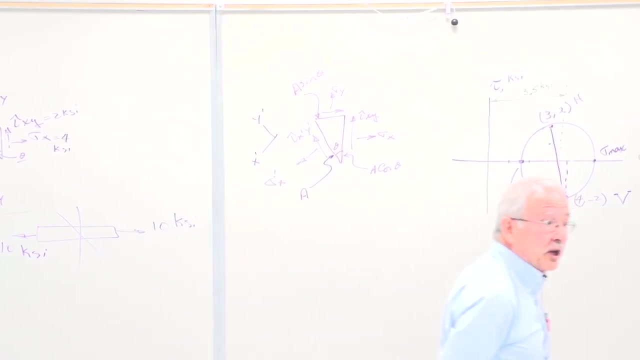 Now that you asked the question, we'll put them in. We have stresses on other planes as well. The sigma max and sigma min are called principal stresses. So what is the definition of principal stress? We have no shear stress. They act on planes of no shear. 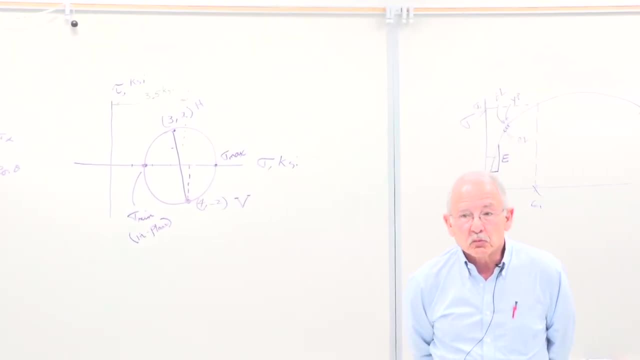 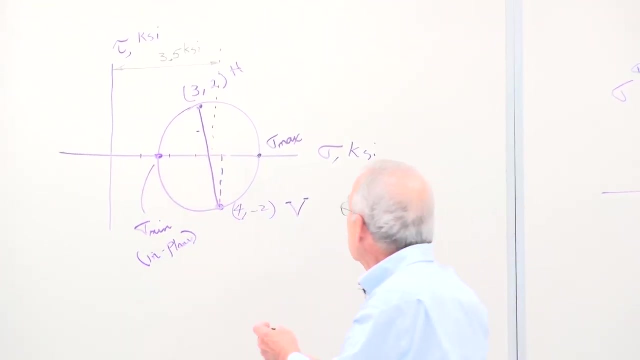 Not that they should be either maximum or minimum, Although that's partially true. Maximum and minimum stresses are included in the principal stresses Because, as you can see, the shear stress here is zero. The shear stress there is also zero, But look at this three-dimensionally. 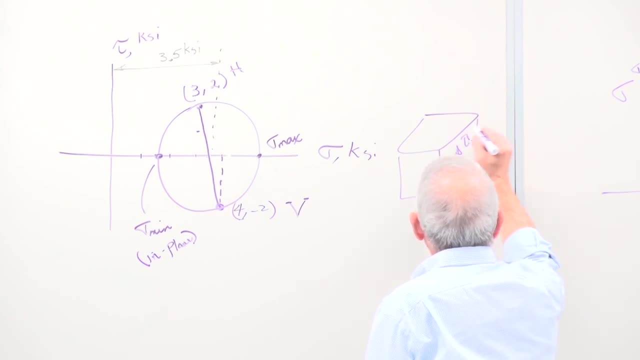 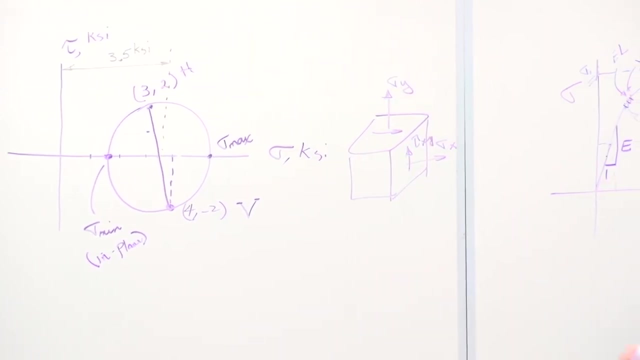 This is our sigma x, tau xy and sigma y. Right, What's the shear stress on this plane, The plane that I have put a circle in At that point? This is one point. Remember this. This whole cube is one point. 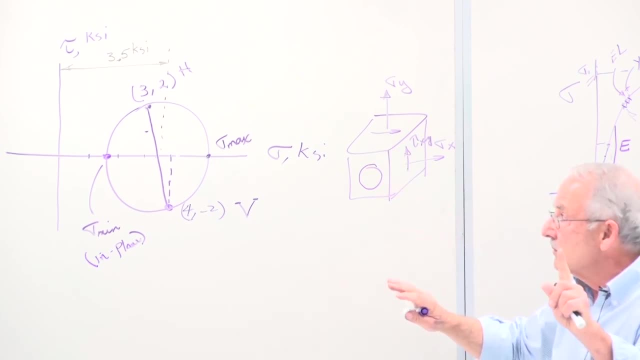 Oh, I thought you meant at the angle of the principal stress. No, I'm not looking at the angle of the principal, Not yet anyway, Not looking at that. What I'm looking at are the principal stresses, the shear stresses themselves. 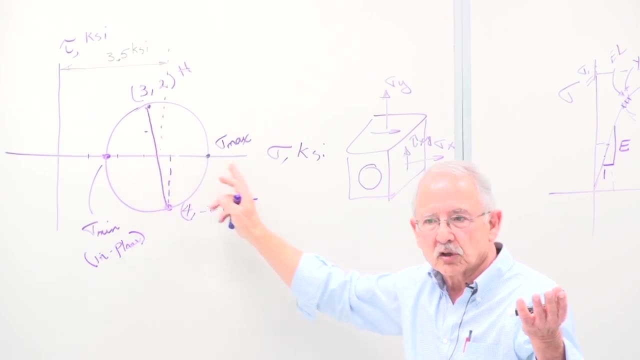 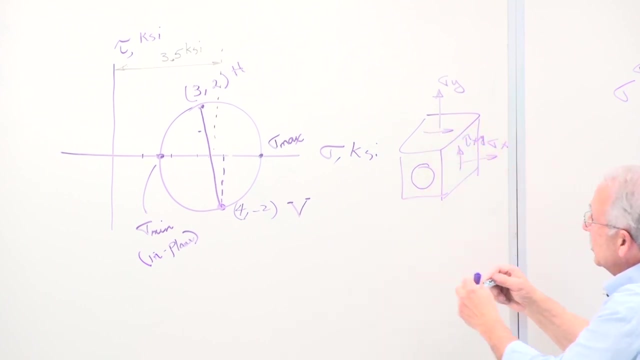 What are they? They're stresses that occur on planes of zero shear, Correct, Okay? Then my question to you is- and they're oriented at some angle here, So if I were to draw them on this, I won't draw them right on it. 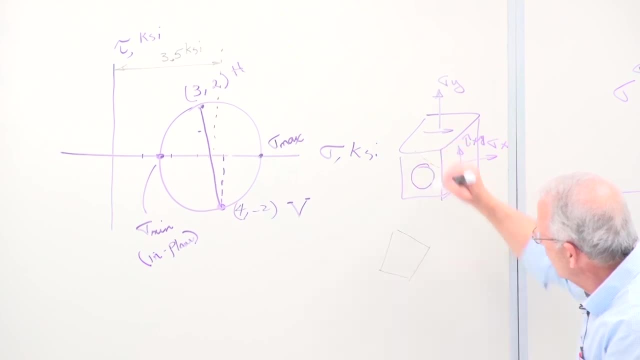 but probably they would look like that. This on top of that, See, like so. Those would be the planes on which the principal stresses will act. But this is that This is four, that's two, that's three, and so on. 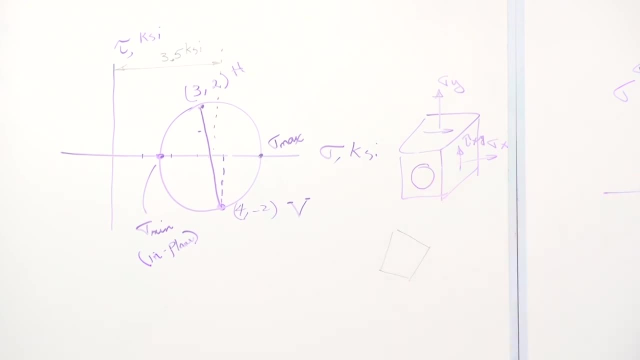 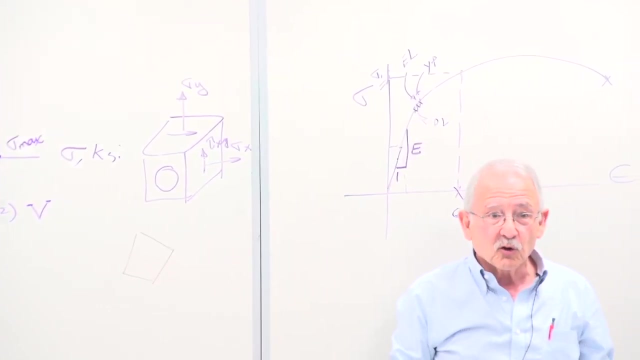 What's the shear stress on this plane? Zero, Zero. You don't see any loads. What's the normal stress at that point On that plane? Also zero, Also zero. You don't see any normal loads either. You don't see any loads perpendicular to that plane. 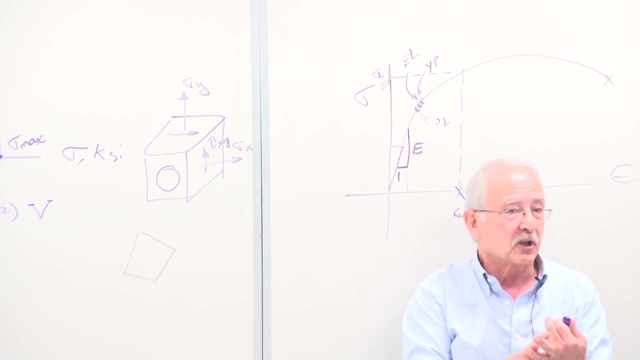 You don't see any loads parallel to that plane. You don't see any loads parallel to that plane. There is no normal stress on that plane. There is no shear stress on that plane. Therefore, zero is a principal stress Because it acts on a plane of no shear. 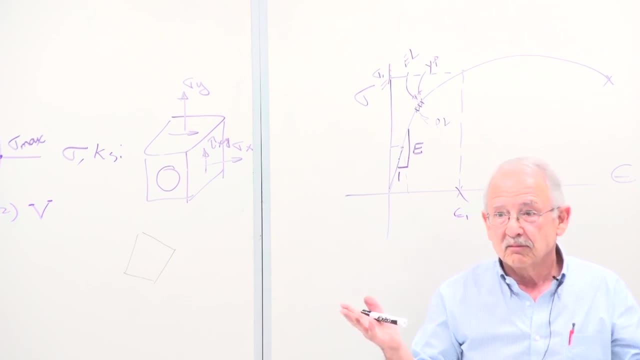 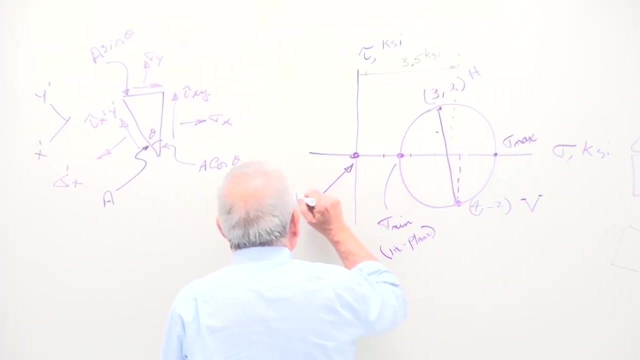 Because it acts on a plane of no shear. Because it acts on a plane of no shear, So coming back here, So coming back here, That is our real minimum principal stress, Not that. And if you take a look at this cube, 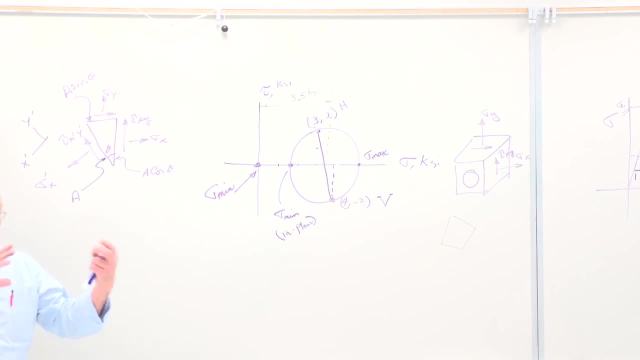 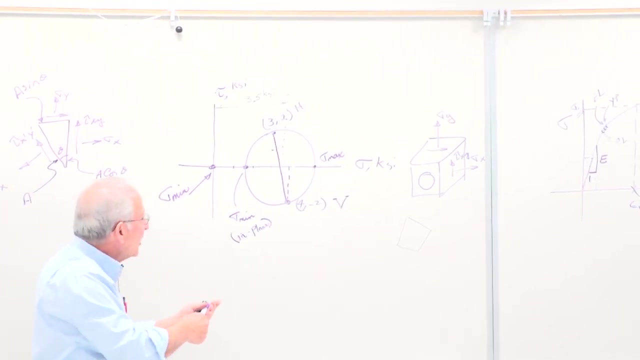 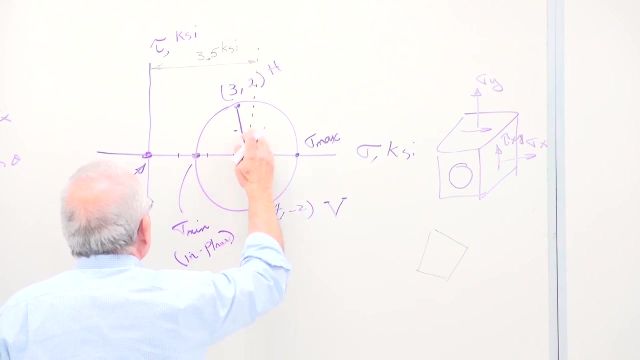 And if you take a look at this cube, And if you take a look at this cube, this element, this three-dimensional element from the three sides, from the three sides, for each side, you get a more circle. Before I draw those, 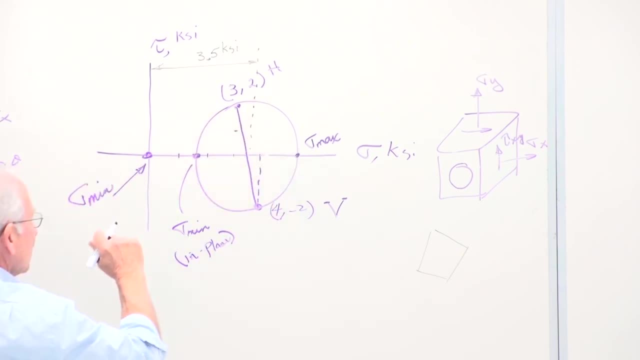 Before I draw those, one more thing: The maximum shear stress. I will write the values for these after we come back from this, after we come back from this, But the maximum shear stress is that, isn't it? That's the maximum shear stress. 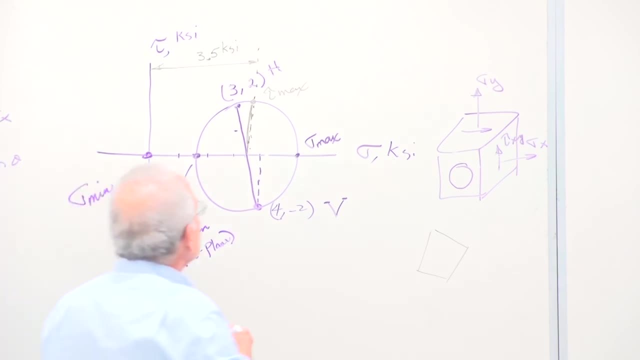 In plane shear stress. So if I have these principal stresses, I will have the ends of more circles. These two have given me one, These two will give me another one, And these two will give me another one, And the radius of that. 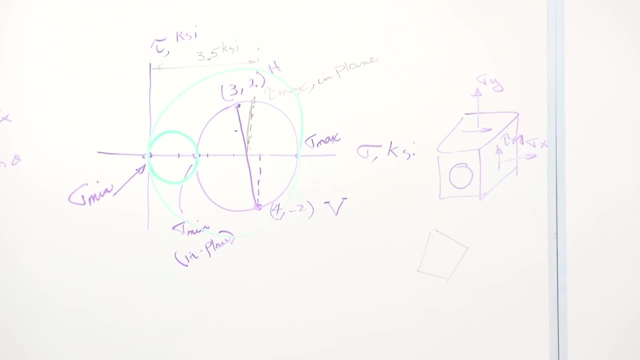 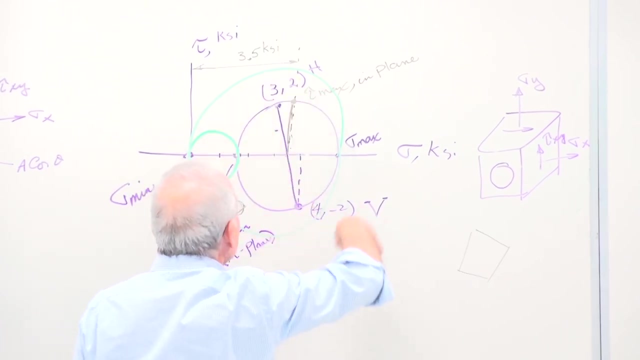 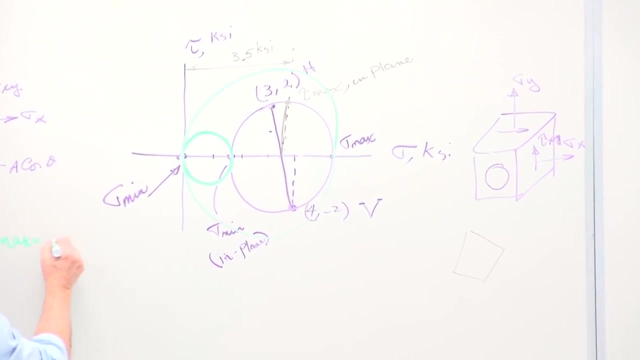 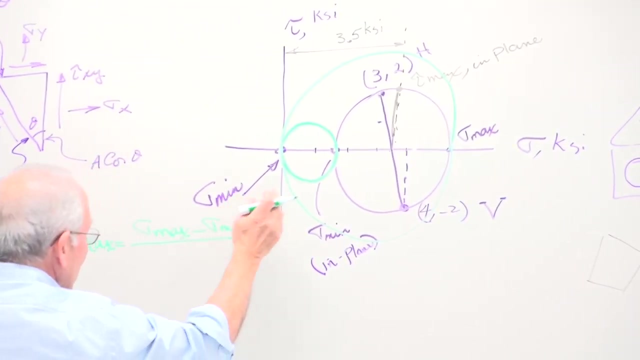 large green circle is the real maximum shear stress, not the in plane one. So tau max is the radius of this big circle. Tau max therefore is sigma max minus sigma min, not in plane, just sigma min. sigma max minus sigma min. 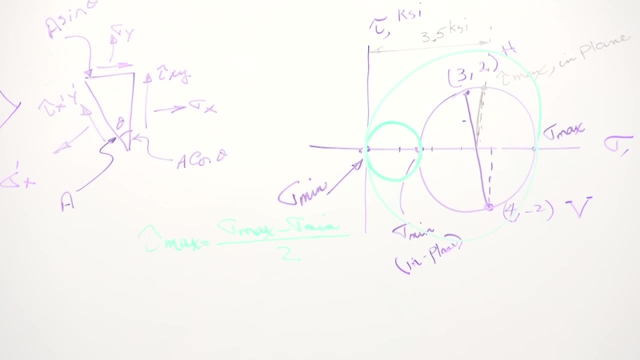 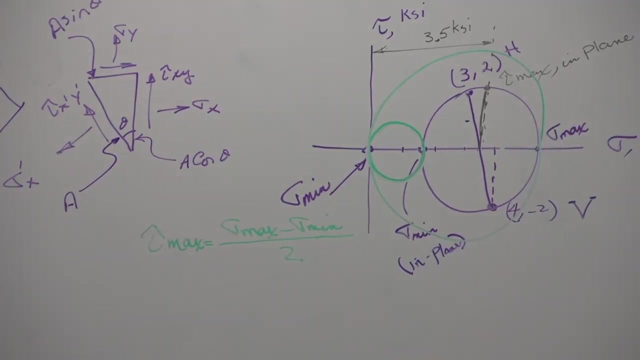 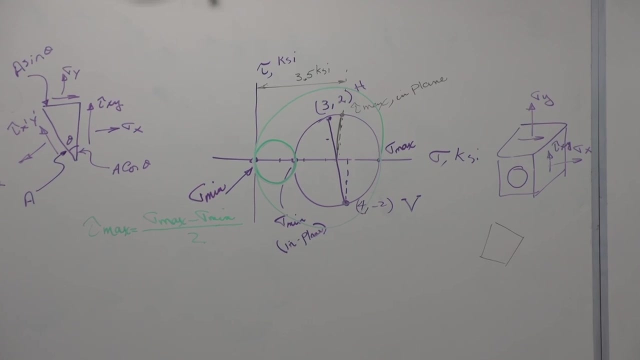 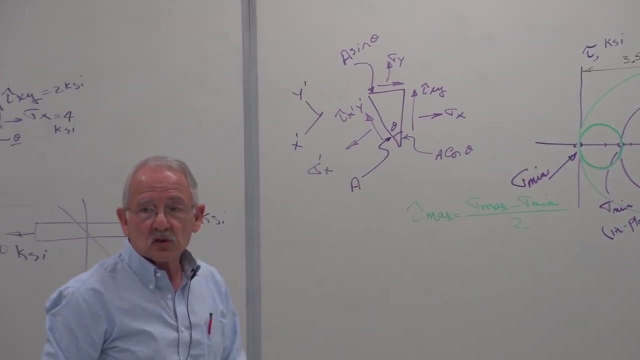 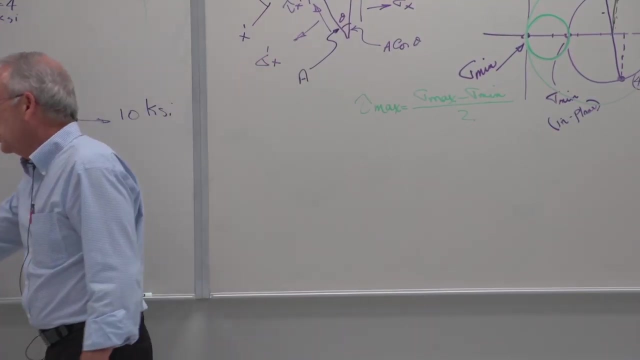 divided by two, The radius of the largest Mohr's circle. Okay, any questions? Okay, let's take a break. Ooh, way past the time. Now, any questions so far. The location of the principal stress, meaning the angle. 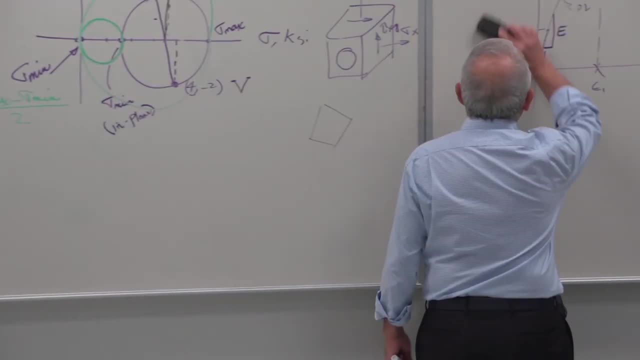 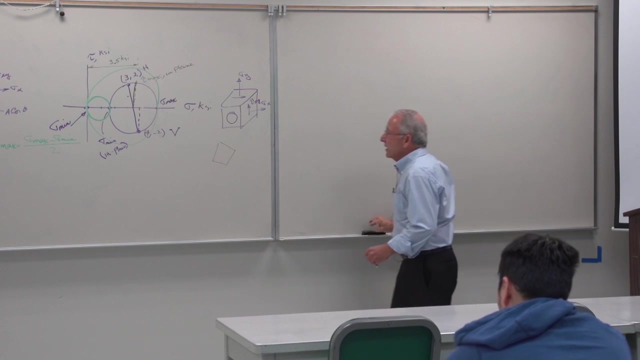 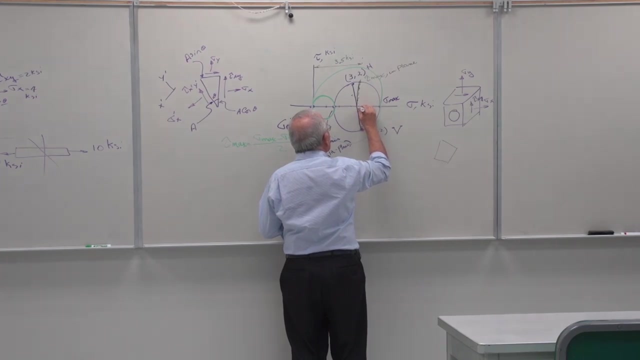 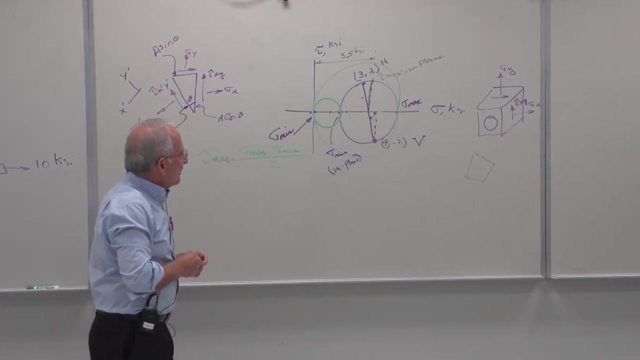 at which the plane of the principal stress acts can be found. if we find either of these two angles, either this one or that one, Of course they're both exactly the same. So how does that tell us what the principal stress is? 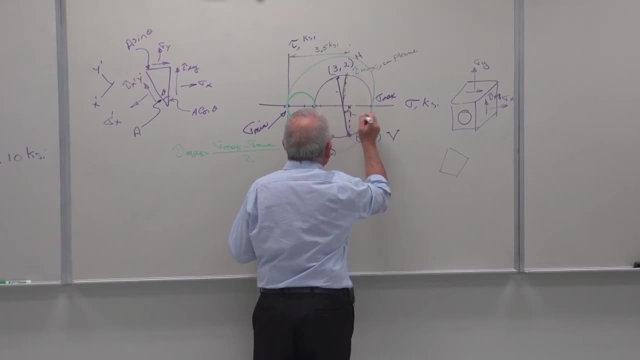 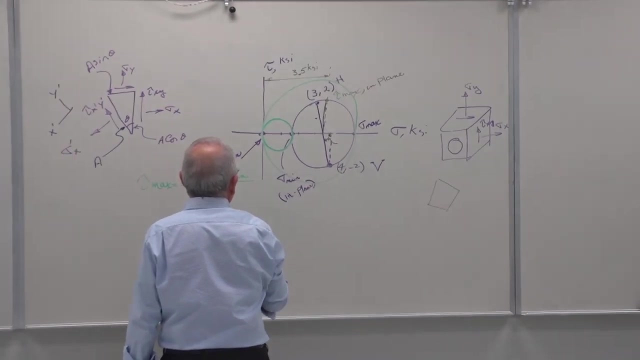 Let's assume- and I'm not going to go through finding that angle- it's simple enough- in the right triangle you can do that. Let's say that angle is- I don't want to call it theta, because I called that one theta- 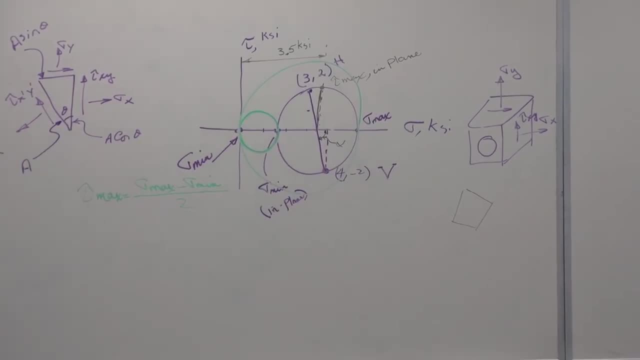 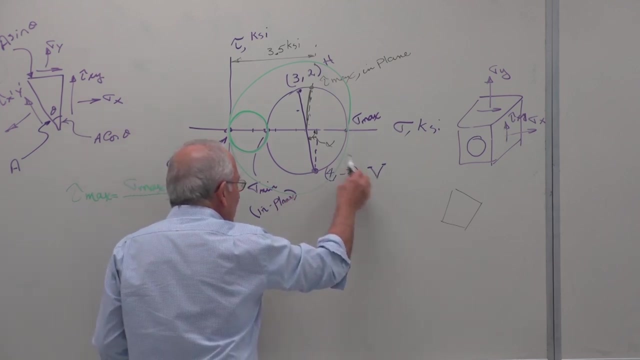 let's call it alpha. Then this point representing the vertical plane, or this radius representing the vertical plane, stresses, if it is rotated through this angle. call it two alpha. you recall that the angles on the element are doubled on the Mohr's circle. 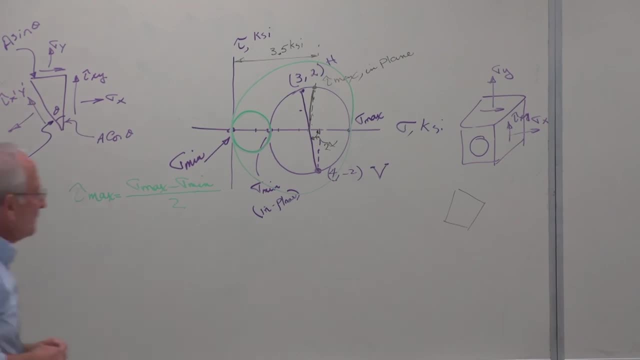 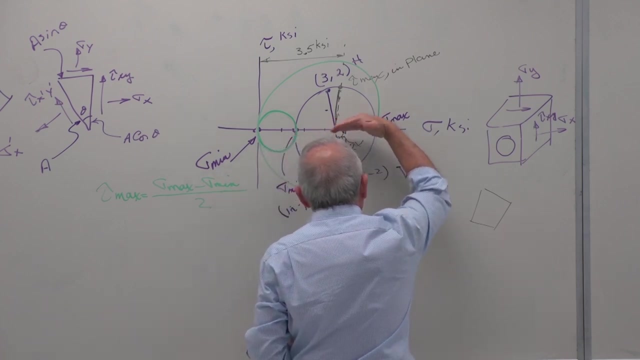 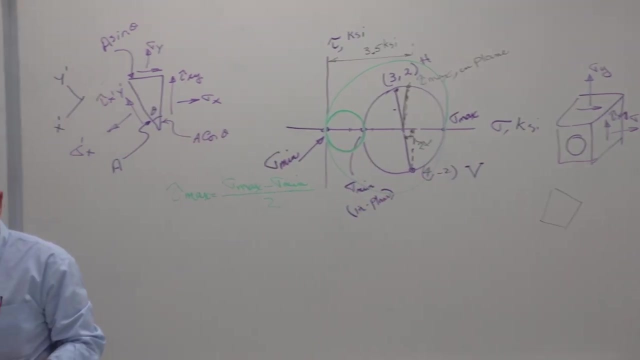 Therefore I'm calling that two alpha. If I rotate the vertical plane radius counterclockwise two alpha, I will get to the plane on which the maximum principal stress acts. So if I am to draw that here and notice that I took the 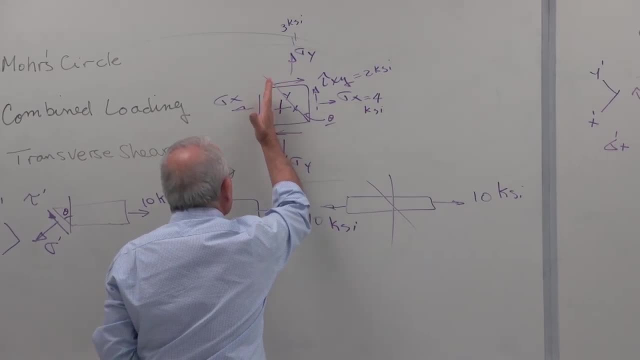 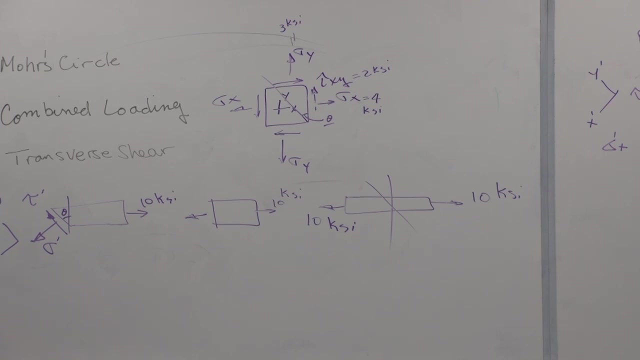 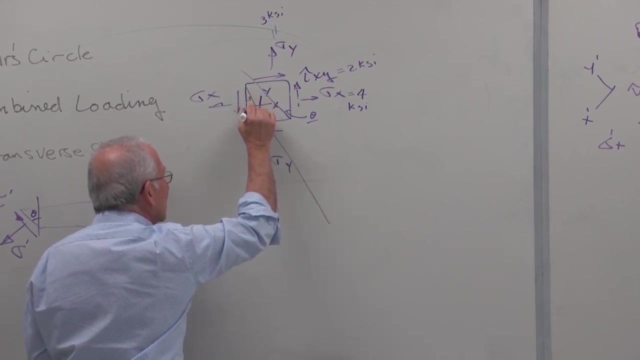 vertical plane- counterclockwise two alpha. Take the vertical plane- counterclockwise alpha. Counterclockwise alpha means like this: This is the plane on which the maximum principal stress acts. Notice that the maximum principal stress acts on the vertical plane. 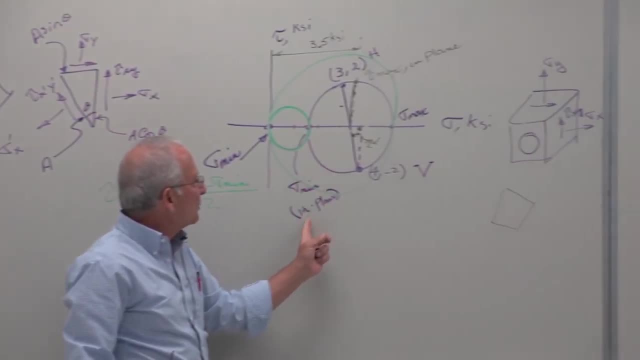 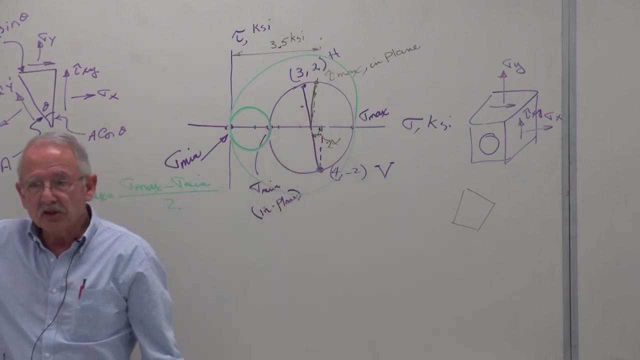 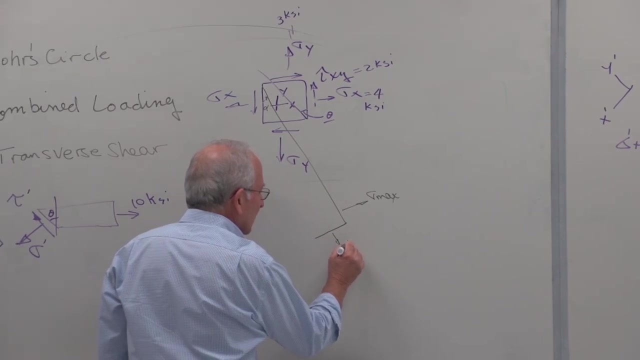 Principle stress and the minimum in plane principal stress are 180 degrees apart in the Mohr's circle. Therefore, they will be 90 degrees apart in the actual element. In other words, if you were to draw an element, it would look like that. 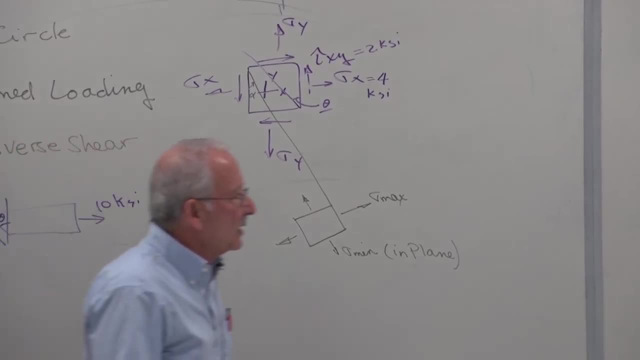 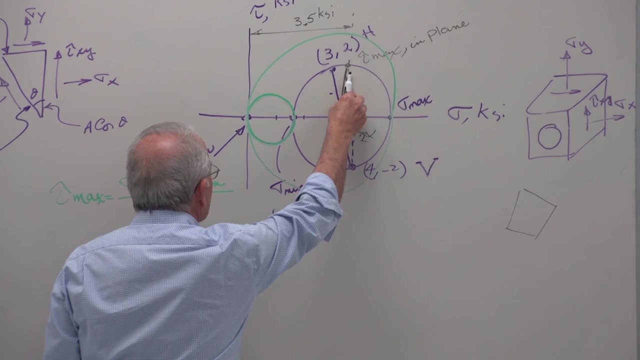 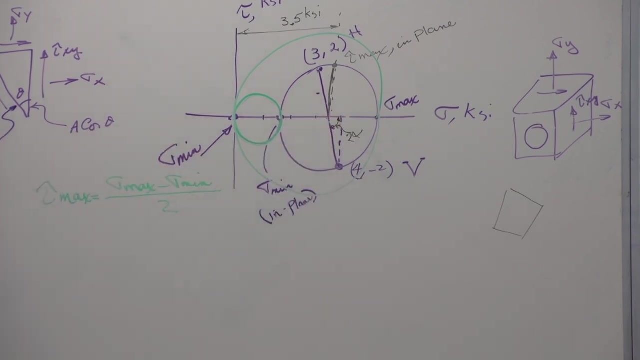 Sometimes they include the maximum shear stress in this sketch as well, because the maximum shear stress is located 90 degrees from either one of these. That's the in plane maximum shear stress, 90 degrees from each one of these, so 45 degrees. 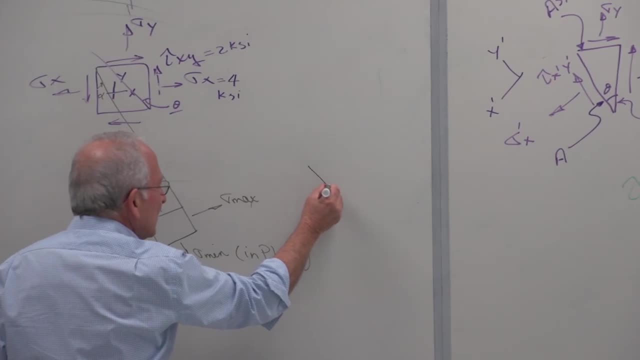 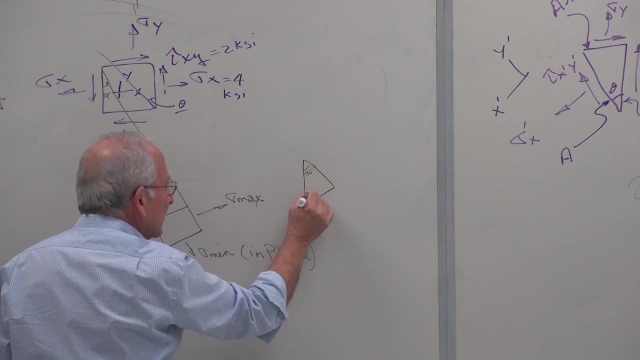 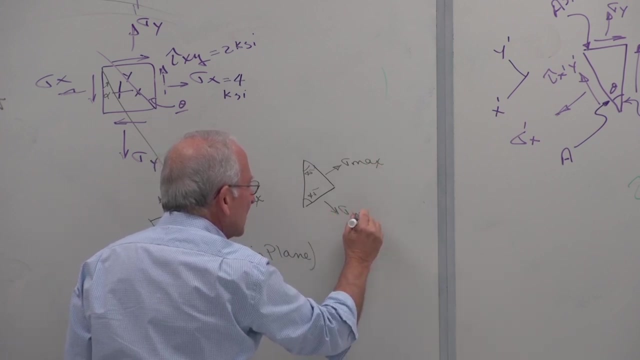 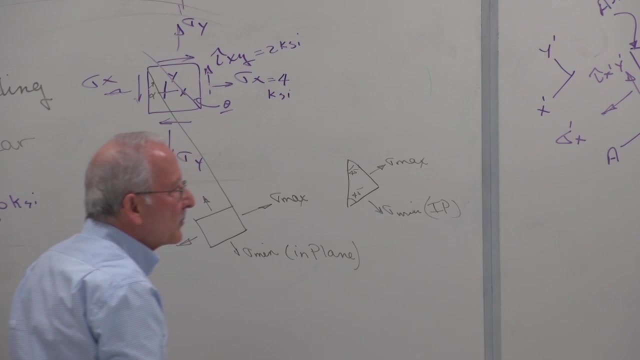 So if I want the maximum shear stress to be shown here as well, 45,, 45,, 45, sigma max, sigma max, sigma min, sigma min in plane and the maximum shear stress, So the maximum. 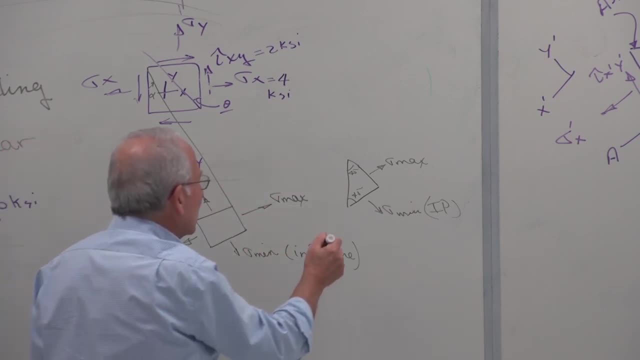 shear stress depends on whether you rotate clockwise or counterclockwise. You can come up with the direction and there's a normal stress which acts on that plane of maximum shear stress. whose value is this? In our case, three and a half. 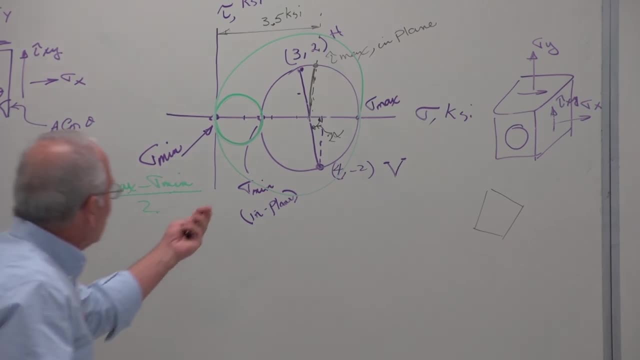 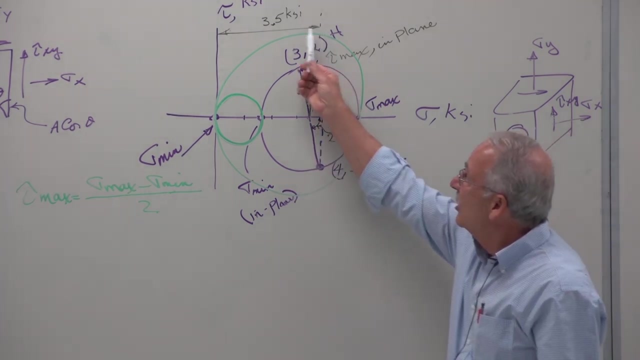 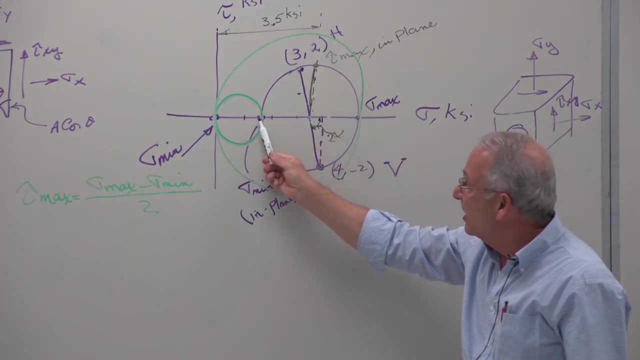 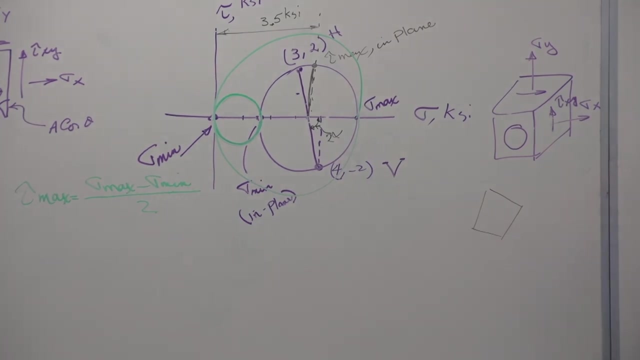 The magnitude of the principal stresses can be found again by looking at that. in plane Mohr's circle, For example, sigma max is three and a half plus a radius. Sigma min is three and a half minus a radius. So sigma max, 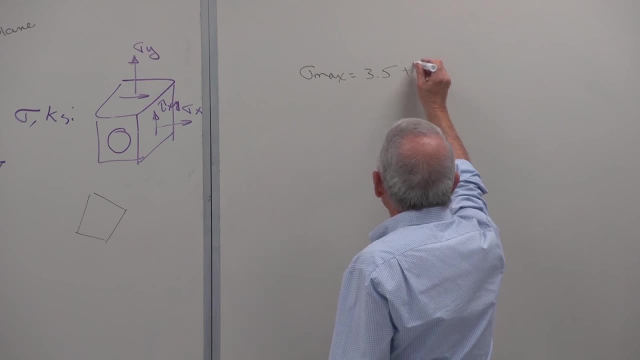 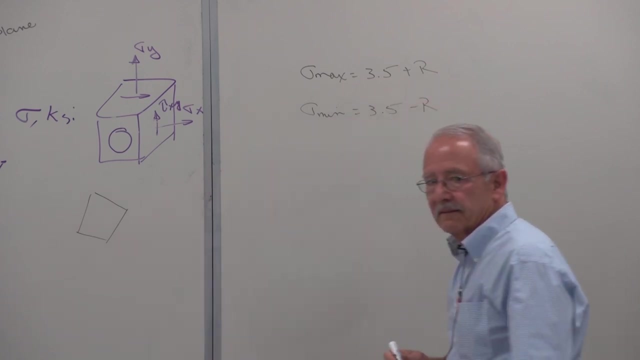 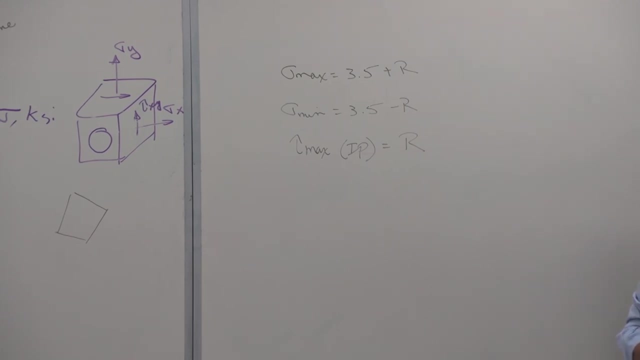 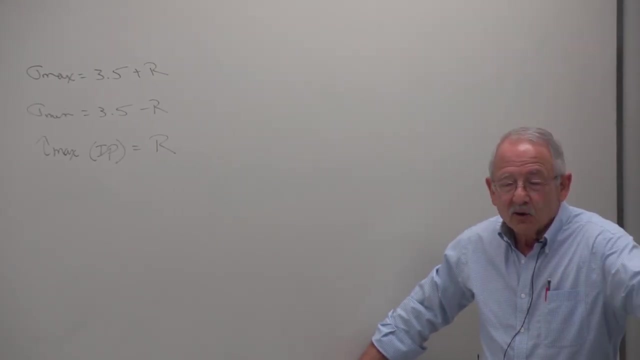 in our case. and of course, the maximum in plane shear stress is just equal to the radius. Okay, Any questions. Whoever asked for Mohr's circle? I forgot. Have I answered all of the questions, or at least the vast majority that there may have been? 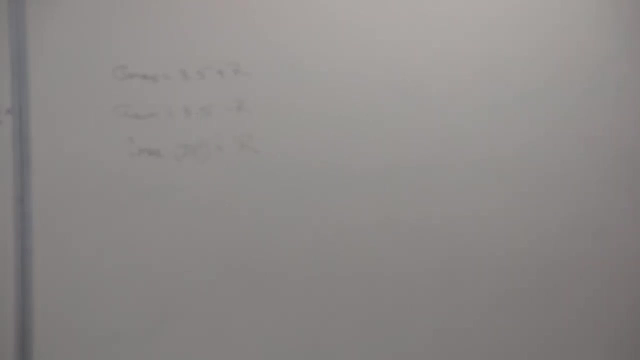 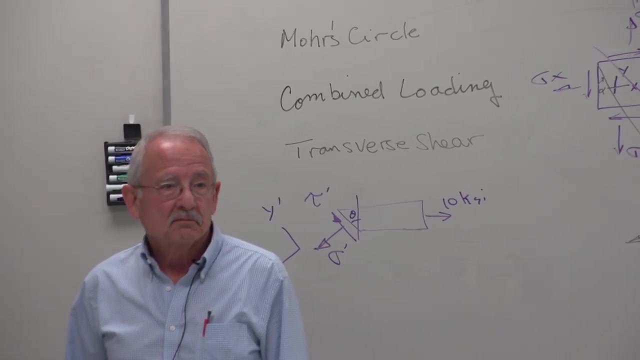 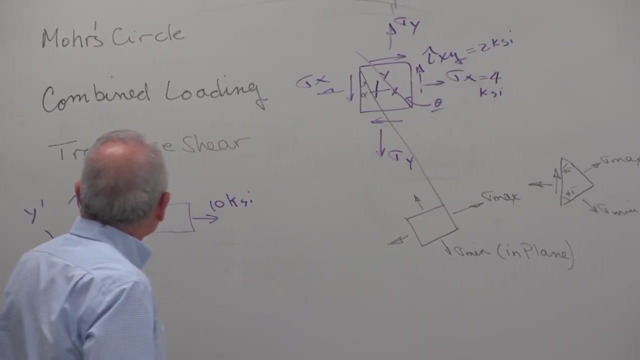 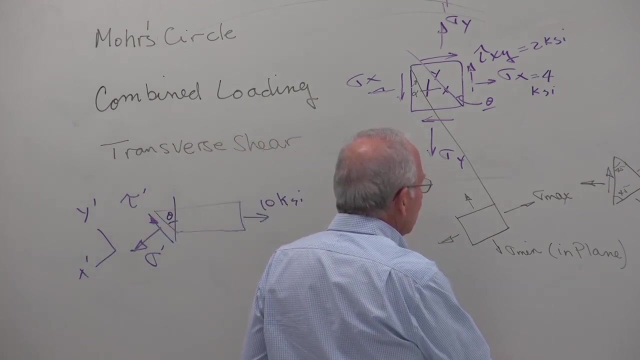 If not, if there's something regarding Mohr's circle that is still not clear, tell me. Nothing comes to mind, huh? If it comes to mind later, ask later. Not a big deal. Next subject: combined loading. Whoever asked this question? do you have anything? 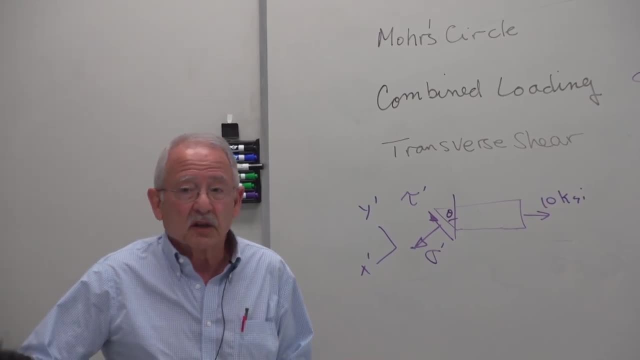 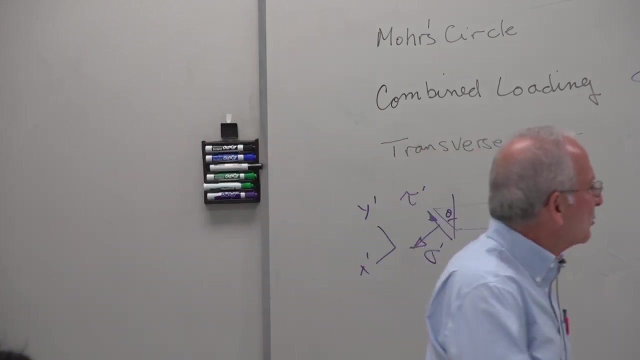 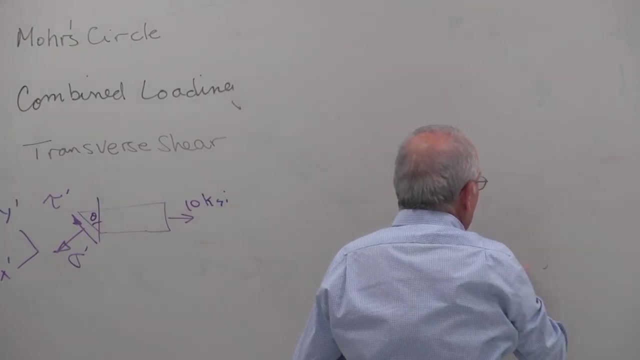 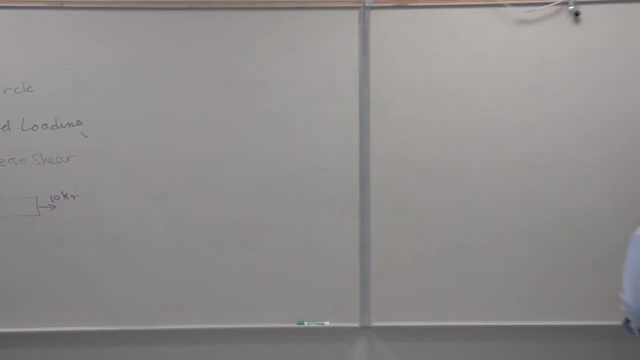 in particular in mind A problem, for example, in combined loading. Who asked the question You did? Do you have anything in mind? Nothing in mind? Okay, No big deal. Let me then give you a problem. We did this in the 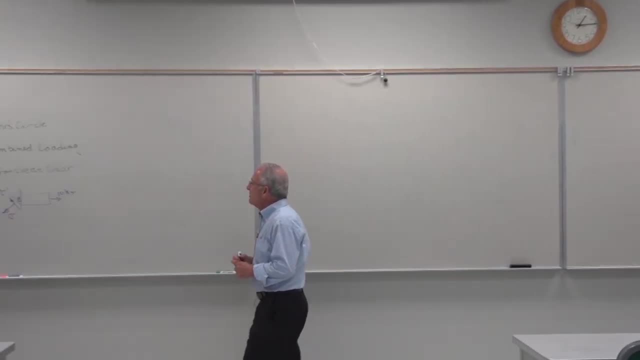 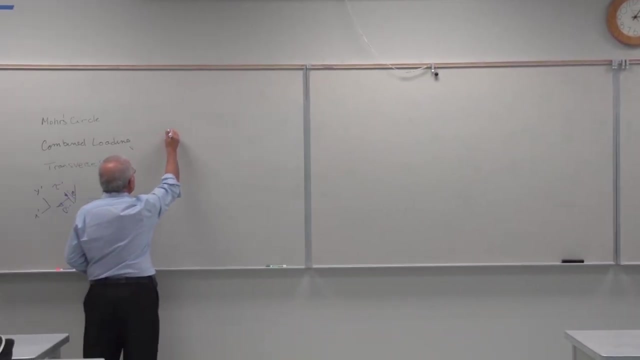 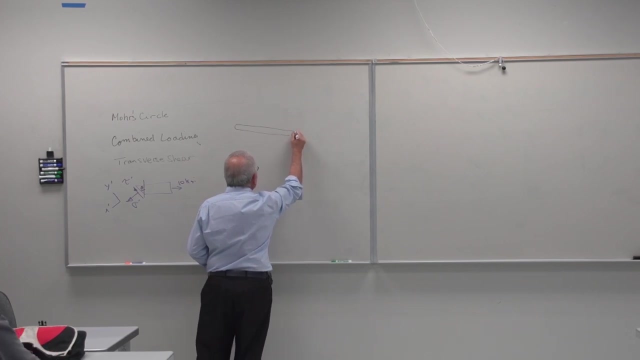 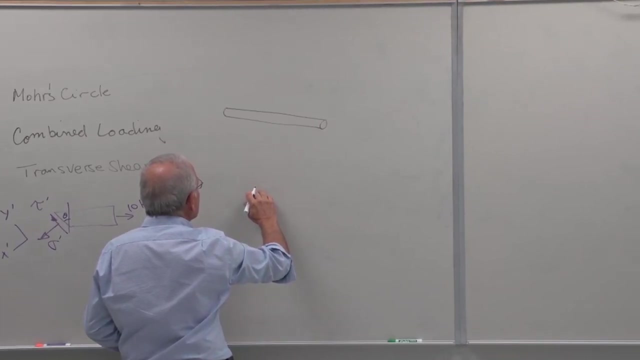 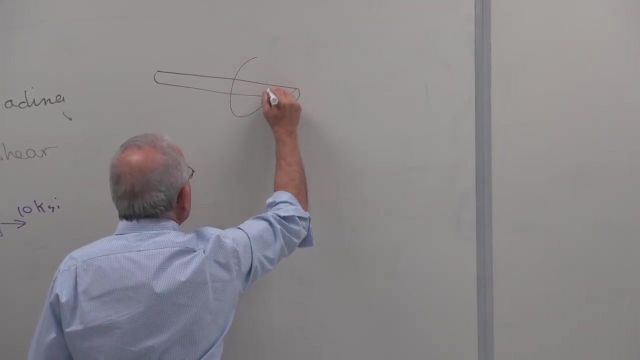 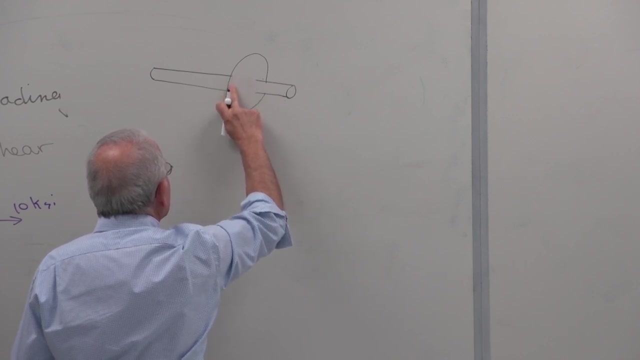 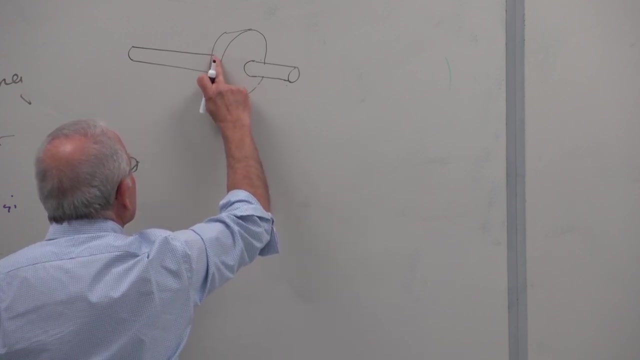 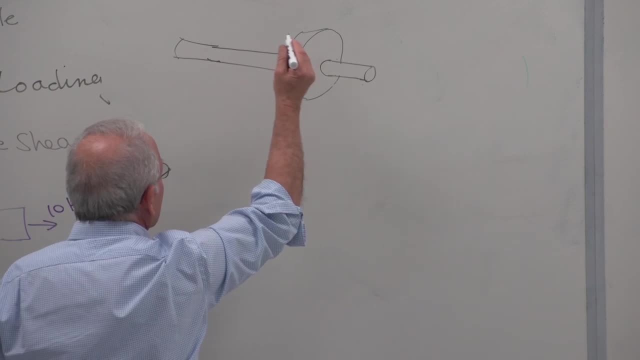 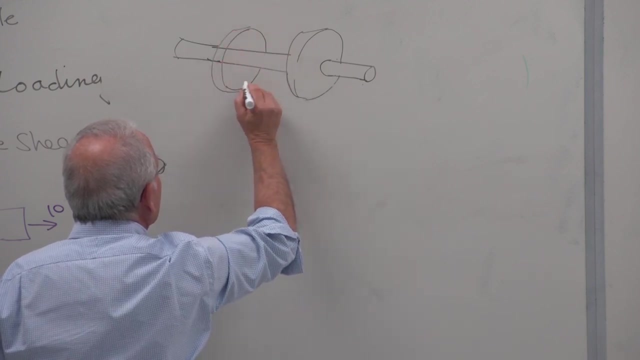 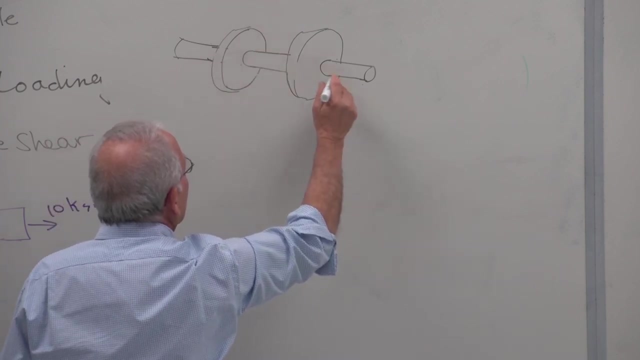 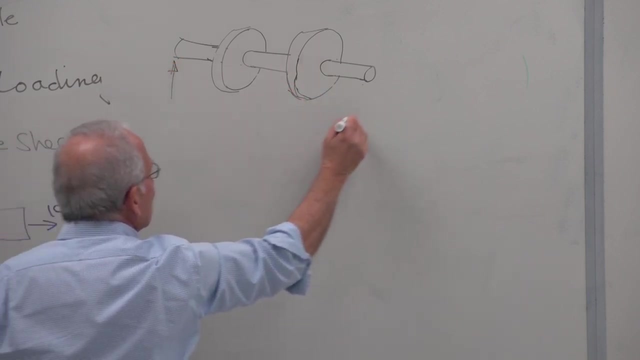 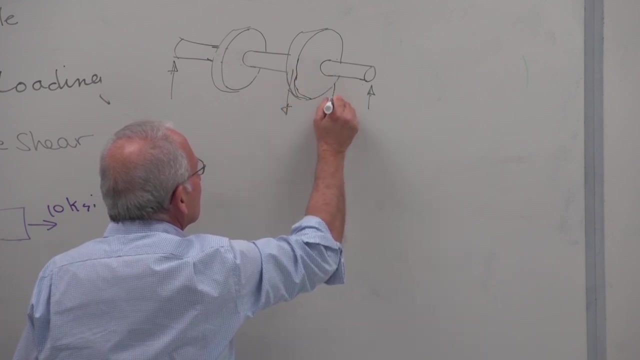 Will you tell me what's the problem that I have to deal with? You know, do you have anything in mind? that is not the best in the world, for sure, But starting next time, Okay, let's say it's simply supported here and here and you have loads on the two sides. 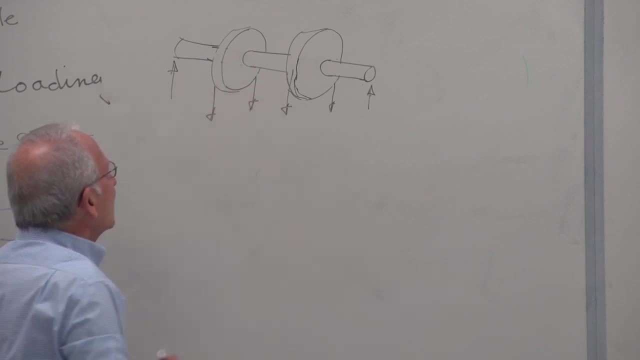 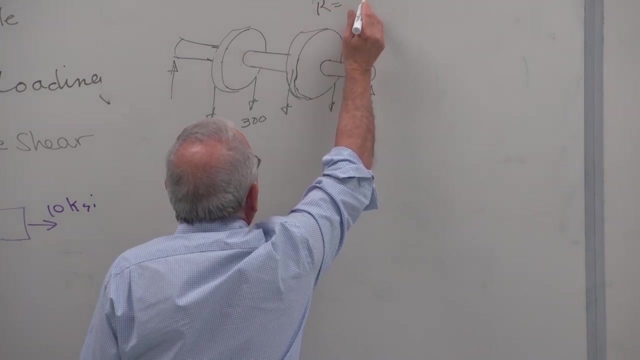 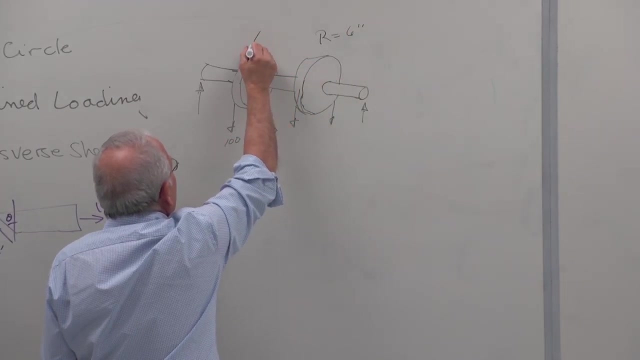 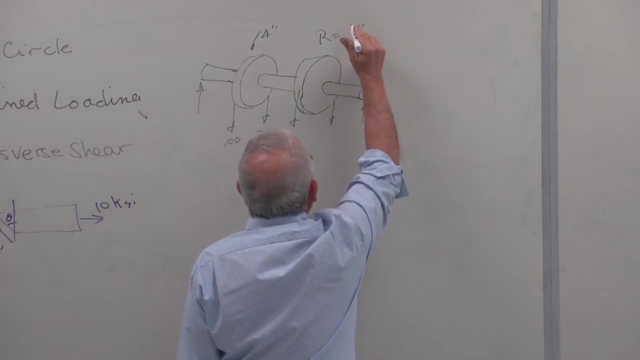 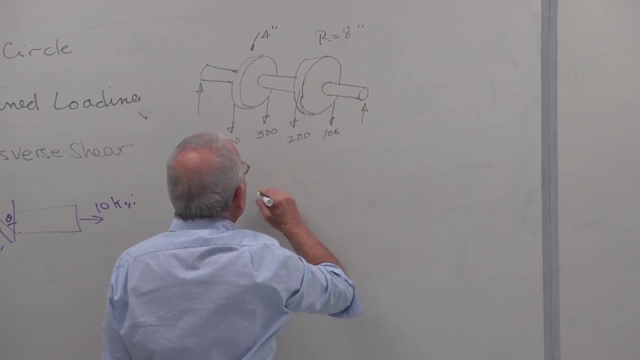 of these pulleys. just give them some numbers. let's say, and let us assume that the radius of this pulley is equal to 6 inches, Okay, And the radius of that pulley equals 4 inches. So that's 200 times 4 is 800, let's make it 8 here so that I can do this. 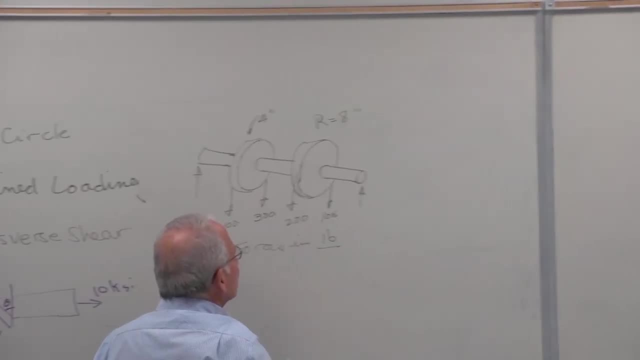 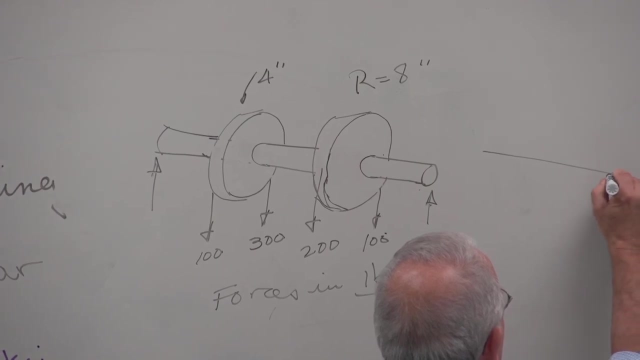 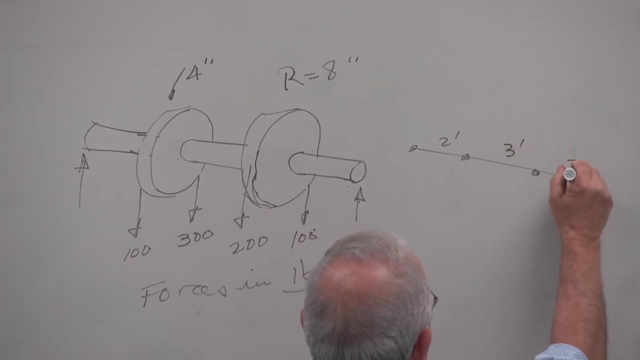 Forces in pounds. Okay, And distances. I'll put them in here like this: 2 feet, 3 feet, 2 feet, just to have taken some number. Is that clear? Especially the last part where I'm showing the length along the member. 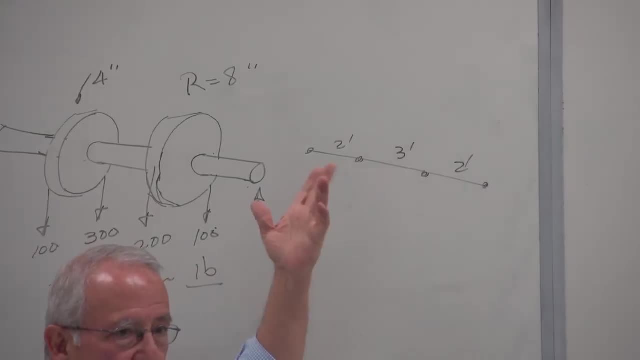 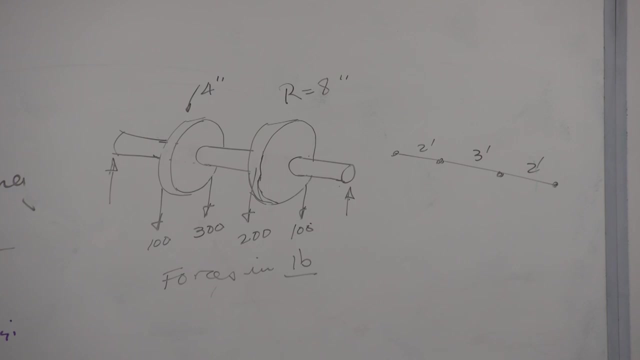 This is the location of the two pulleys. Those are the distances in between them, One of the things that you have to be sure of and if given in a problem, for example, something like this and this load is not given, so F the question is the first question. 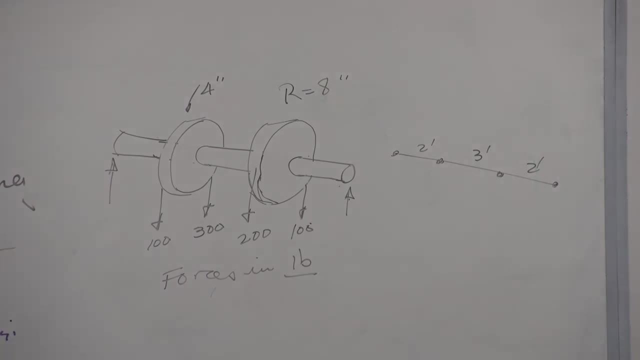 is what's F? Even though this is a shaft and it rotates, it must be in equilibrium, Okay, Okay. So you do know that equilibrium does not mean the state of the material being stationary, not moving. That is not what it means. 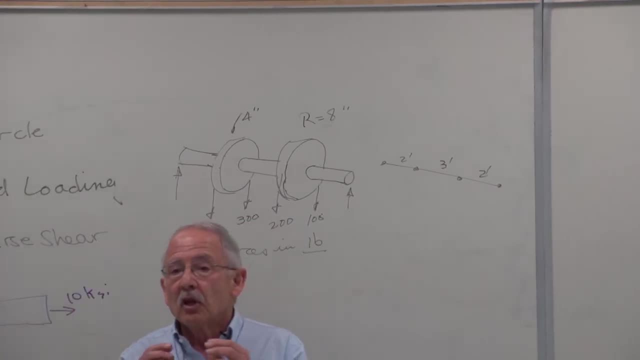 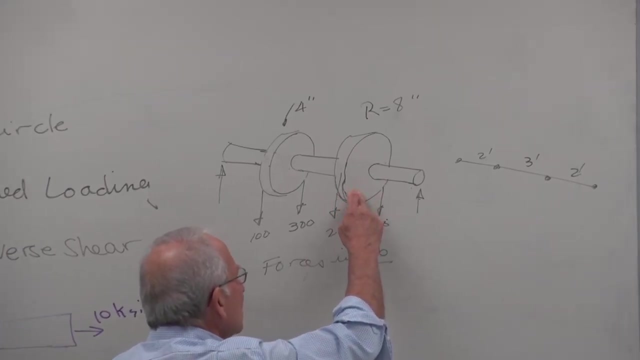 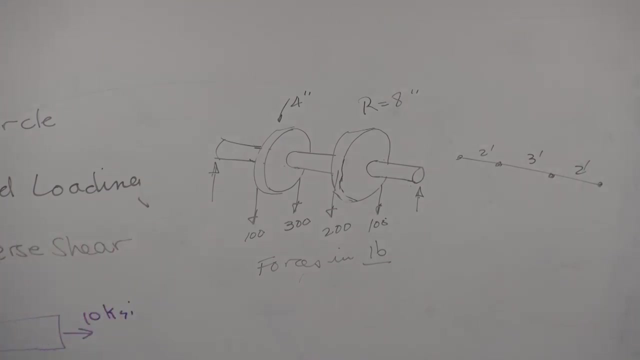 It can be, but it doesn't have to be. Any motion has to be with constant speed, whether rotational or linear. So in this case, if it's constant speed, Okay, Then that means that the torque that's being applied on the two sides by these two pulleys 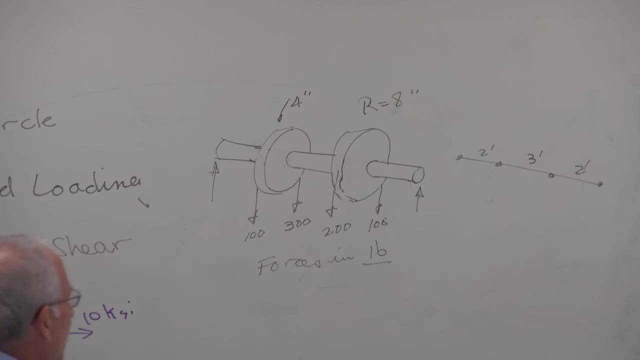 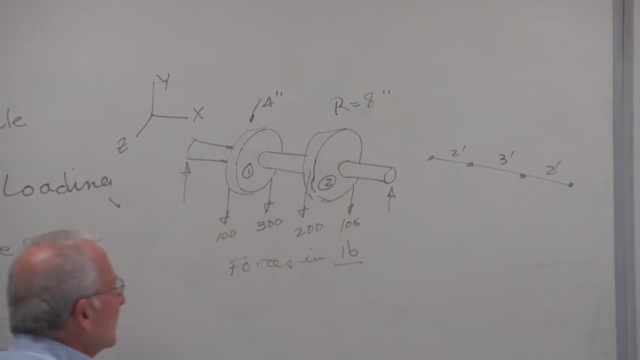 must be equal. So if these are my axes and if I call this pulley one and that pulley two, the forces on pulley one create a torque. Okay. So if I call this pulley one and that pulley two is equal to two hundred times two inch. 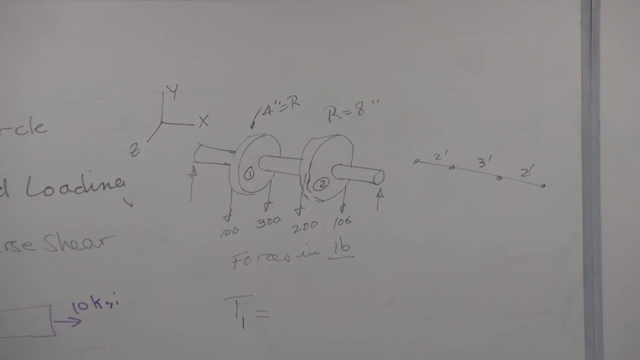 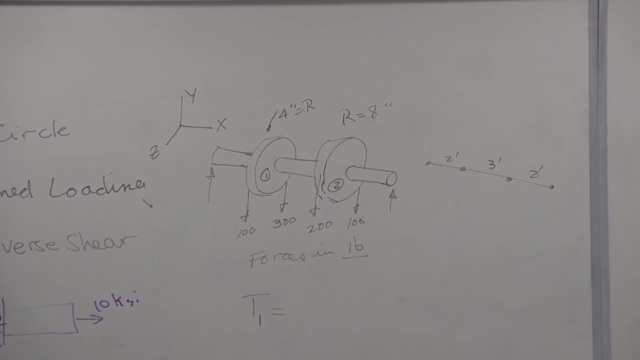 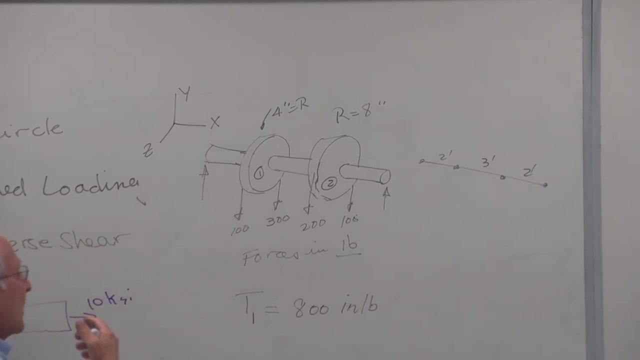 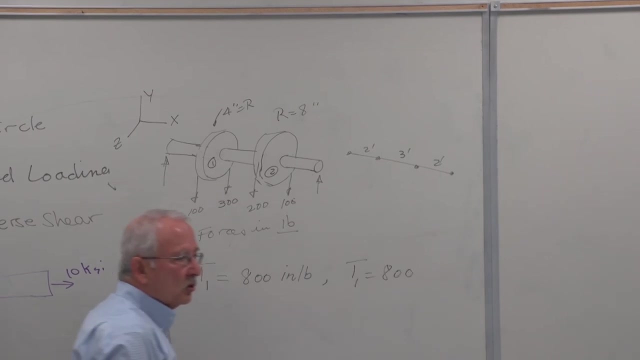 or four inches, I say radius. four inches, that's okay. Two hundred times four inches, that's eight hundred inch pounds. And if I were to write this in vectorial notation, Okay, Okay, Okay, Okay, What would be the unit vector? 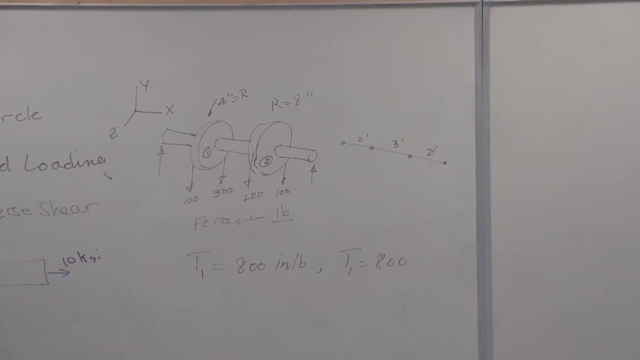 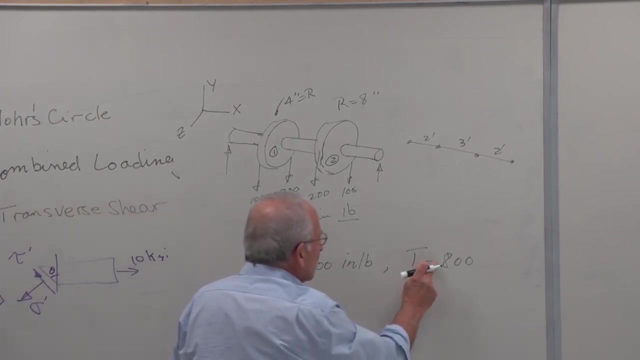 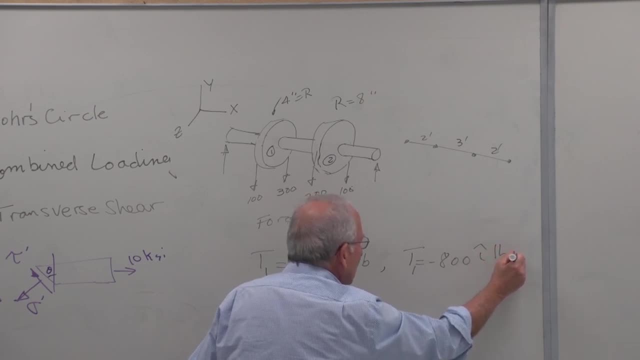 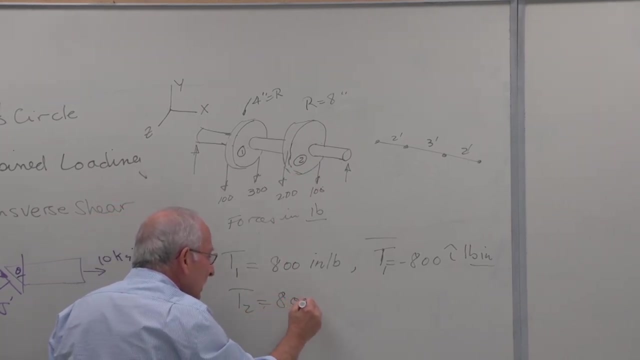 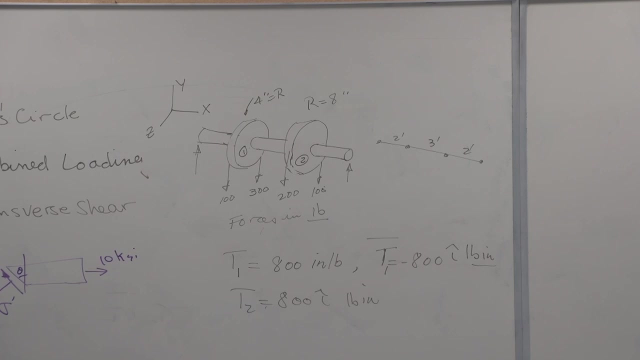 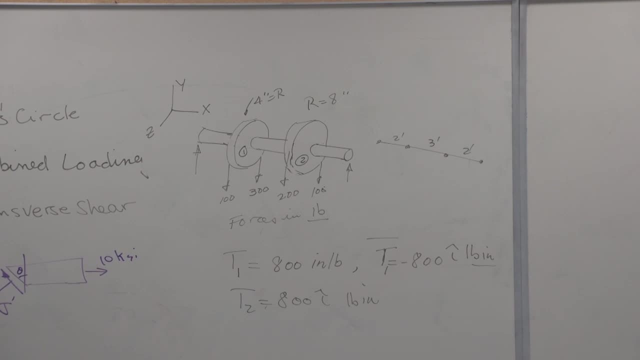 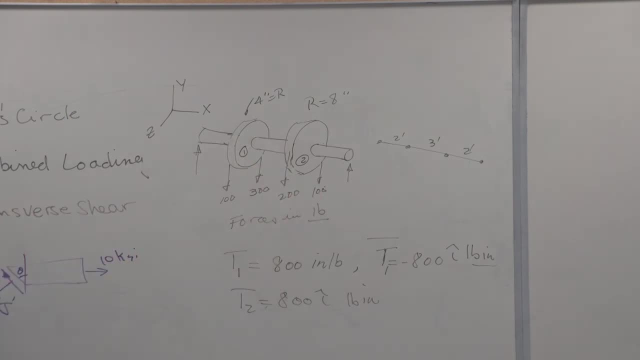 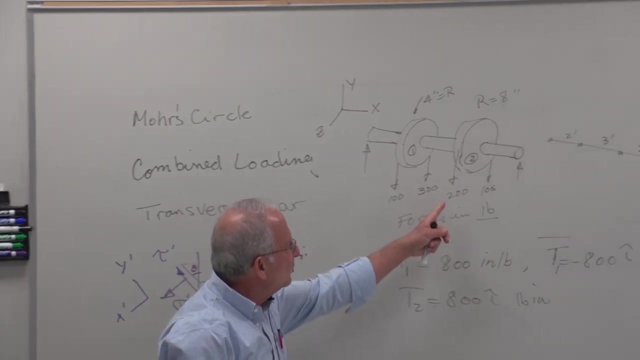 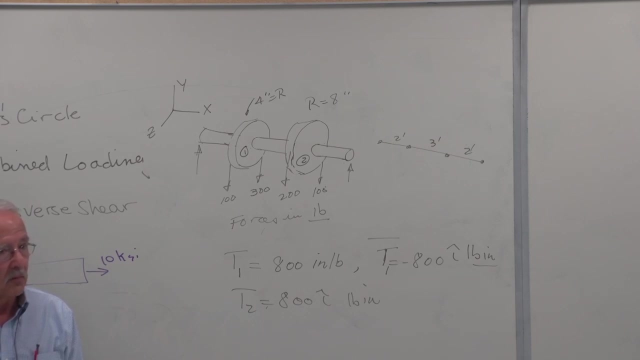 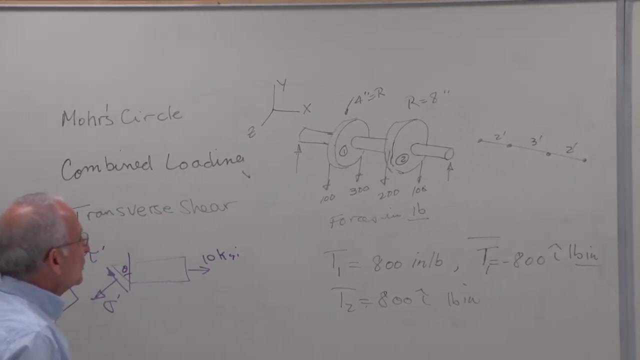 must be 100.. Does that make sense? Is that okay with everybody? If you take a look at that, it will also give you 800 pound-inch, except that it is in the positive x direction. Okay, And let us assume that the question is this: What is the location of the maximum? 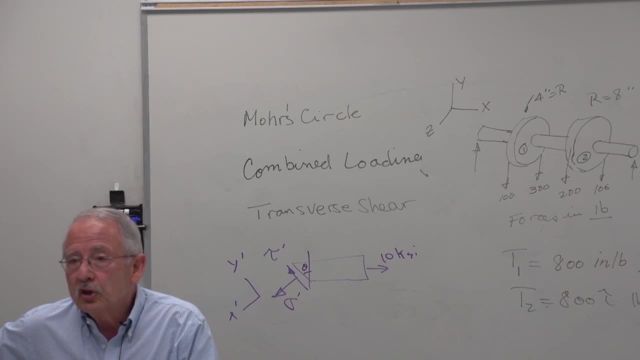 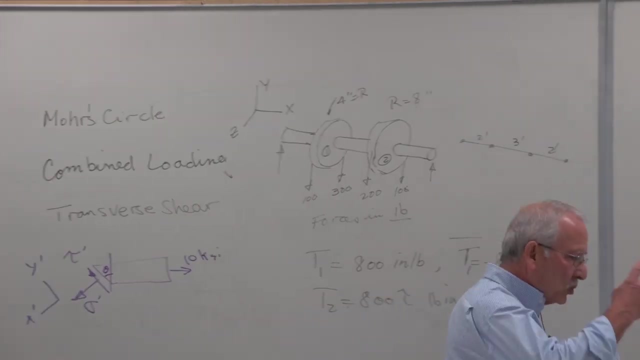 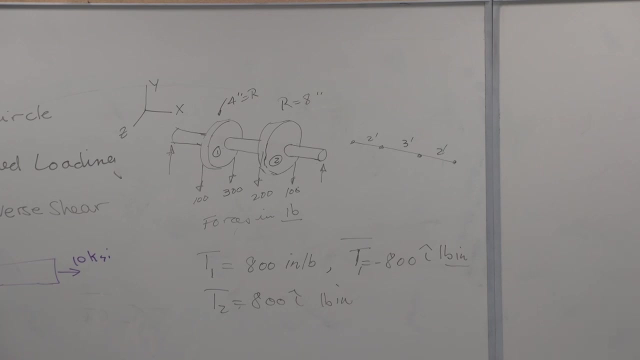 stress in this shaft and what are the stresses at that location? By location we mean cross section and a point which is usually on the outside of the shaft, because that's the point where both the shear and the normal stresses are generally maximum. That's not. 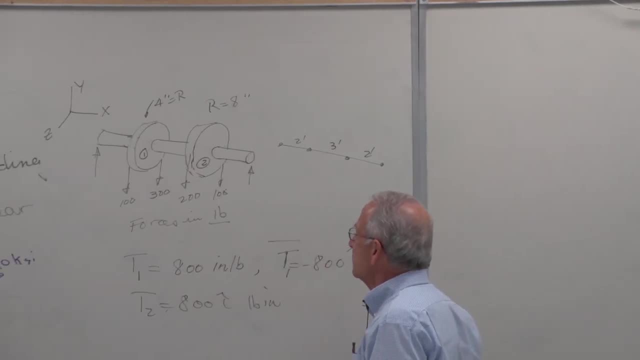 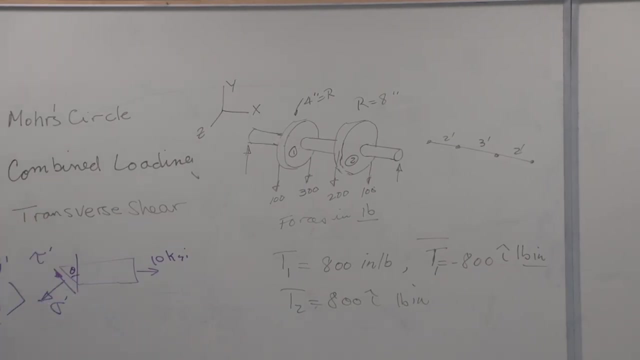 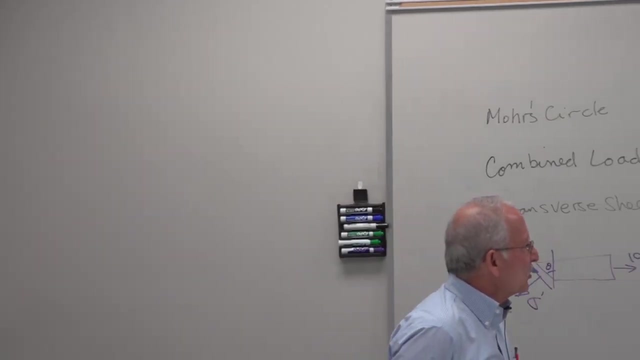 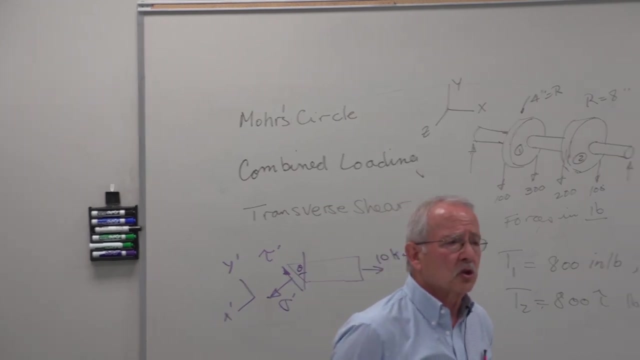 the case if there is stress concentration, of course, but not in this case. So if that is the case, what part of the shaft should I be looking at in order to find the location of the maximum stress or stresses? First, what about the shear stress? Where does it act? Maximum shear stress? I'm not. 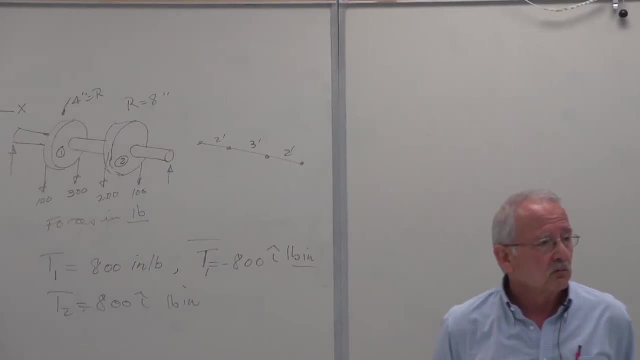 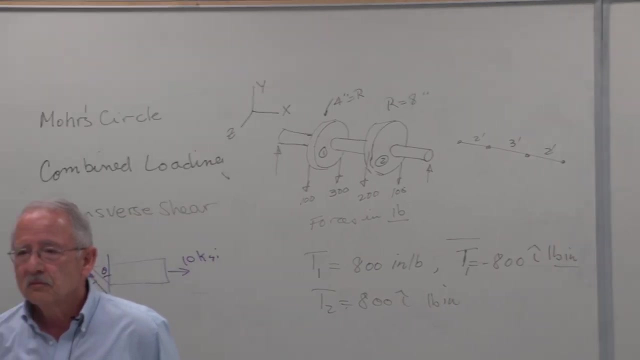 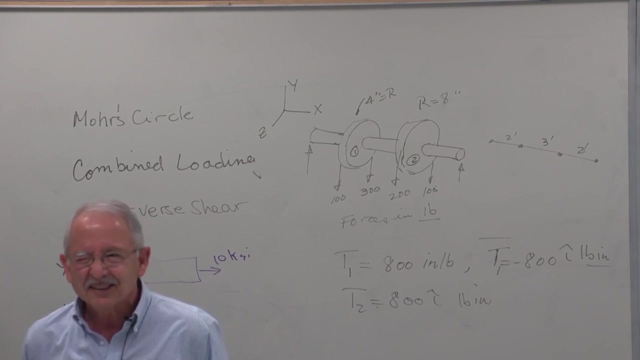 talking Mohr's circle, I'm just talking your regular old shear stress from the Tc over J equation. Where does it act? Throughout the center of the shaft? Oh, yeah, yeah, yeah, yeah yeah. Remember the stress distribution. 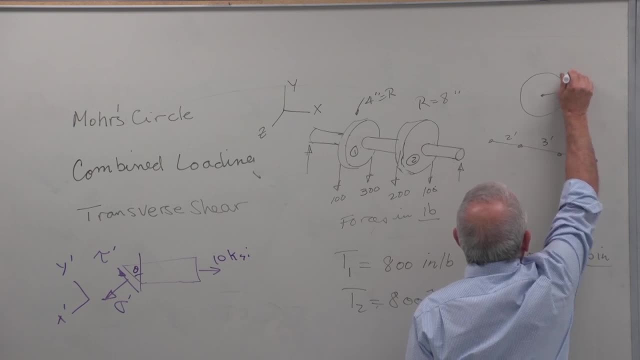 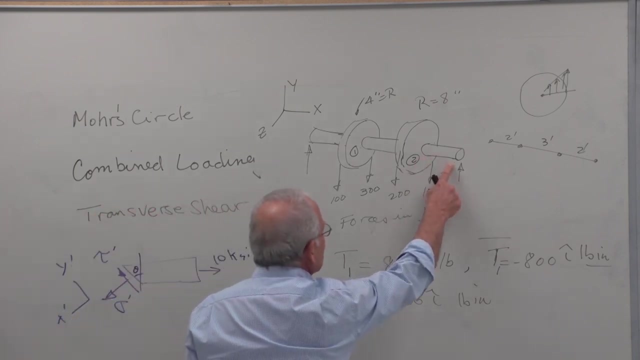 At the outside of the shaft. But where in the shaft, Here, here or here or any other point in between or section in between- Where does the maximum shear stress occur? I hope you're just bashful, Because that you should be able to answer. What's the torque here in this section? 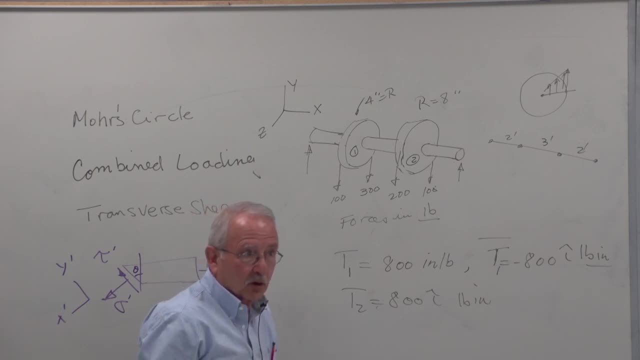 Zero, Zero. There is no torque, That section Zero In between. So the maximum shear stress occurs from here to here. So it occurs on the left-hand side, immediately on the left-hand side of pulley two, or immediately on the right-hand side of pulley one, and every place in between. 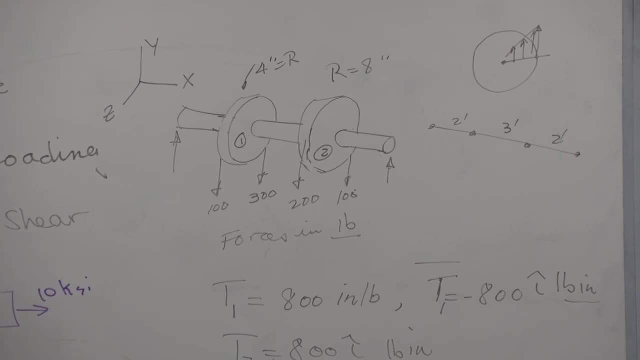 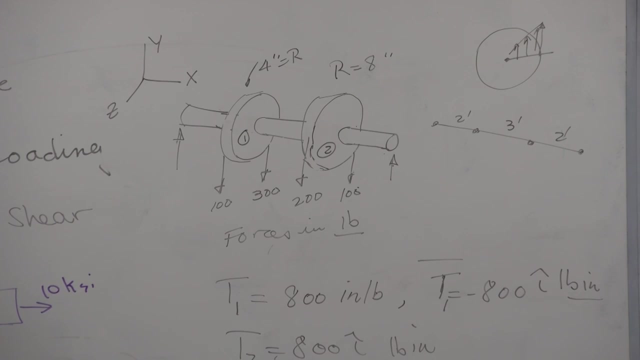 those two Okay. However, the shear stress is not the only stress that acts on this shaft. There is also a bending moment, which creates a normal stress. In order to be able to answer the question, what is the most critical section of the shaft? 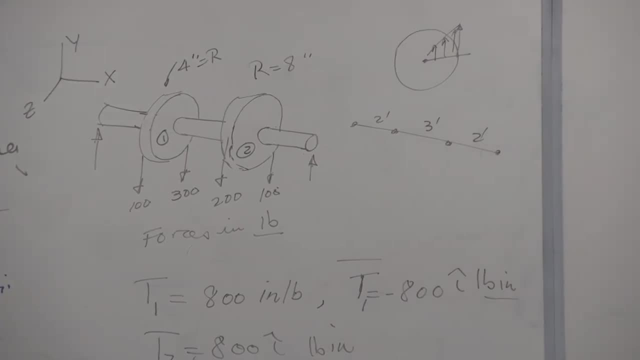 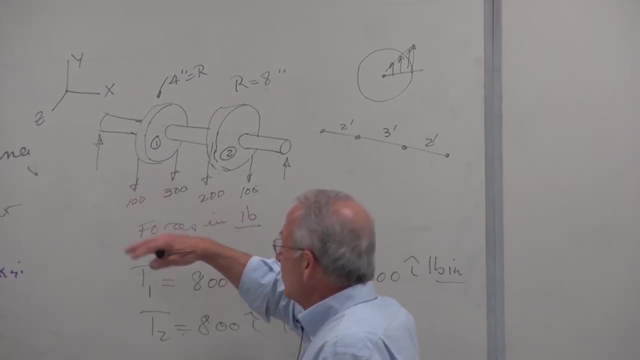 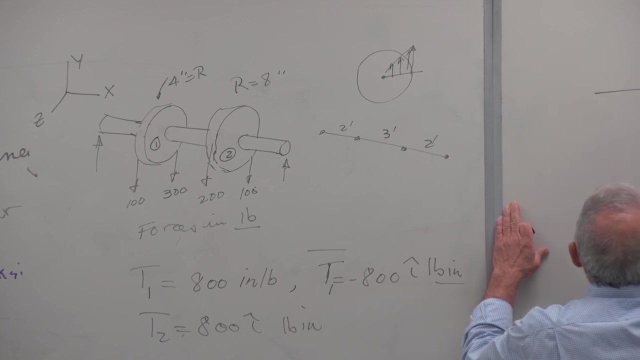 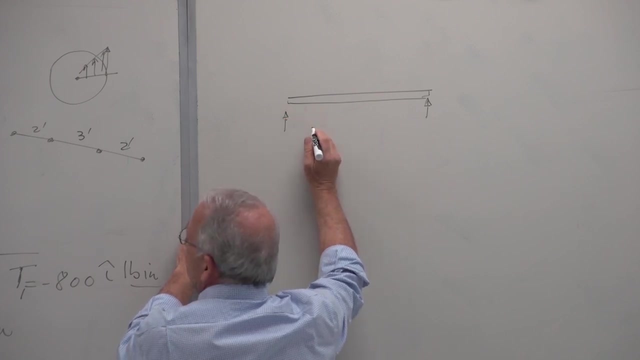 Zero, Zero. Not only do we need the maximum shear stress location, we also need the maximum normal stress location. To do that, you have to draw a shear and moment diagram, So this would be a good exercise in that as well. We draw the shaft like this, And then we have 400. 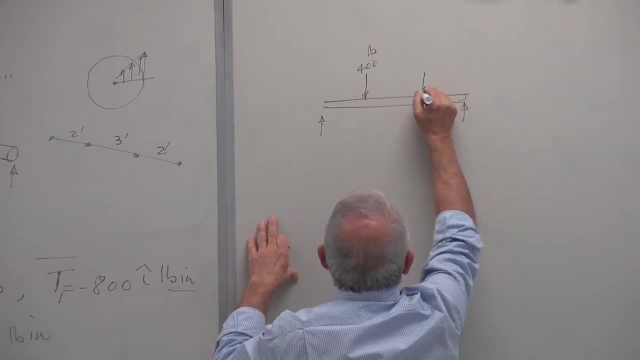 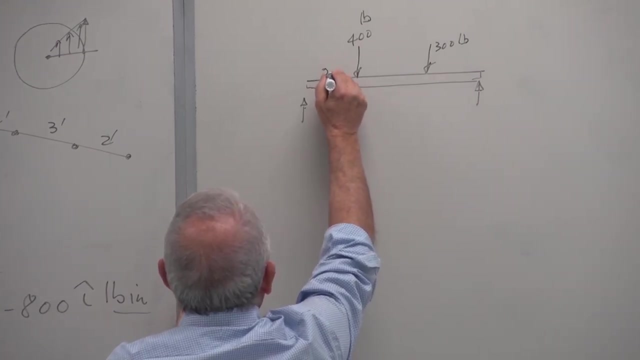 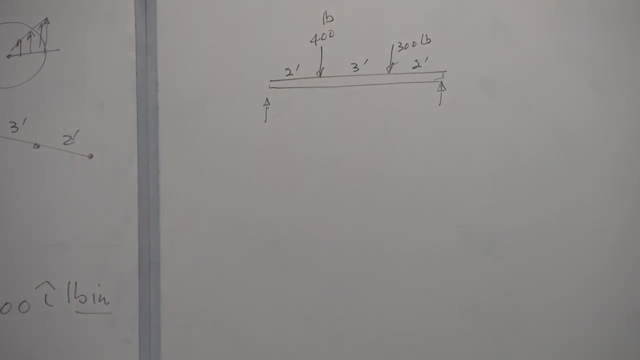 pounds here and 300 pounds there, and this is 2 feet 3 feet, 2 feet. okay, You can draw shear and moment diagrams, which is really not that big of a deal. you, just for the shear diagram, follow the load. 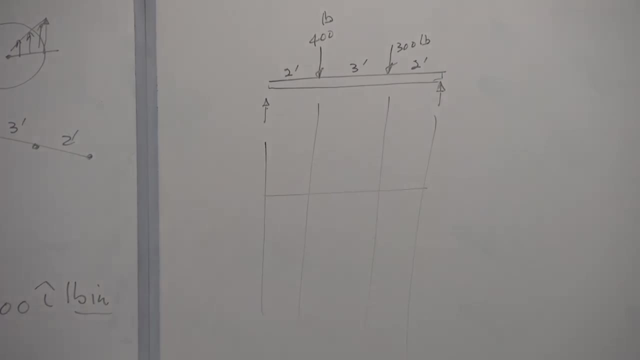 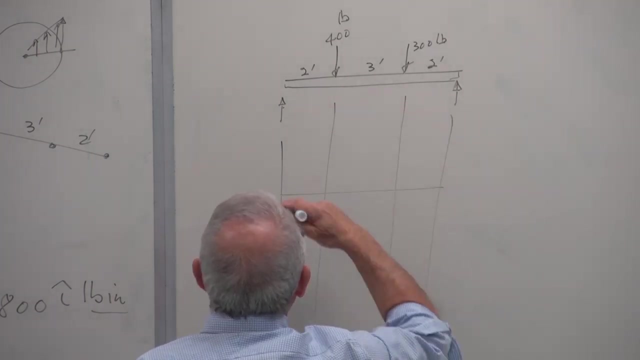 Go wherever the load goes. First, of course, you have to find: let's see, let's see, let's see, that's 4, so, ah, good, good, good, Yeah, it'll work for one, but not the other. 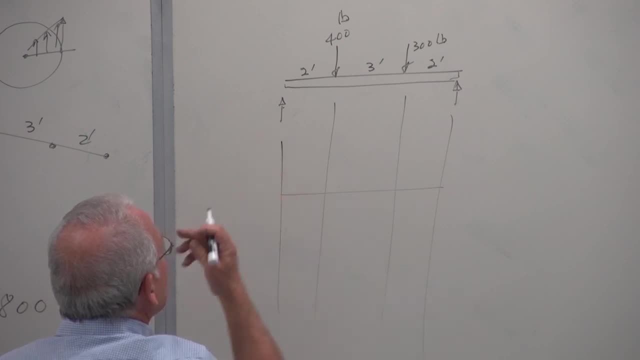 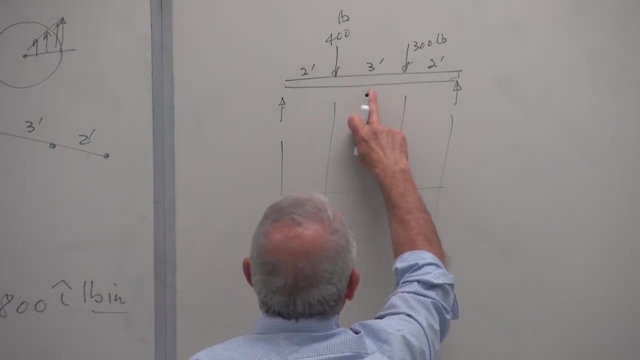 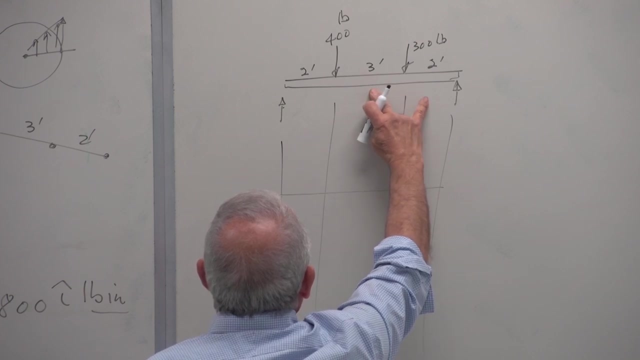 I want to change those numbers. I don't remember the numbers from the previous section. I want to change those numbers so that we get round numbers for the reactions. I make that 4, and then I get 3 and 1. And if I make that, 4.. 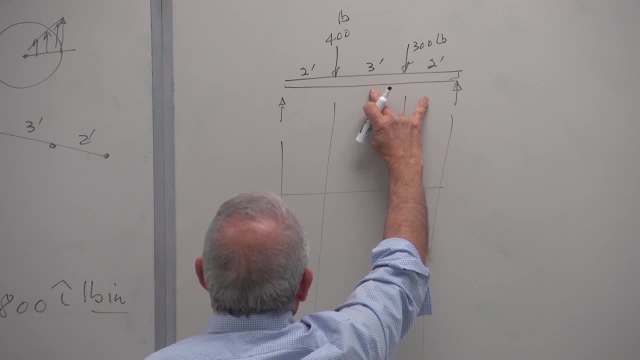 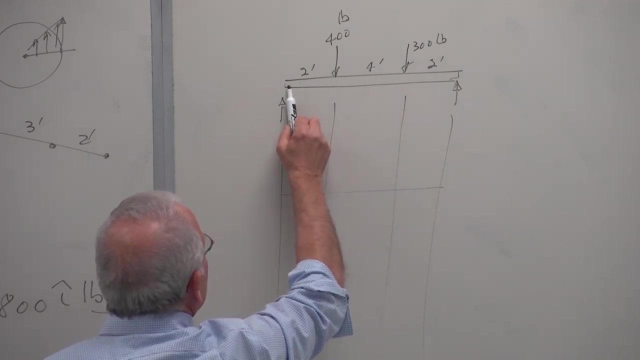 Okay, that 4,. I may get 3 and 1.. It may turn out to be OK, let's see. I don't want to write equilibrium equations just yet, So I'll show you where I get these numbers. That's 6, 2, so 1 third and 2 thirds. 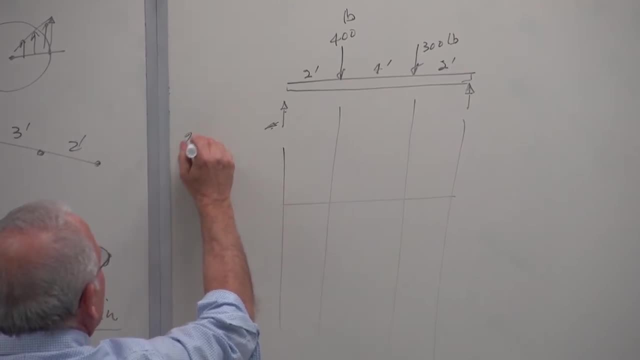 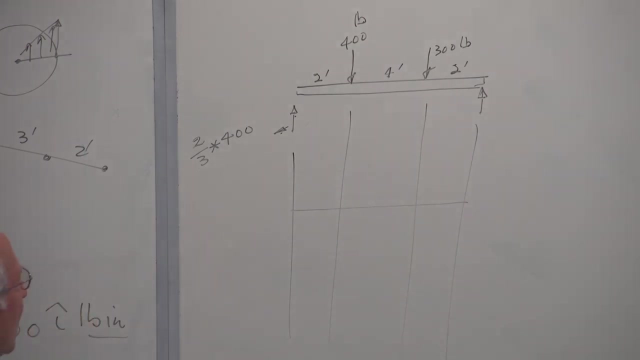 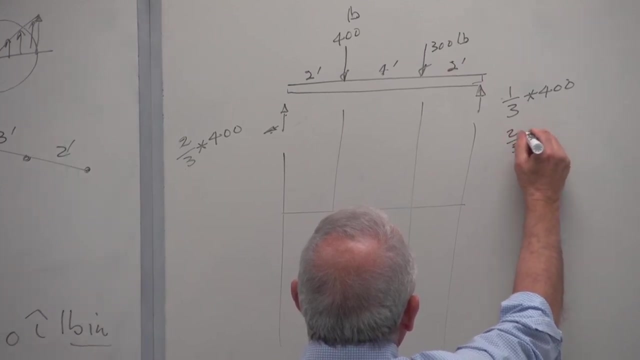 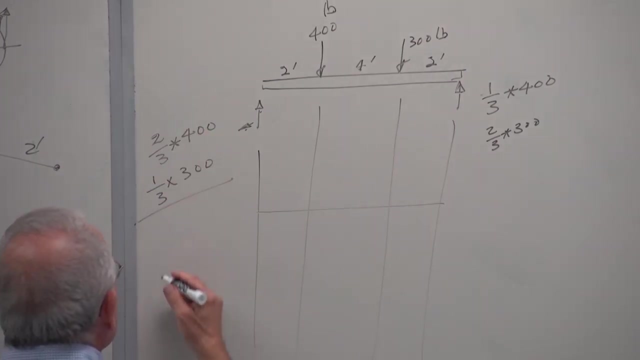 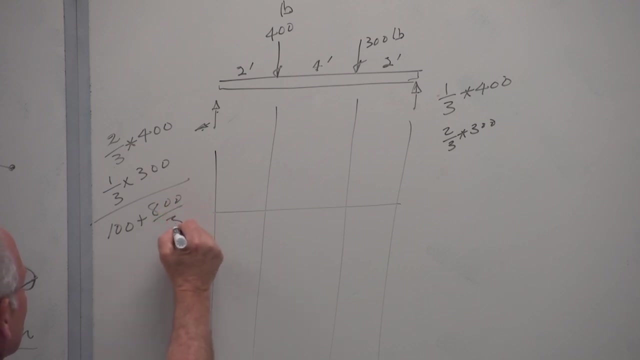 So this is equal to 2 thirds of 400. And that's equal to 1 third of 400,. then this will be equal to 2 thirds of 300, 1 third of 300. If you add those, two would be the reactions, So it's 100 plus 800 over 3, and this is equal to 400 over 3 plus. 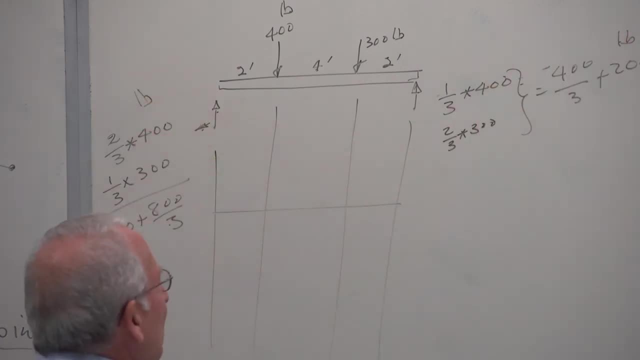 200 pounds. We'll figure out what they are. Now that we're on the subject, let me show you how you get that. If you have a simply supported beam, which that is, if this is a force F, this is A and that's B- Yes, you can write equilibrium equations and find the 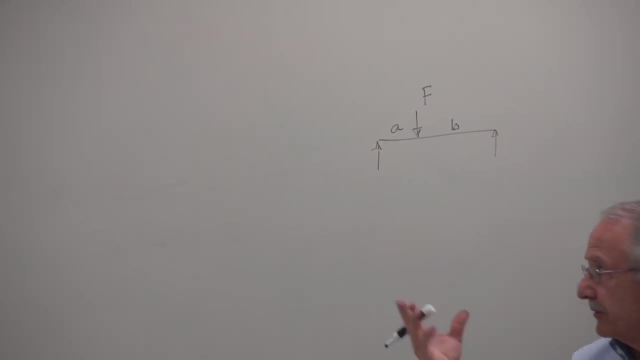 reactions. But if you remember this, the easy way is to say that this is divided between these two supports in the ratio of these two distances, And it's clearly the reaction due to that force is larger at the left side than it is on the right side. Therefore, and this will be AF divided by A plus B, That's what I've. 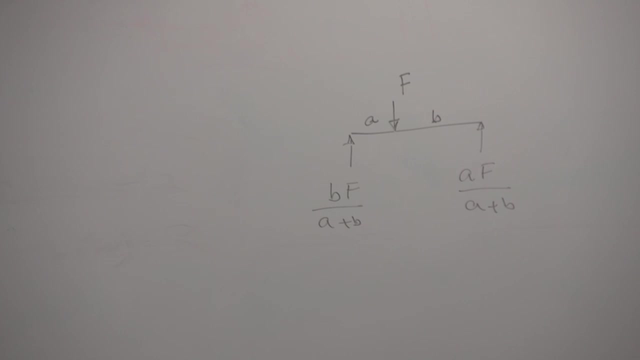 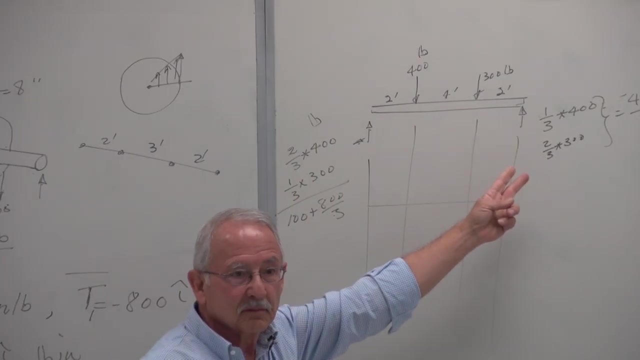 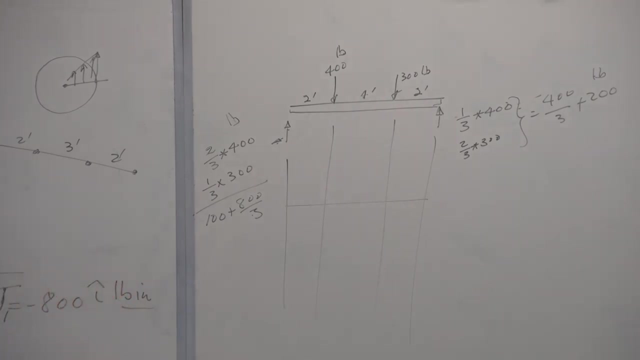 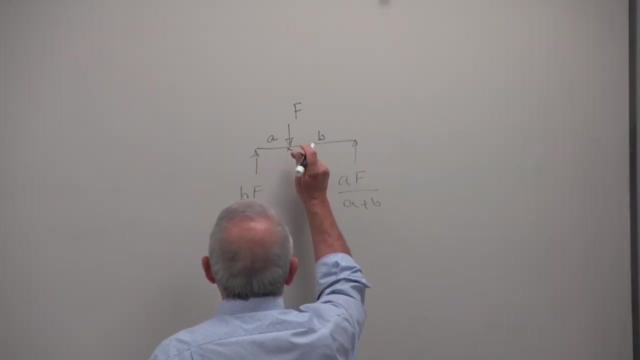 used to come up with that. So I looked at each one of these like that And for each I wrote its own ratio. Then I added them up. But again, if you're more comfortable with equilibrium equations, that's fine. Furthermore, the maximum moment which occurs here this: 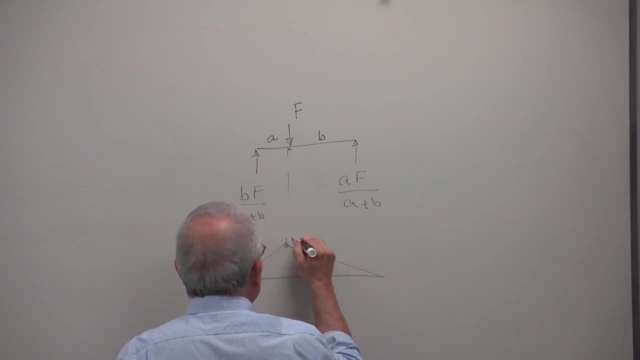 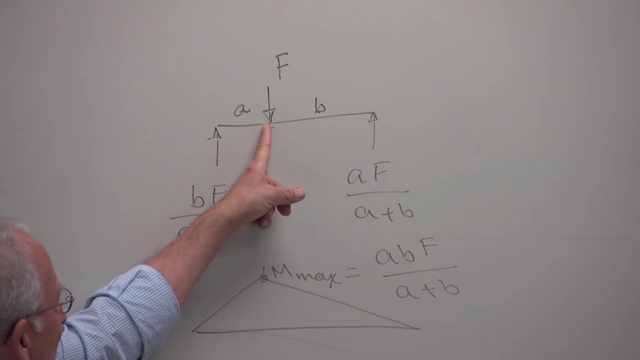 is the moment diagram. Maximum moment is that. All you got to do is cut a section here, And the moment here, just next to F, is equal to A times that, Or, on the other side, B times that. So those are your moments, the. 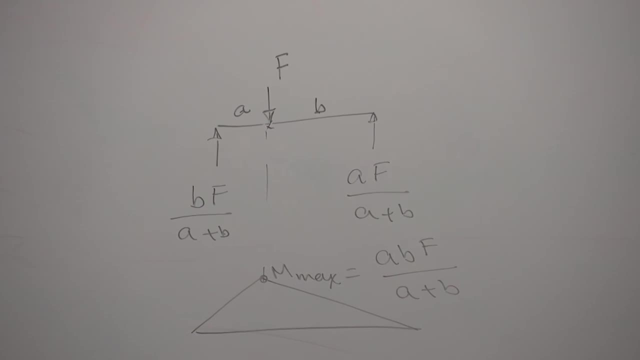 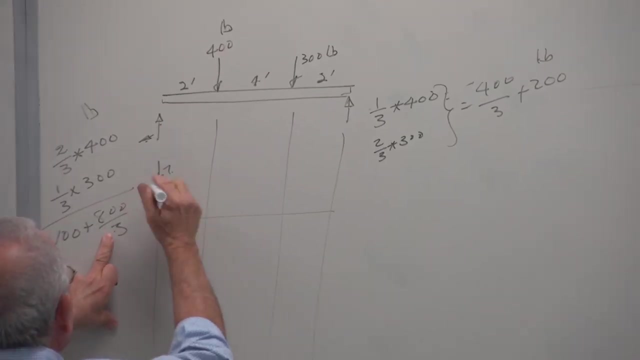 maximum moment and also the reactions for a simply supported. This is something good to have in the back of your mind. Saves you a lot of time. So what is this? This is 800 over 3.. So it is about 267 approximately Plus 1, 367.. And 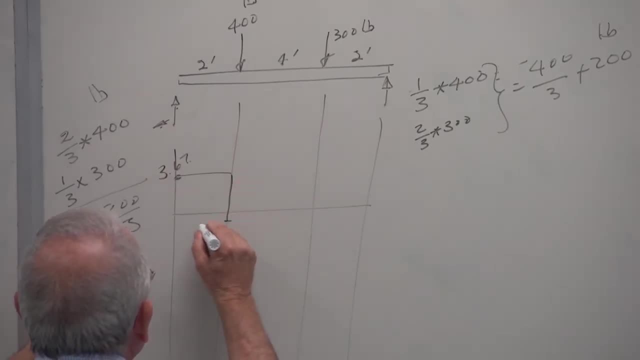 then, from here to here, nothing, So we drop down to 33.. And then nothing from here to here, when following the load, And 333.. And the sum of these better be 333.. It is right, Sir. How come it's one, two, three instead of three, four? 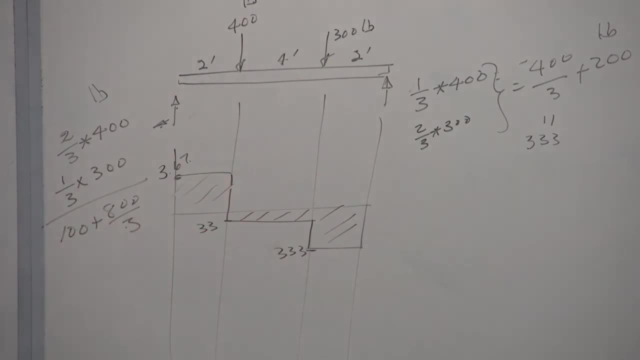 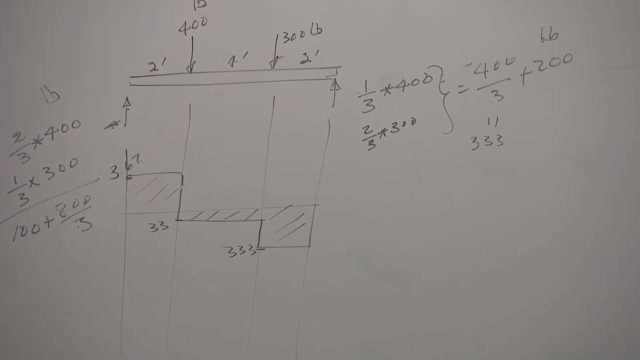 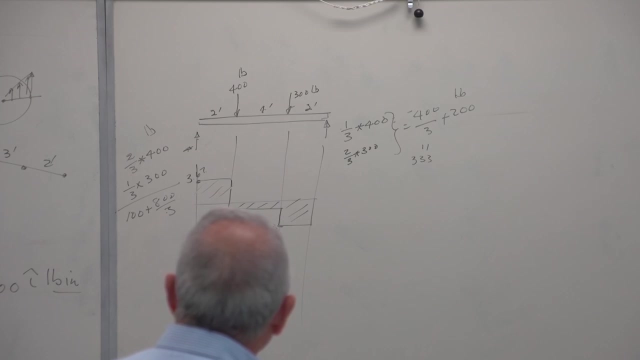 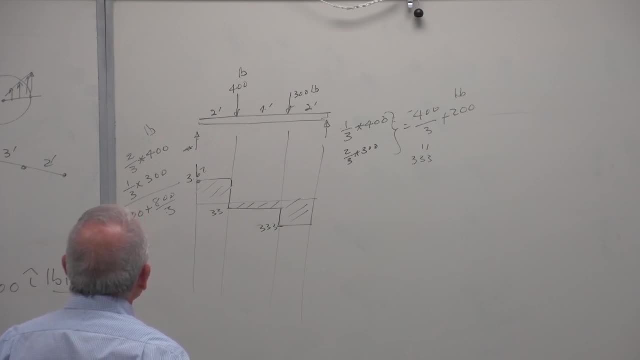 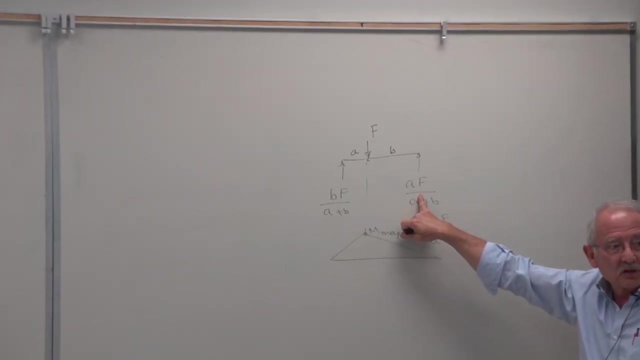 Oh, okay, Let's see. let's see, It's two eights. yeah, you're right, I divided it in the ratio of these two. So here's what I did. This has to be divided into these two parts, right? 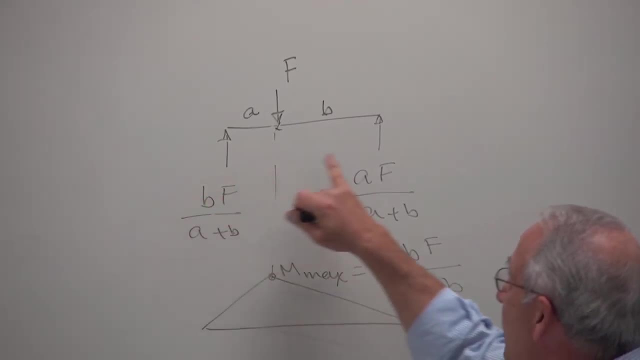 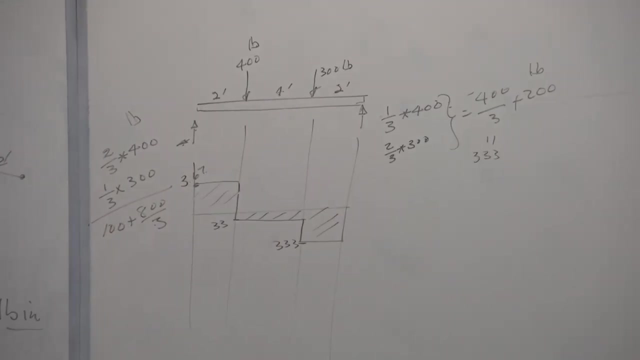 This one or this one is A over B times that one Ratio of those two A and B, Correct? So come in here. the ratio is two to six, One to three. okay, Two to six, And then you do the moment diagram. 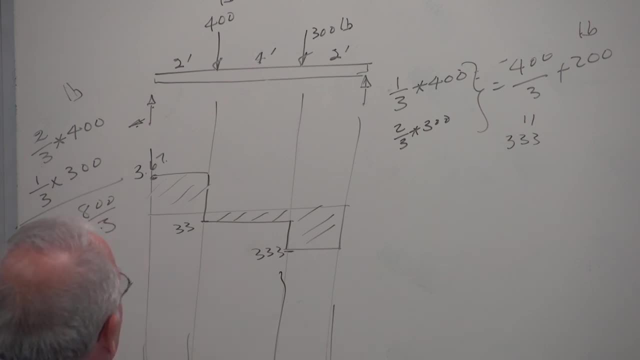 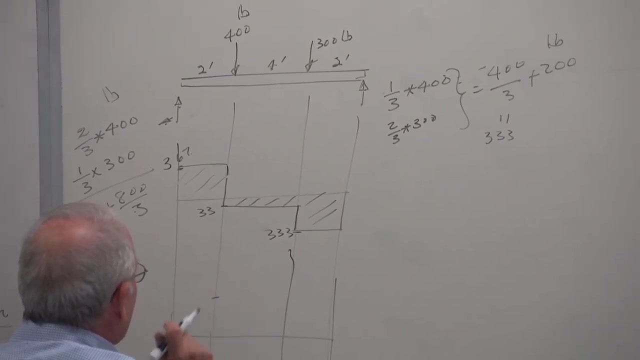 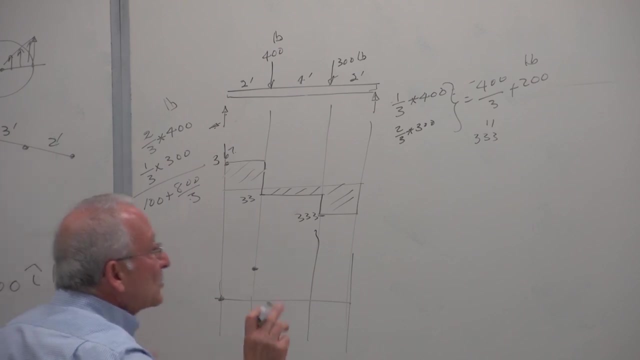 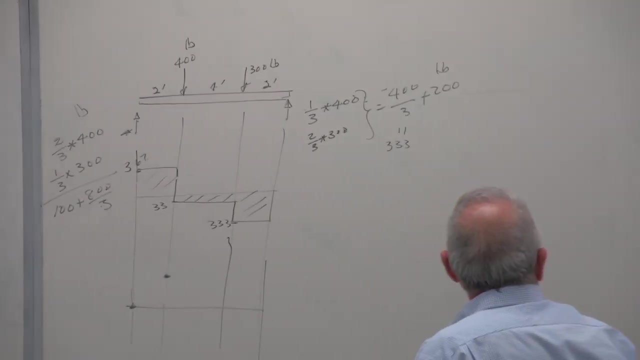 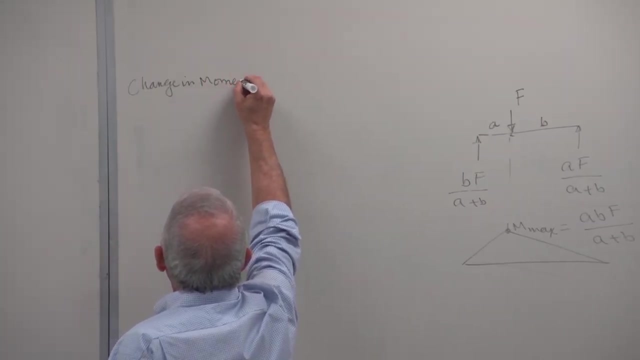 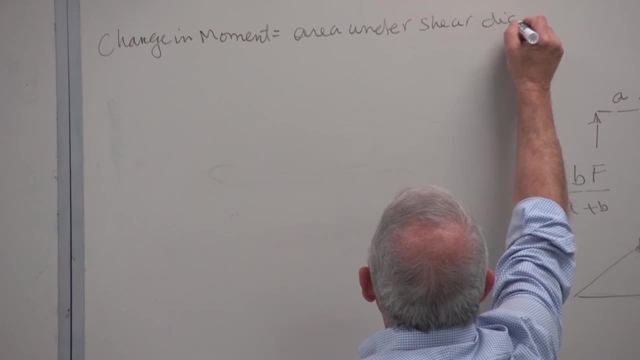 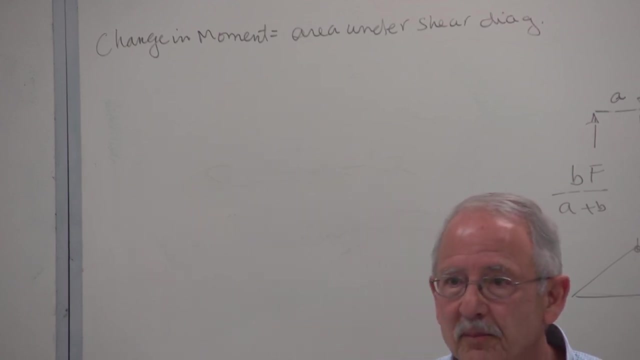 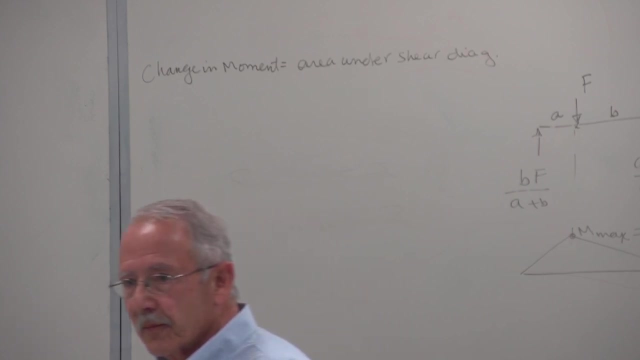 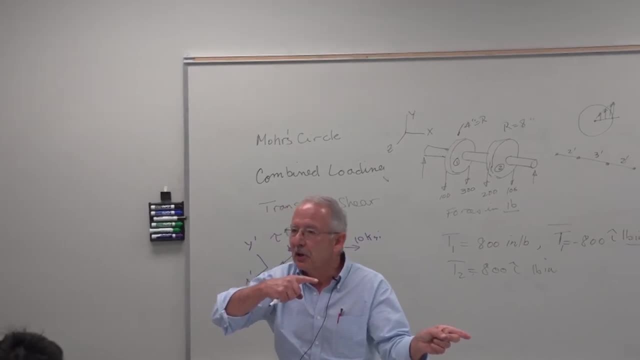 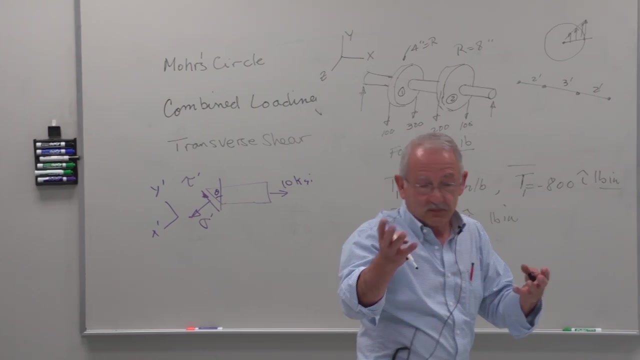 Torque may not be there, but the shear stress from the bending diagram is there. On the other hand, that one may not be there, but the torque is there. so you get it, But in general you're right, Correct. 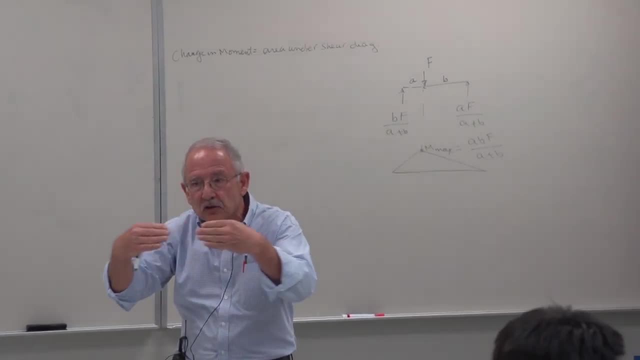 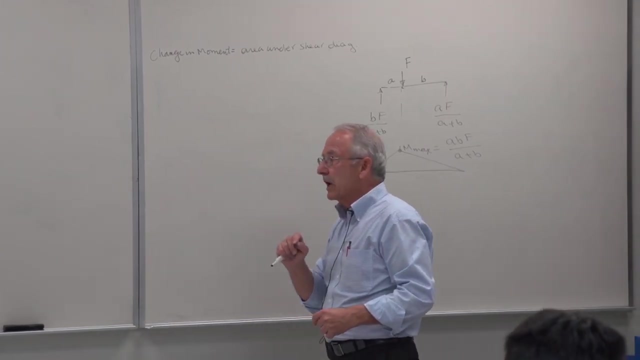 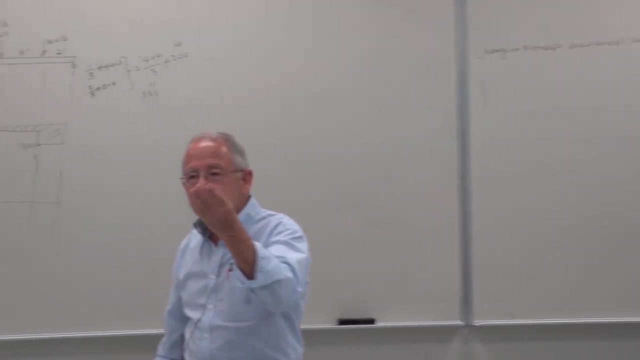 Both of them are there, so they're either additive or subtractive. depending on whether they both act in the same direction or they act in opposite directions, They may be additive or subtractive. That's number one. Number two, the transverse shear which I have down there. what is the value of the? transverse shear at the surface: Zero Zero. It's maximum at the neutral axis, right. What's the maximum value of the shear stress due to torque? Where does it occur? Surface Zero at the neutral axis? Yes, there are these two shear stresses and in some locations they add to one another. 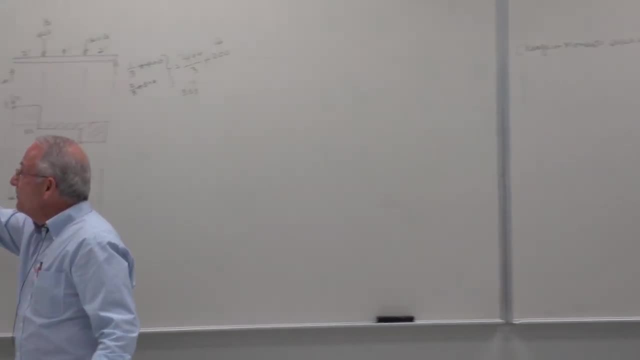 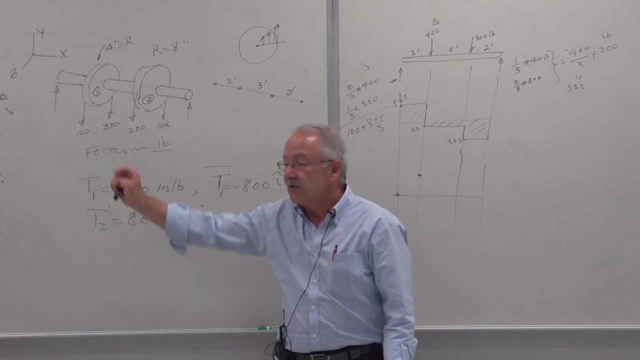 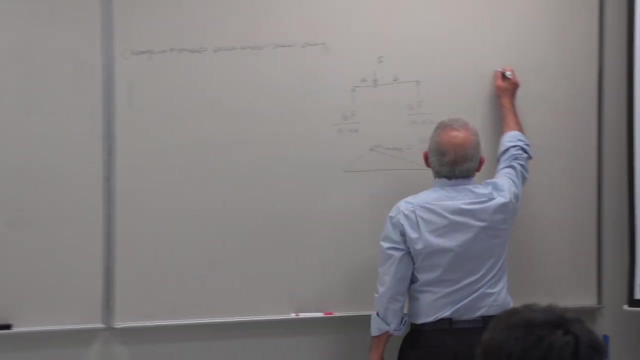 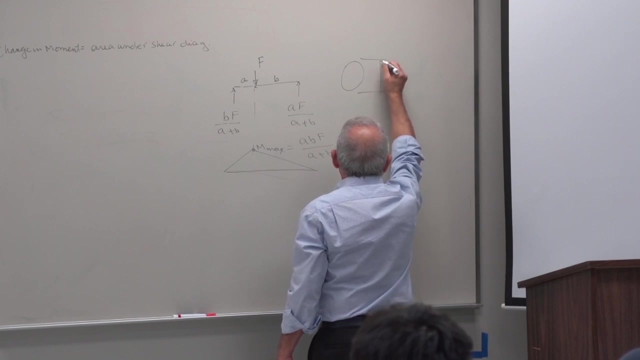 But at the point of interest that we have on the surface of this, only the torque has a value. The transverse shear is zero. Remember. it looks like this: The variation of the shear stress. I have to continue writing that If this is your cross-sectional area, that's the transverse shear. 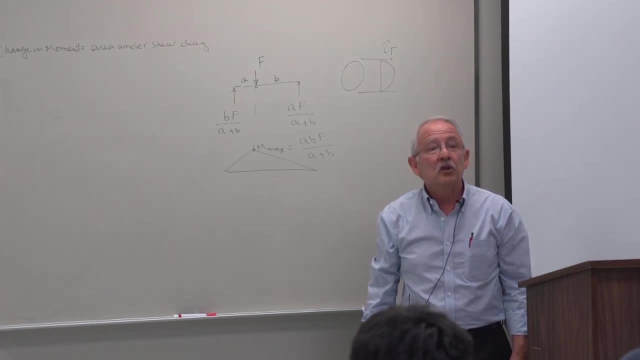 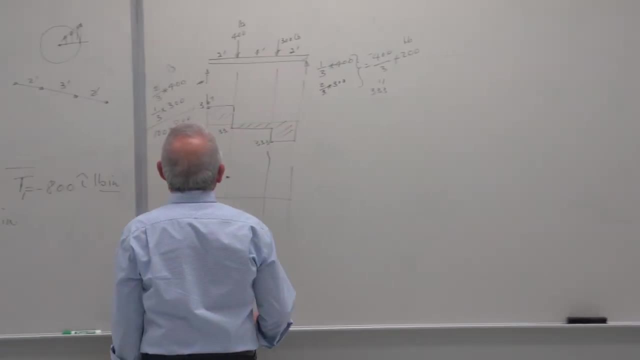 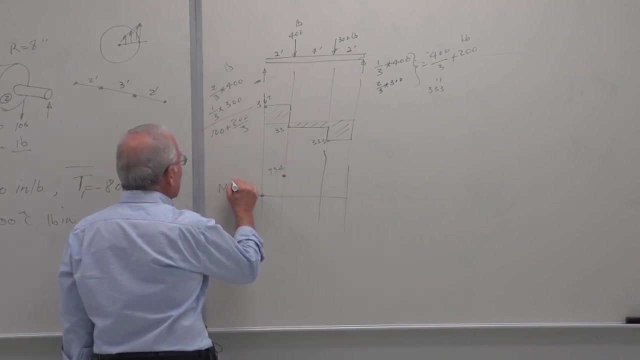 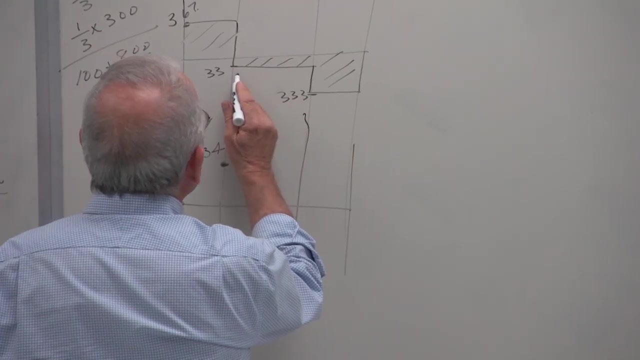 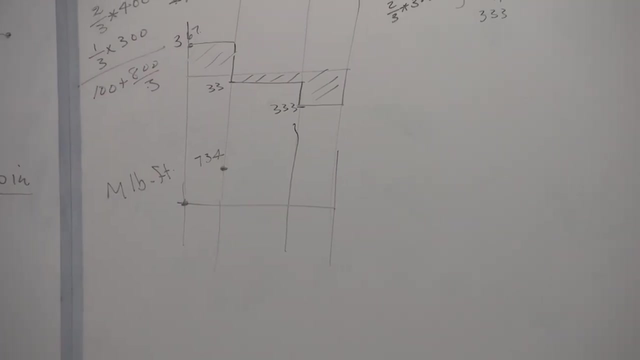 Agreed. So it's zero on the surface. So we get that torque. Okay, here we have four three seven. Okay, Okay, Four three seven. This is m in pound foot, And then we subtract from that 300 times four, that's 1,200.. 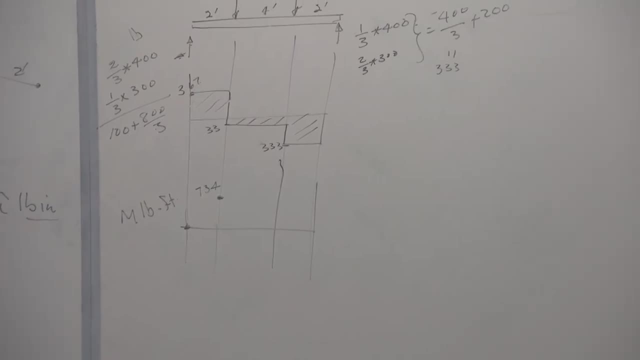 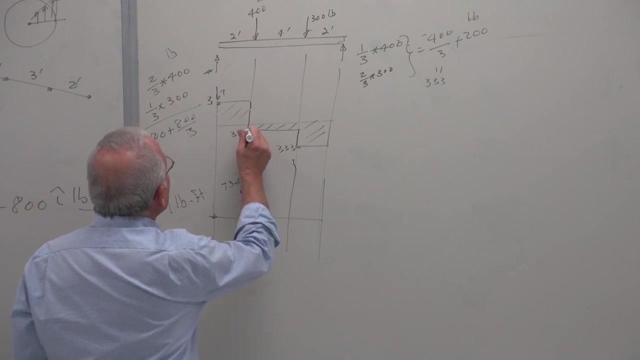 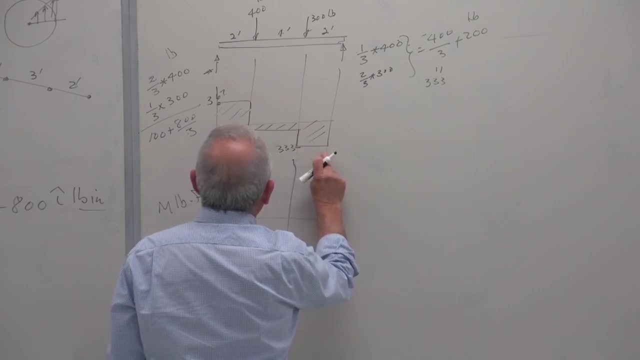 Something is not right. It may be what you were talking about: the eight. Did I do that right? Yeah, that's fine. 433.. 734.. 734.. Well, let's check the reactions. I believe what you said is correct. 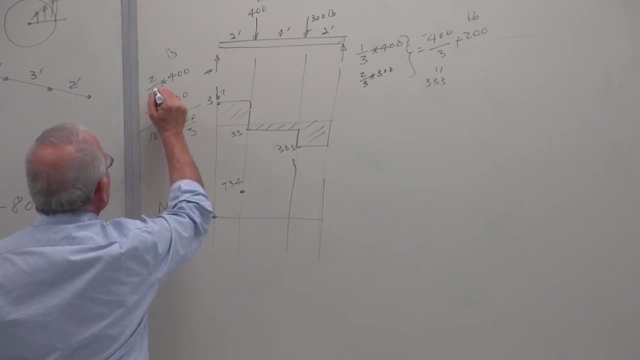 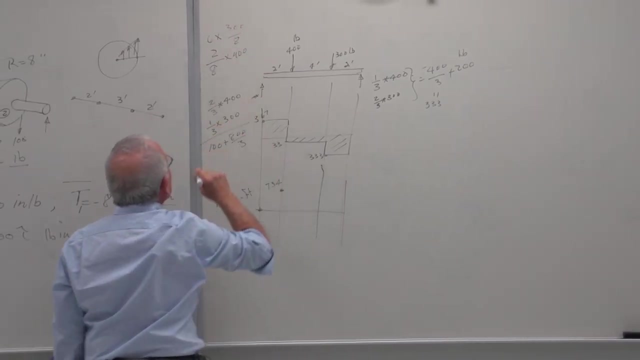 Is two. ah, it's not two-thirds. Okay, Okay, Okay, Okay, Okay, Okay Okay. Let's do the next one. This one is two over eight times 400.. You were right, after all. And from the other one you get six times 300 over eight. 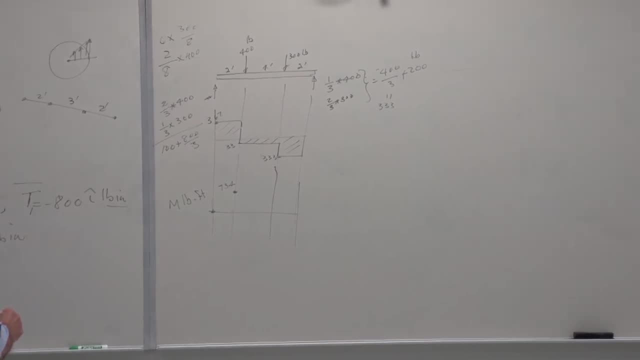 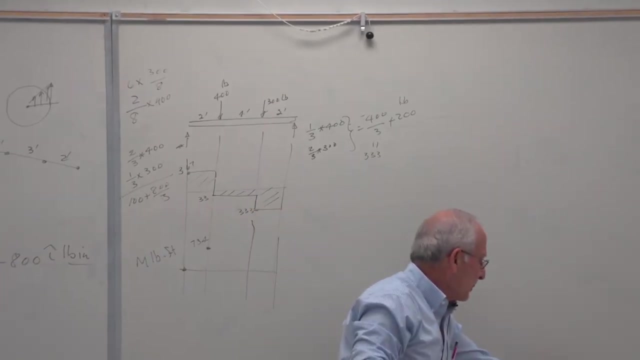 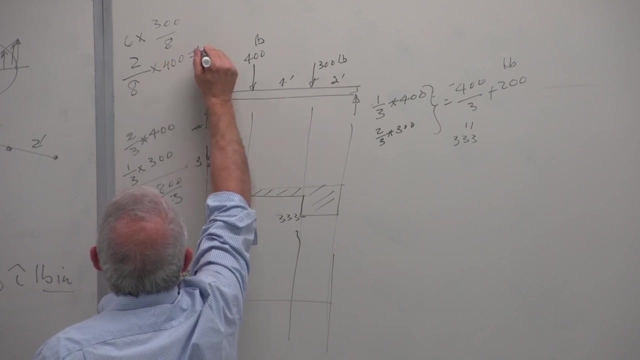 A divided by a plus b in beta. Yeah, I, In reducing the ratios, I made a mistake. So m divided by a plus b in beta. So let's just check this one more time. so that's 800,, that's 100, and what is that? 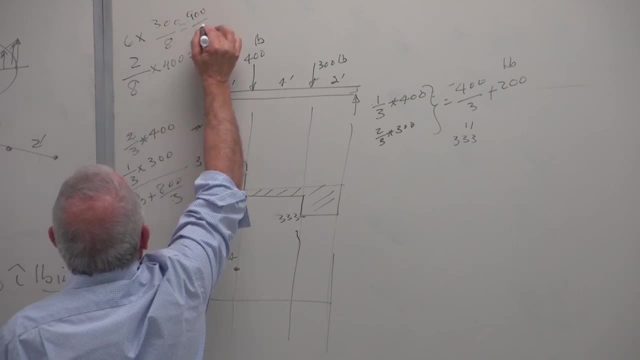 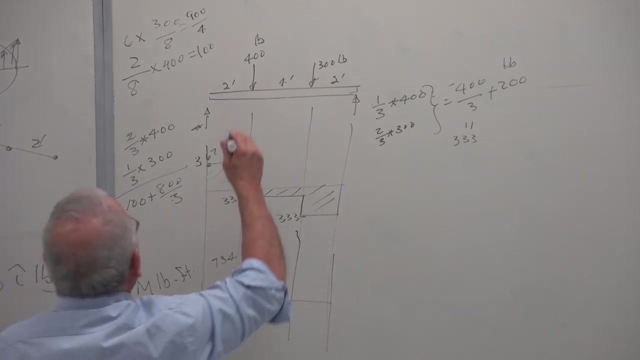 Three quarters, that's 900 over four, And 900 over four is 225.. Add those two and rather than 367, we will have 325,. okay, 325, that still won't give us the right answer, Isn't it? six, eight times 400, and two eight times 300?. 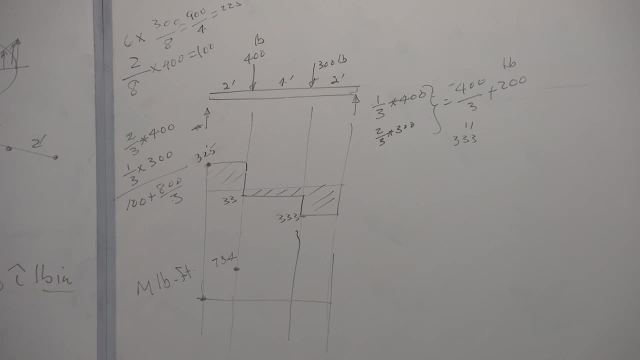 Eight times two divided by eight, sorry, 400 times two divided by eight. It's like in reverse, isn't it? six, eight times 400, and two, eight times 300? Over eight, six times 400, over eight, and. 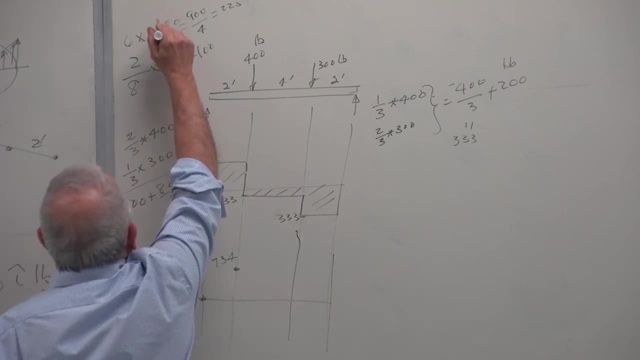 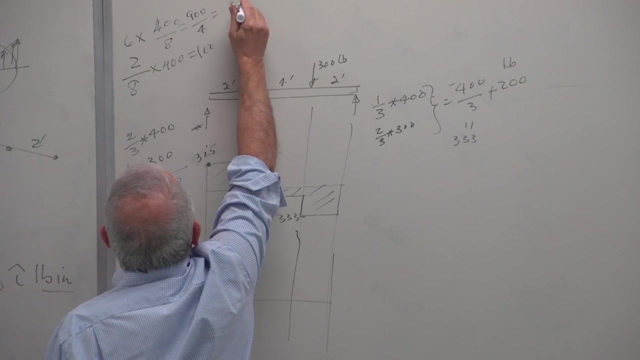 Six times 400, that's right. Okay, one more time. we get two, three, 300, right, Is that right? And the is two over eight times 300.. Yeah, that's correct, So 300, and then this one: 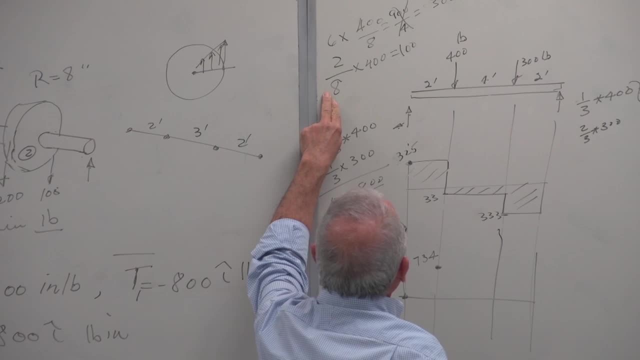 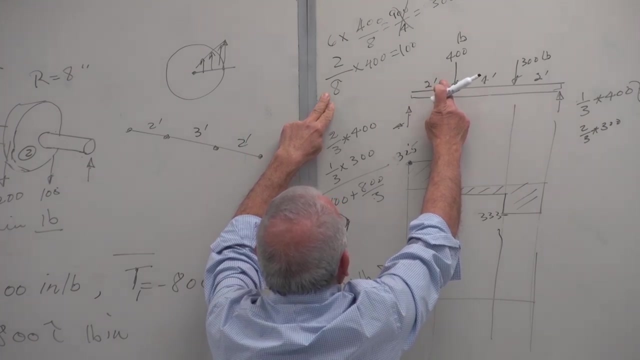 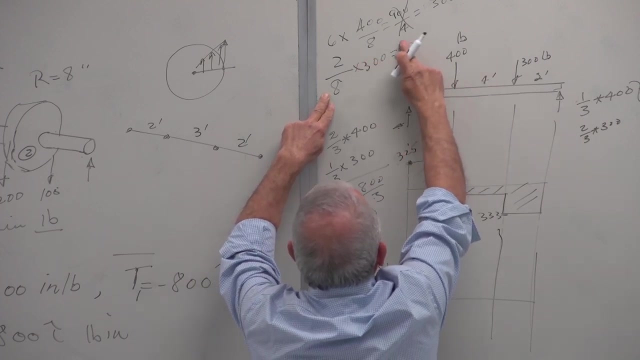 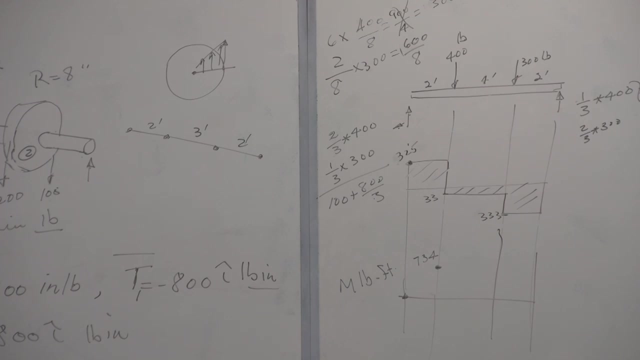 Okay, Oh, I know, I switched those two. Six times 400 divided by eight is correct for that one. Two times 300 over eight is good for this one: 600 over eight. So what do you get if you add those two? calculator anyone? 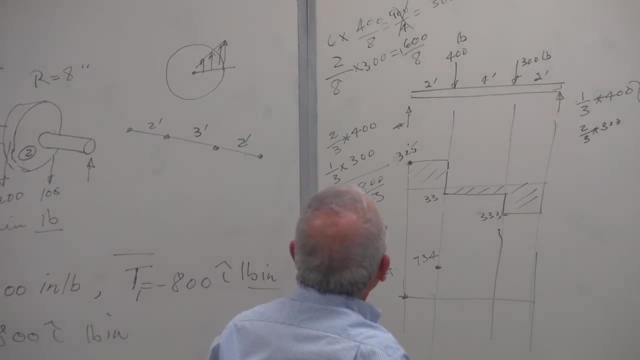 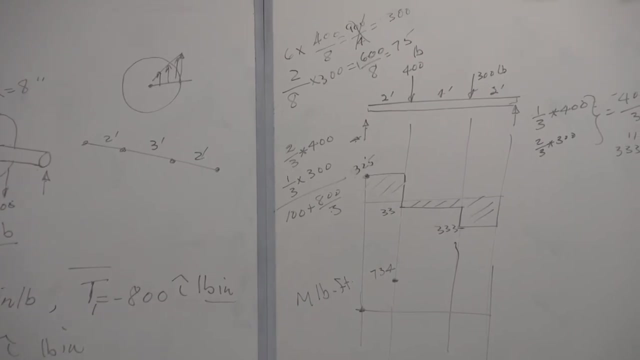 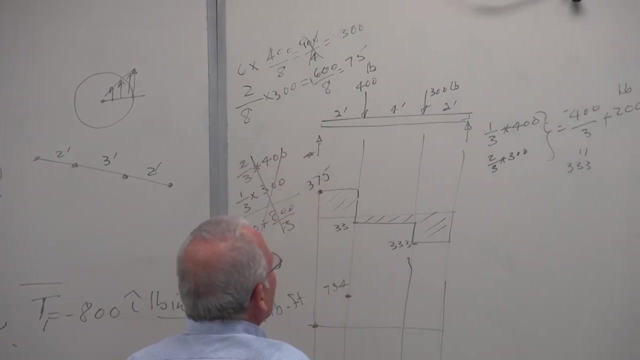 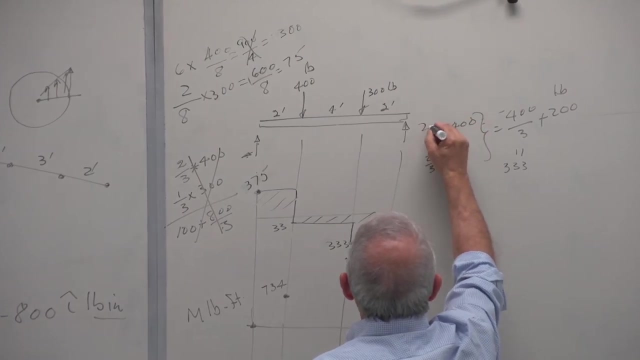 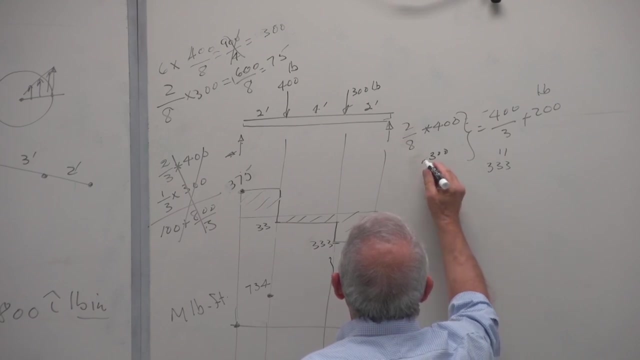 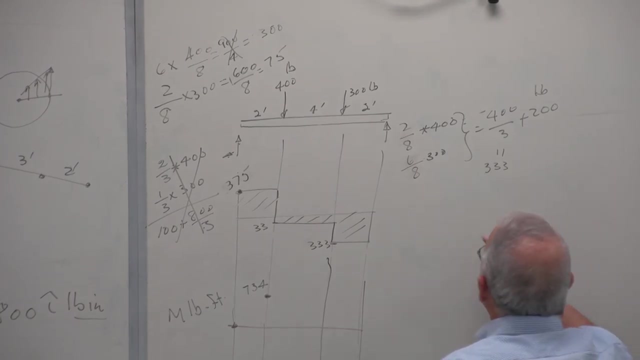 Okay, Divided by four is 150, 75.. Check that correct, So it's 375.. On this side, 400, 205.. Okay, Okay, Okay, All right. So that's two over eight and 300, six over eight. 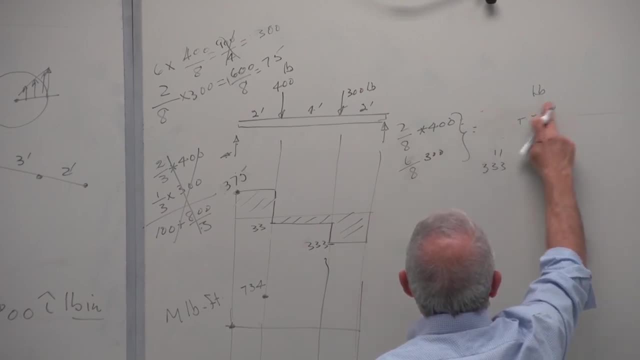 What do we get here? That's 50,, that's 100.. That's 100 plus 1,800 divided by eight, is what? Yeah, Quickly To two, that's 900 divided by four, so 225.. Is that correct? 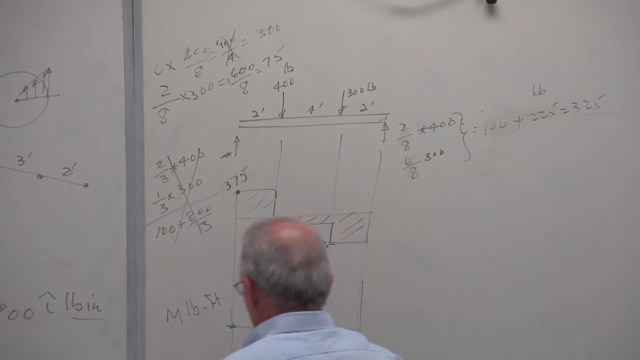 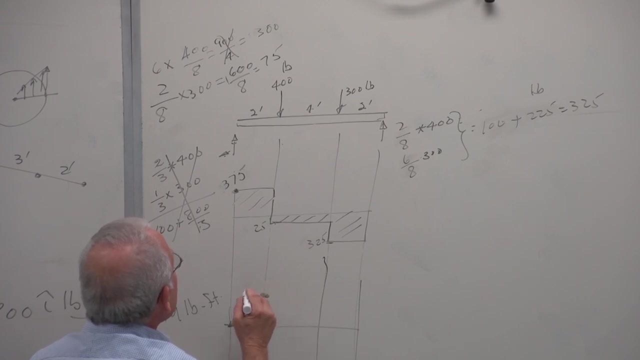 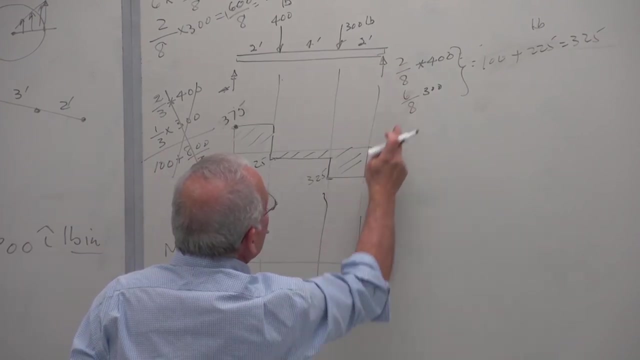 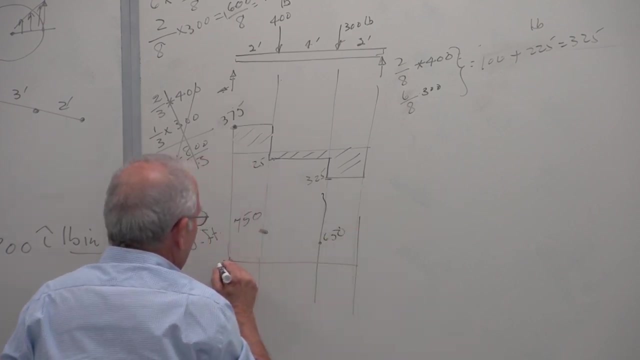 Okay, Now, hopefully things will come out right, So 375.. Okay, All right, All right. And the maximum moment here is this times 2, which will give us 0,, 5, 70.. And the maximum moment here is 325 times 2, 650. 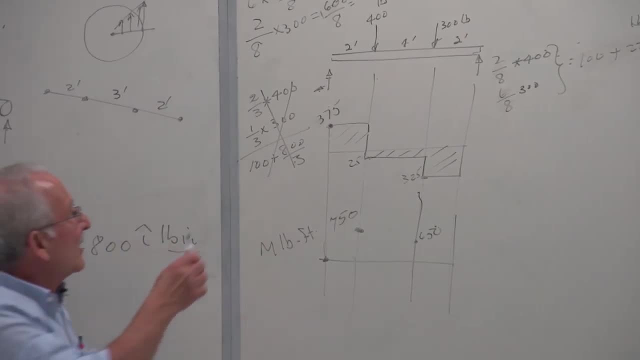 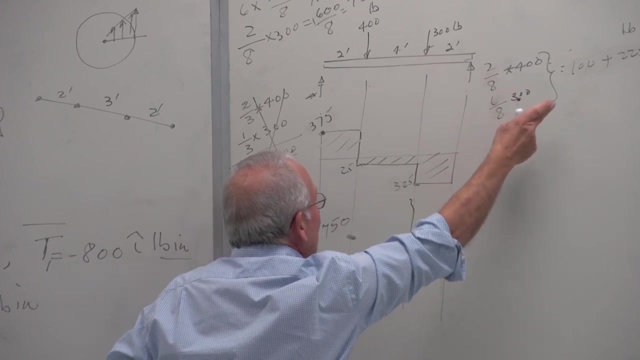 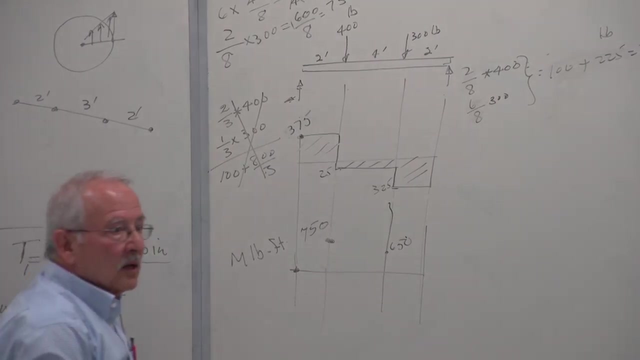 Does everybody know where I got those numbers from? This times, that, that times, that This times? that gives me 325 times 2,, 375 times 2 gives me 750.. So how do I go between these two points, Straight line or curved line? 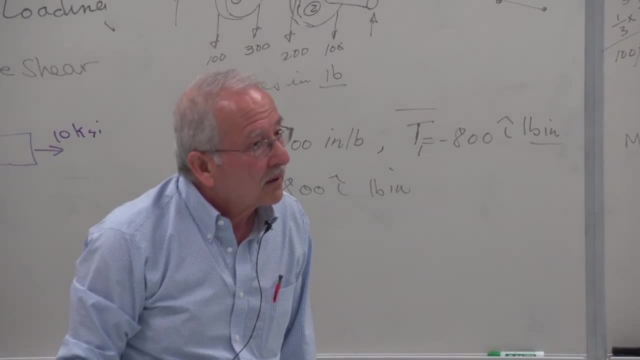 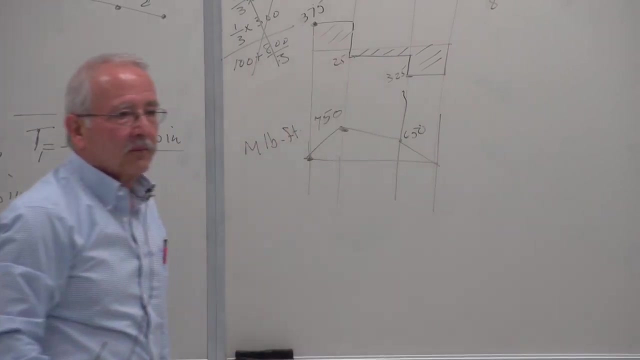 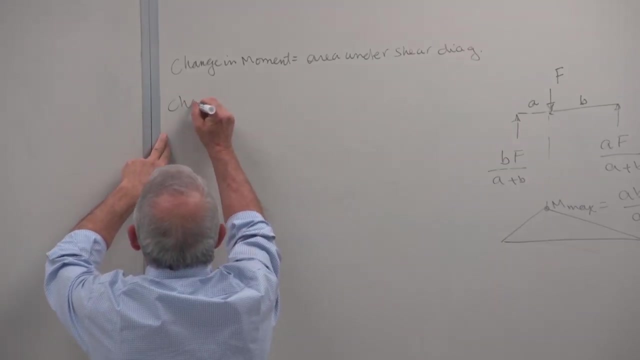 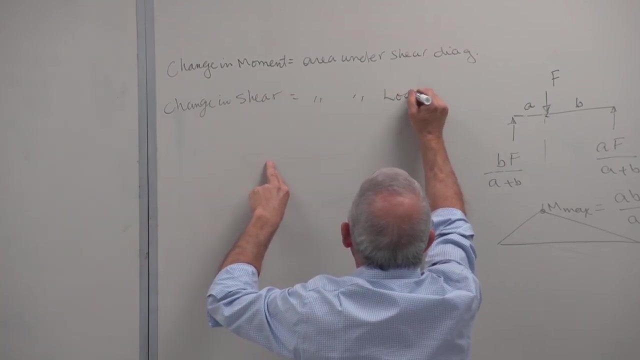 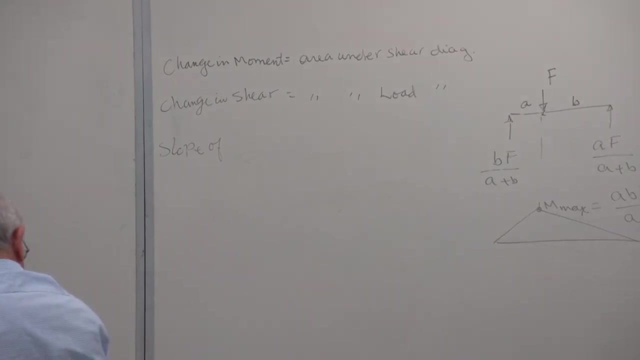 Straight. Why? Because the shear force is constant. Because the shear force is constant, So we go here, We go there And then we go there, Like that. So continuing on this Change in shear equals area under load diagram, Slope of. 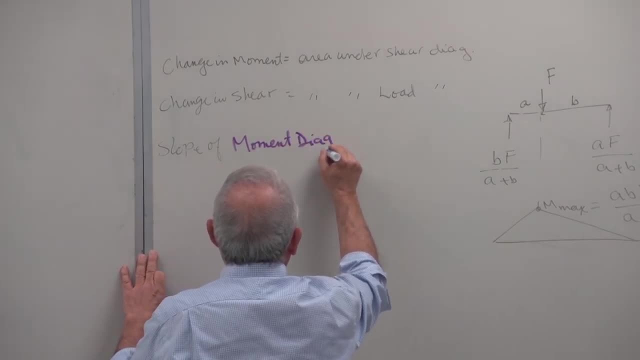 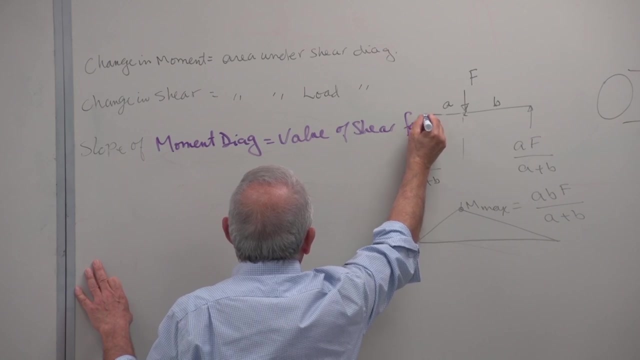 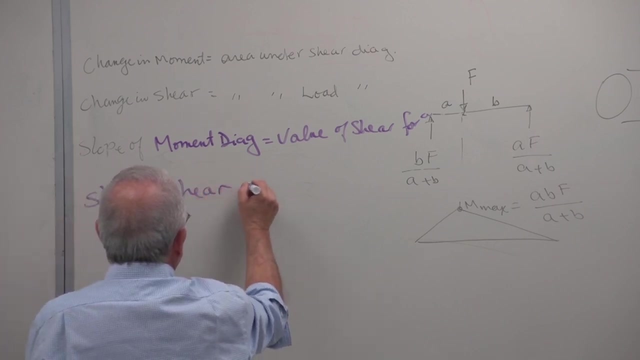 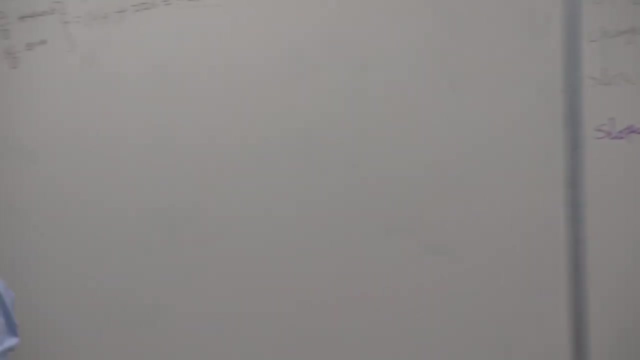 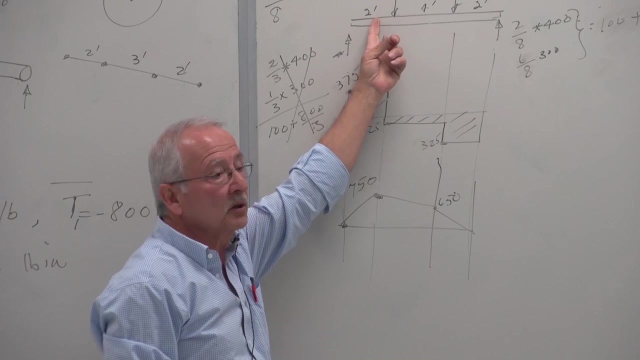 moment 0.. Diagram equals value of shear force And slope of shear diagram equals value of load. So the slope of the moment, the slope of the shear diagram here is 0.. Because there is no load here, This is free of load. 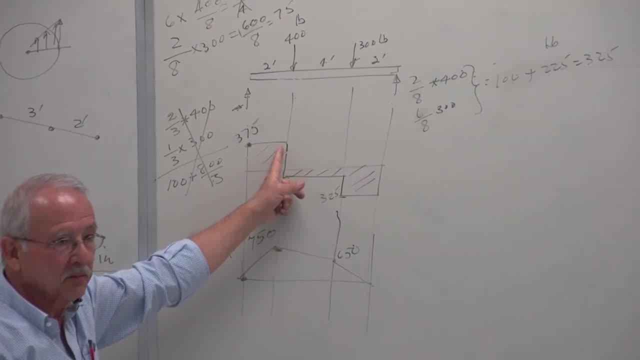 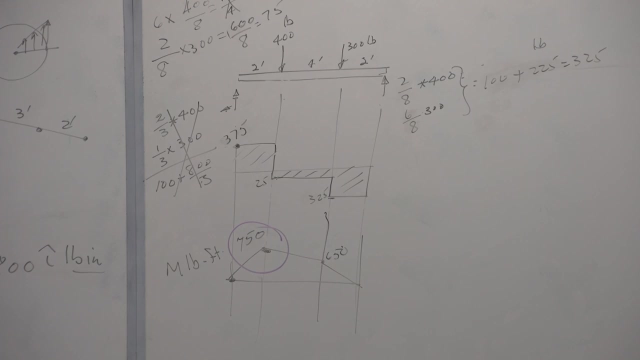 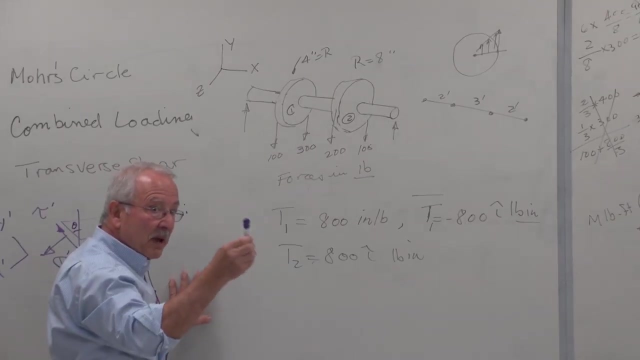 Slope of the moment diagram is constant because shear is constant. So now that you can see, this is our maximum moment. we said the maximum shear stress occurred between here and here. Since the maximum moment occurs here, then we should be looking at this section, right? 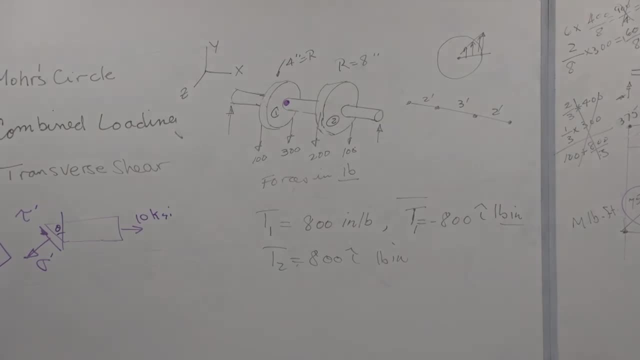 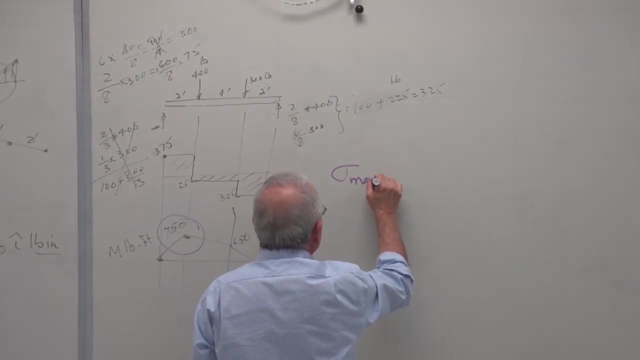 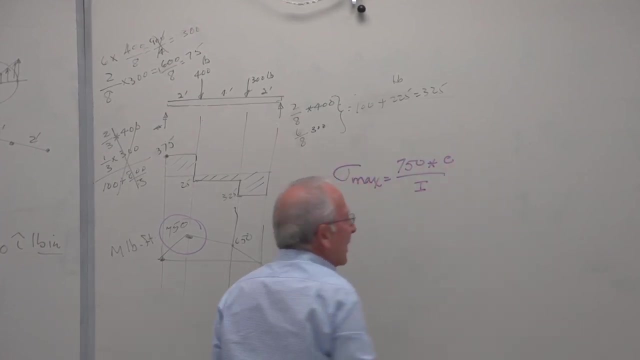 there on the right hand side of pulley, number 1.. And sigma max will be equal to, in this case, 750 times c divided by i. C and i I don't have because I didn't give you the diameter of the shaft. 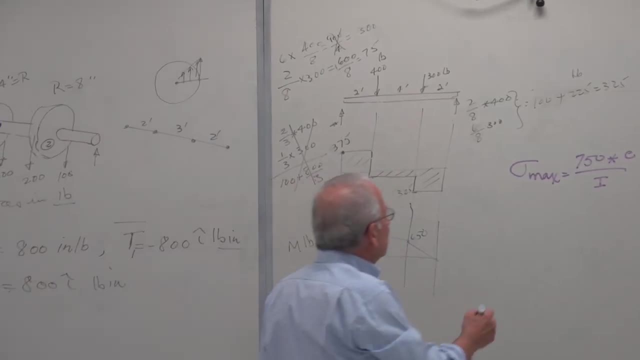 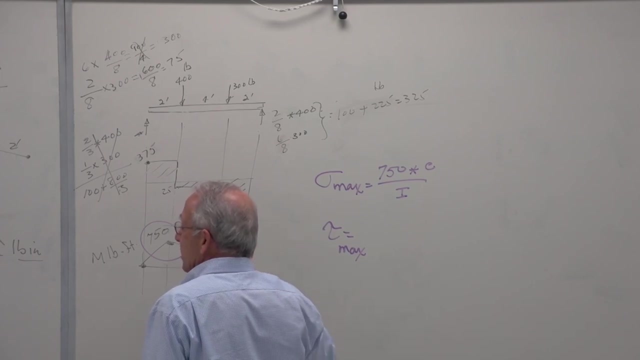 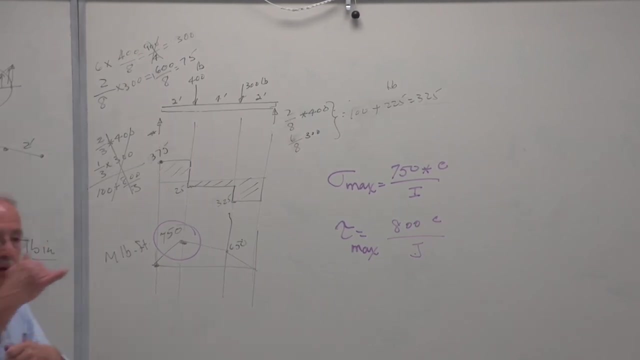 Once you have these two And tau, of course, we can calculate that 0. Tau max, that means the tau on the surface is equal to 800 c over j. Once you have these two, you're back to Mohr's circle with your sigma x, sigma y and tau. 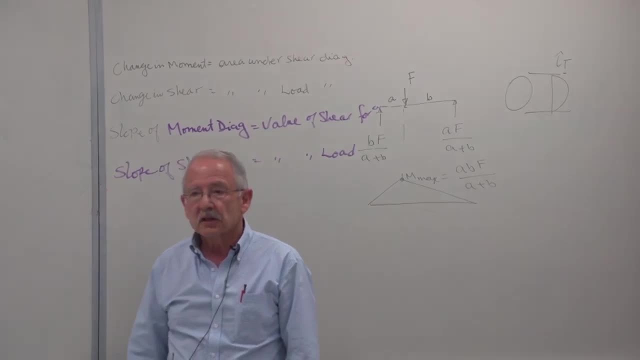 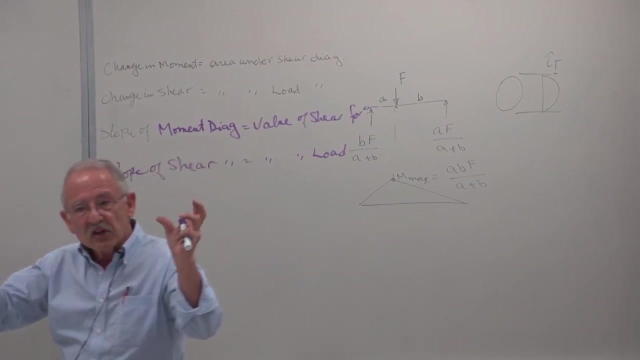 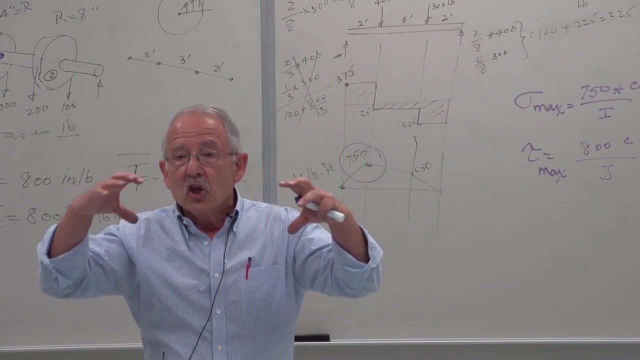 xy, Except that In this case, 0. Tau max, there is no sigma y or sigma z. Whenever you have bending of shafts or bending in general, it doesn't have to be a shaft. It could be a square, cross section, rectangular, I-beam. 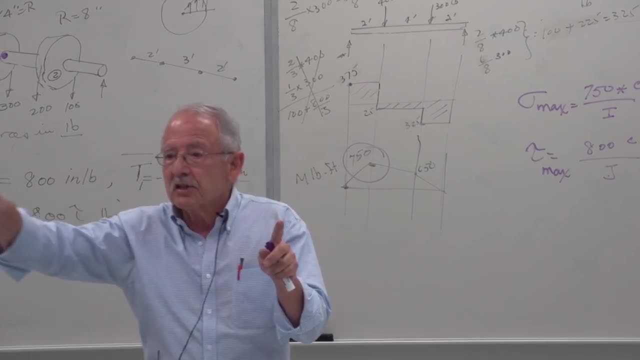 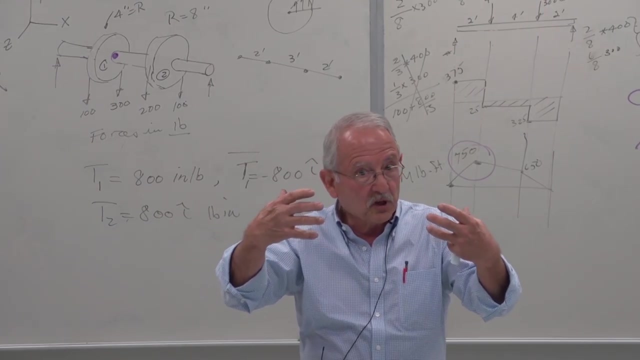 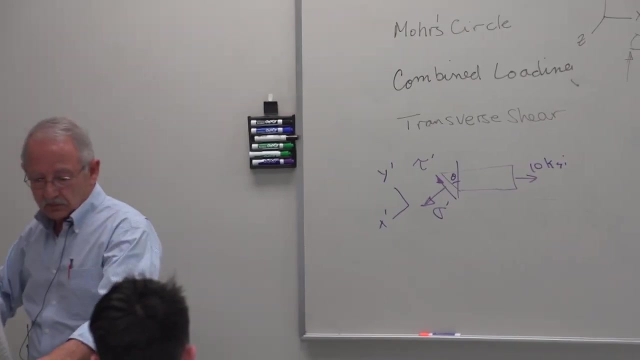 If you have bending, the only stress is along the axis. normal stress is along the axis of the shaft in bending. It doesn't matter whether you bend it like this or like that. 0. Tau max, 0. Tau max. 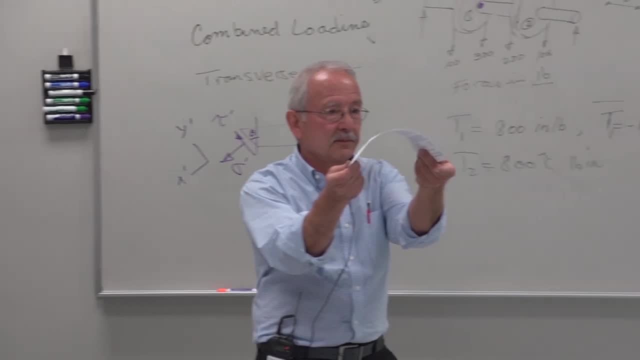 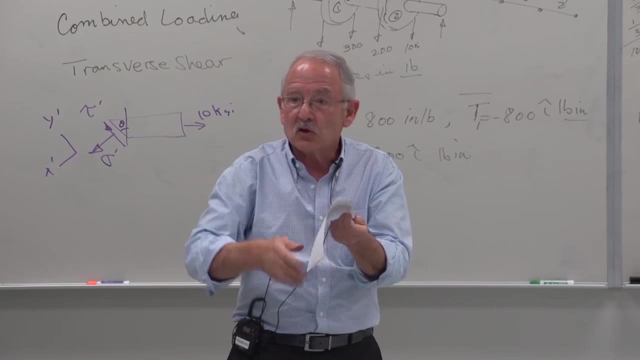 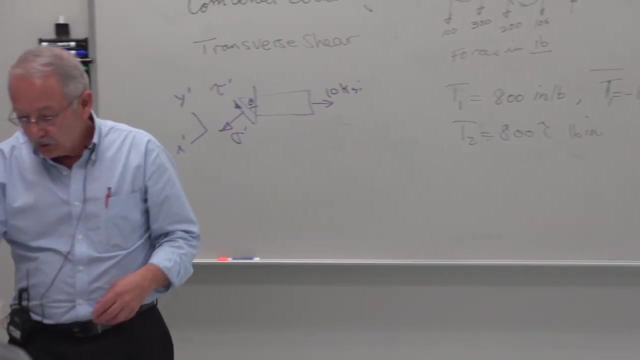 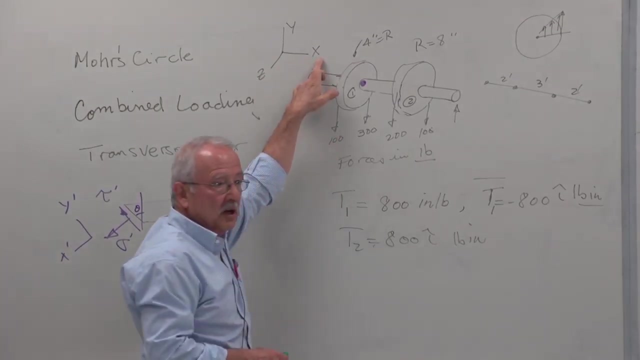 0. Tau max. Either you bend it like this Or you bend it like that, Normal stress is always along the axis of the shaft. It will always be along the axis of the shaft. So don't, When you have shafts like this- and this is your x, y, z- your only normal stress is in. 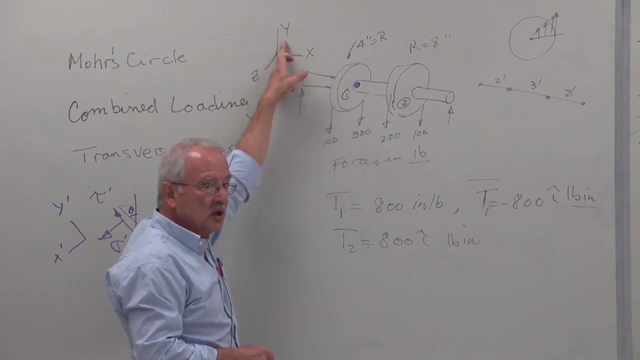 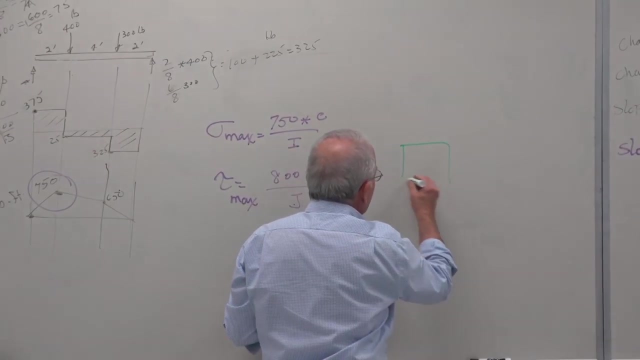 the x direction, along the axis of the shaft. There is no sigma y, is no sigma z, so don't come up with those. Your Mohr's circle, in this case, will look like this, or sorry, your element will be one normal stress and one shear stress, And 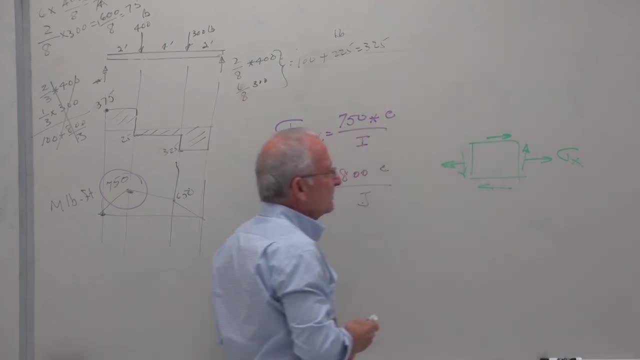 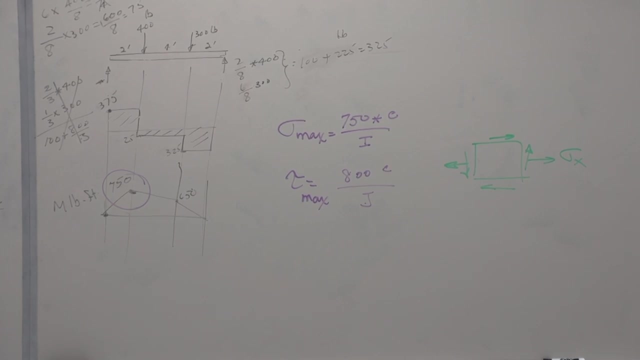 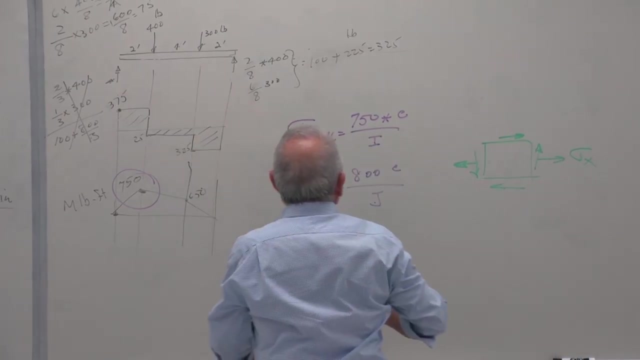 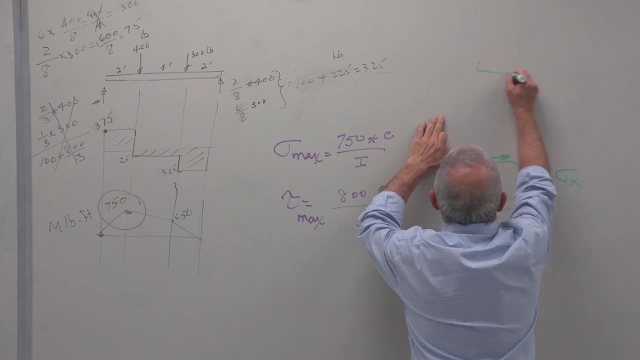 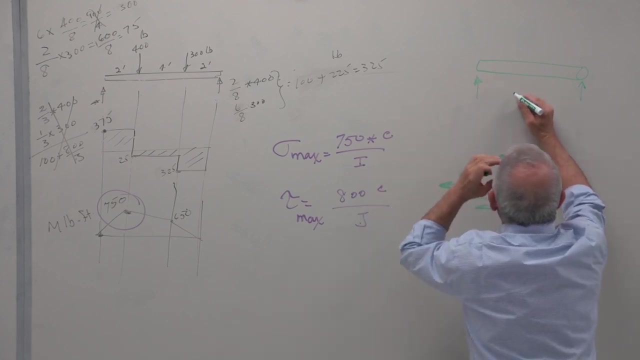 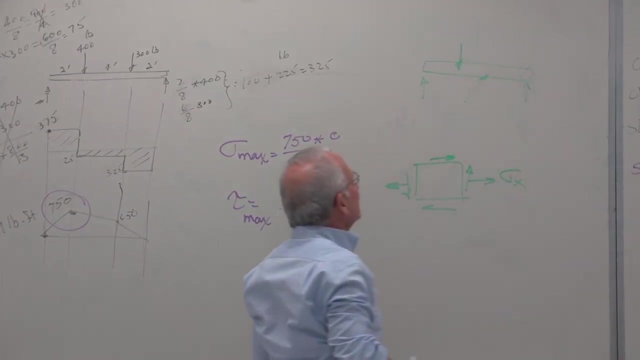 this is sigma x in our case. Any questions Now, what if, rather than these loads being like that, they were like this, Still simply supported And you have a load here like so and a load here like so. The two loads are not in the 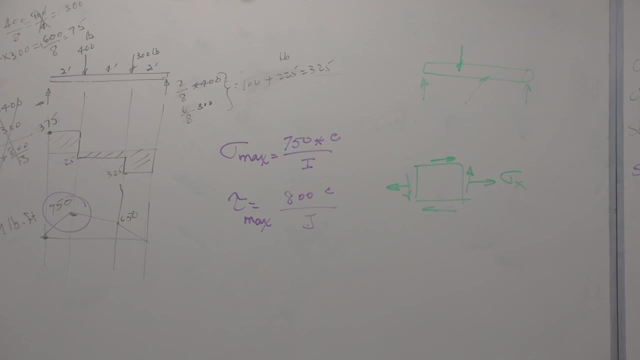 same plane. One of them is in the x direction and the other one is in the z. sorry, one of them is in the y direction, the other one is in the z direction. So this is your x axis. That's the load in the y direction. load in the z direction. 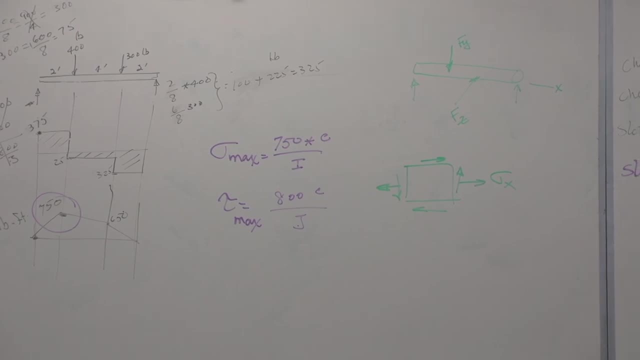 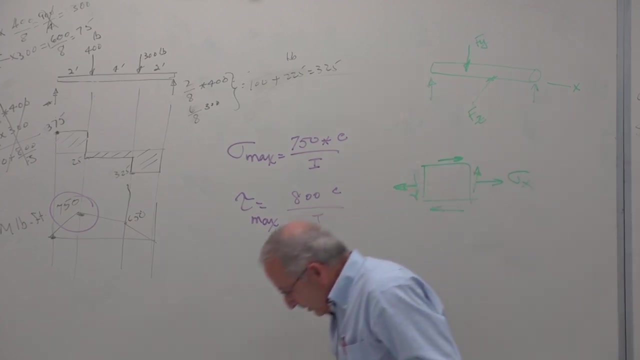 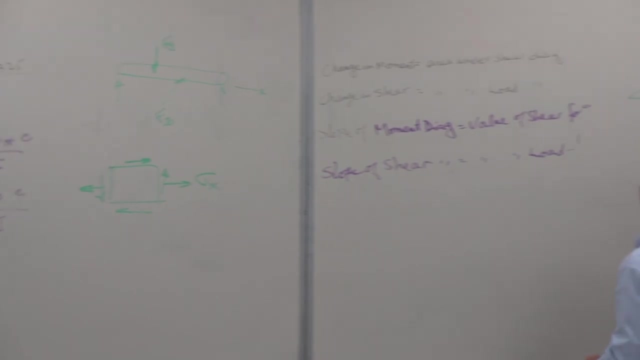 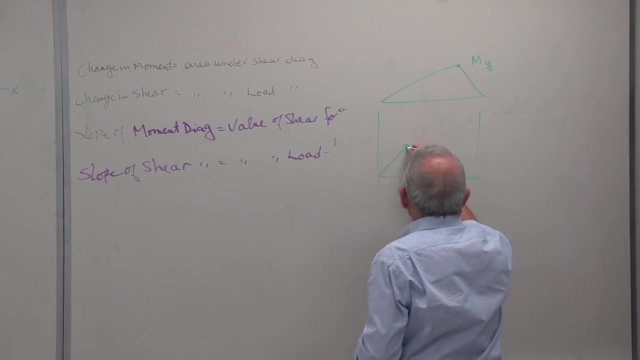 You guys did that in 2.19, right? Yes, I'm sure you did So. what you do in this case is draw two moment diagrams, One for each of these, And you end up with something like this: Say: moment in the y direction, Our moment in the x direction, of course, is torque. 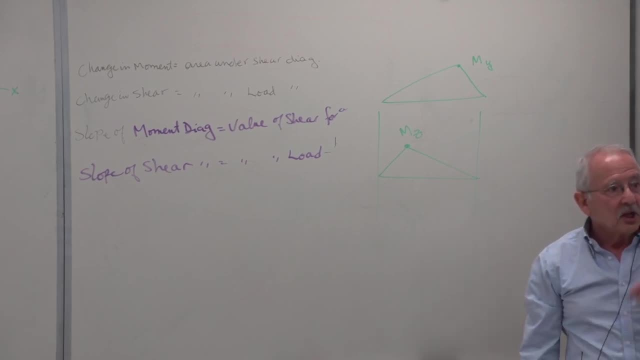 Moment in the z direction. The maximum moment occurs either here or here, And the way you find it Come down here call this m y prime, and then you combine. you say m y max, square root of m y squared plus m y prime squared. 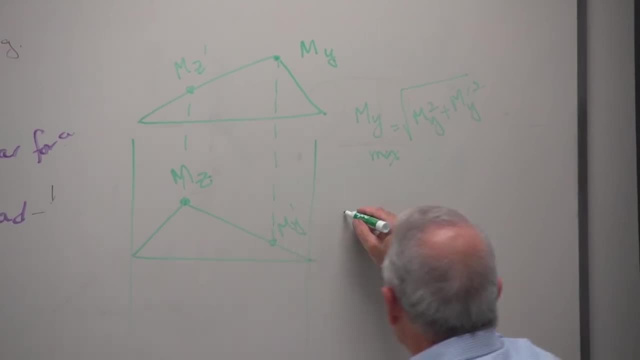 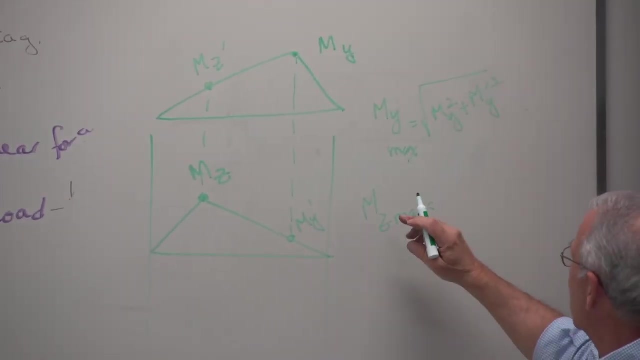 Same thing here: m z prime, m z max equals. I shouldn't actually call them. I guess it's okay. I'll call them: m z max equals the square root of m z squared plus m z prime squared. You compare these two. 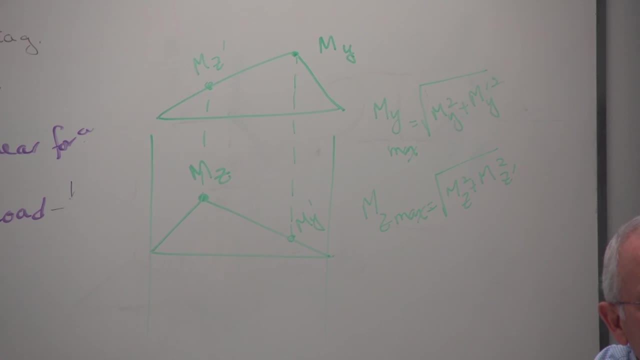 Whichever is larger, that's your maximum moment And wherever that occurs, that's where the maximum normal stress occurs. That's what you use in this equation. in that case, rather than 750, whatever that comes out to be, That ring a bell, of course, from 219.. 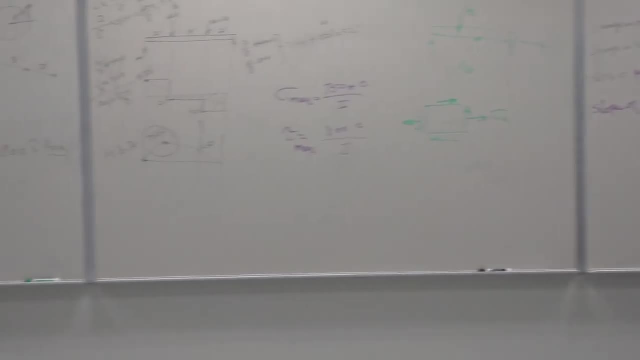 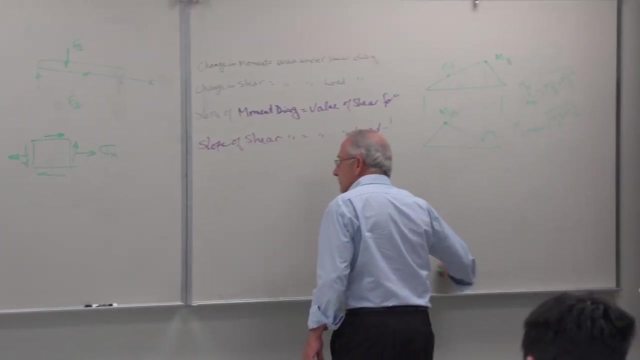 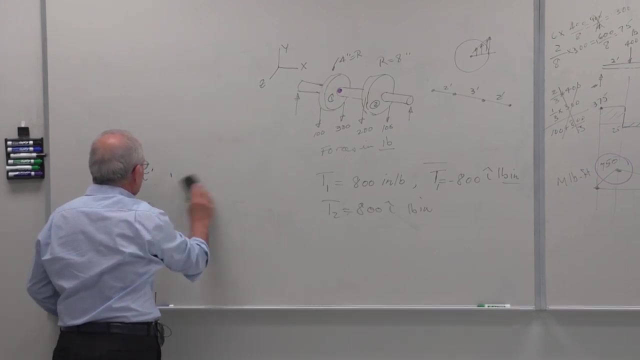 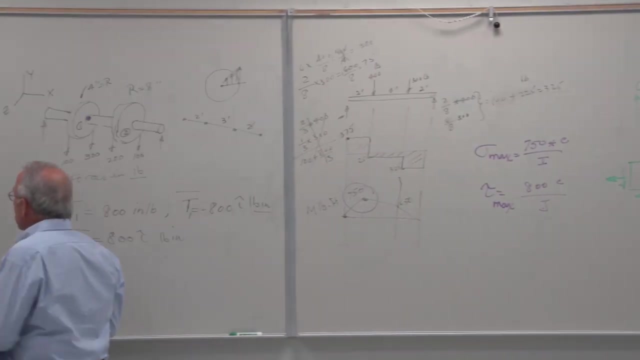 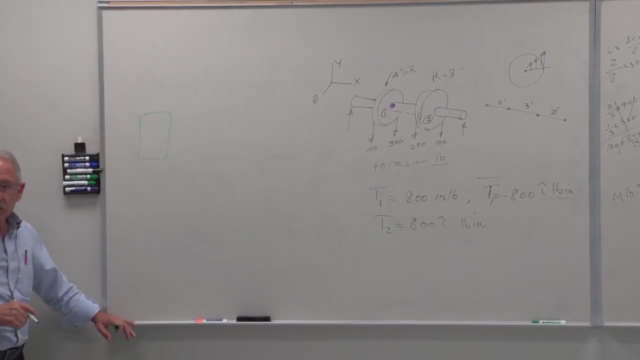 Any questions? I have three minutes. let me talk very quickly about transverse shear, And I forego the preliminaries. I'll tell you this: I had a picture drawn with transverse shear. I guess it's not here. This is your cross section. 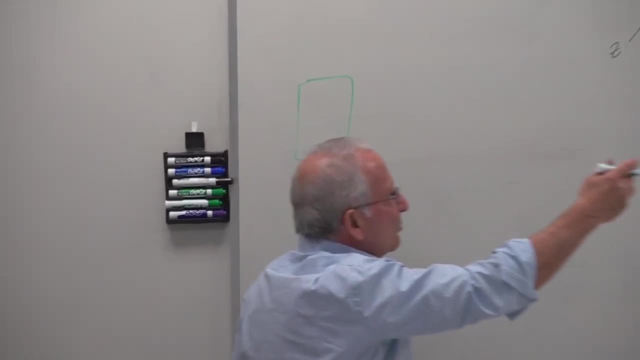 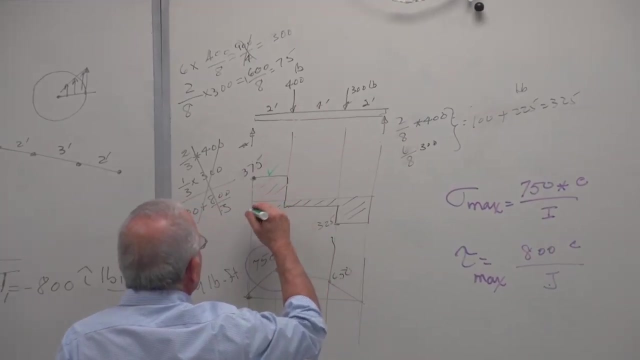 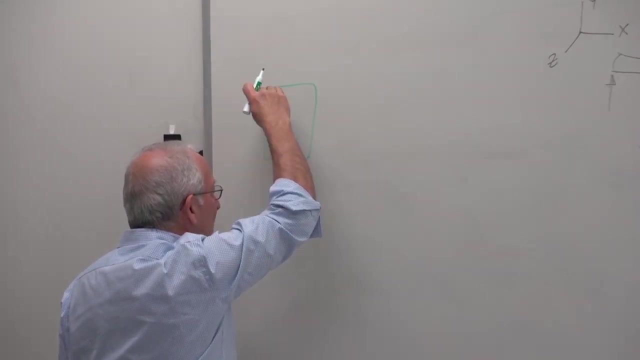 Shear stress will occur in beams loaded like that at various sections. wherever you have a shear force, There will be a shear force, So you'll have a shear stress. The shear stress acts both on a vertical plane and on a horizontal plane. 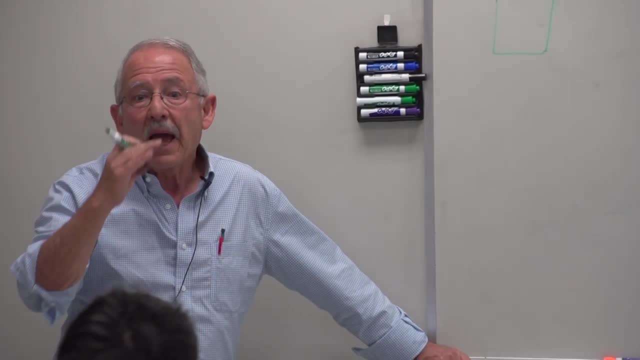 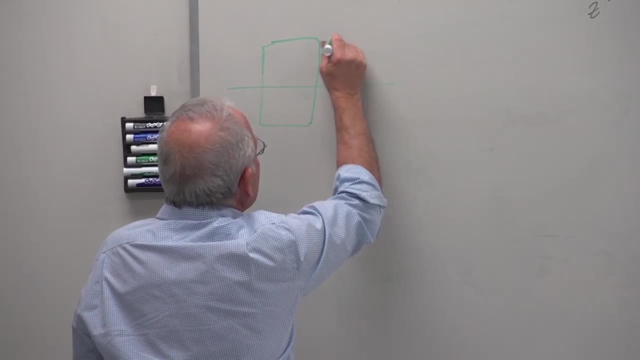 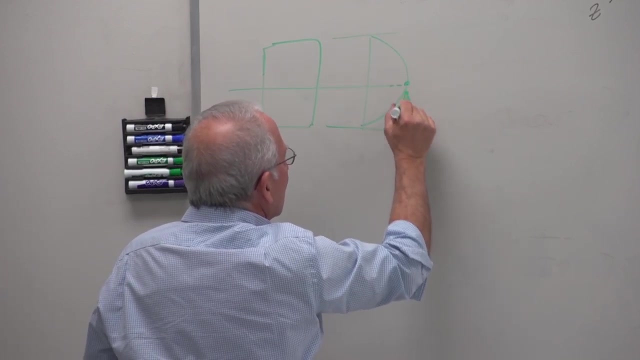 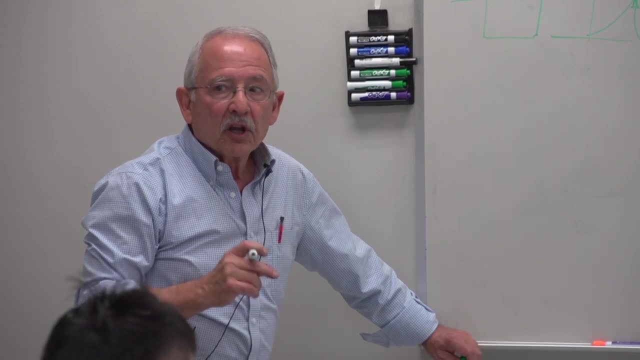 Because shear stresses must occur in pairs And on two perpendicular planes. The magnitude of and the distribution of the shear stress is like this: It's maximum at the normal level, Okay, Okay, So you'll have a shear stress at the neutral axis. 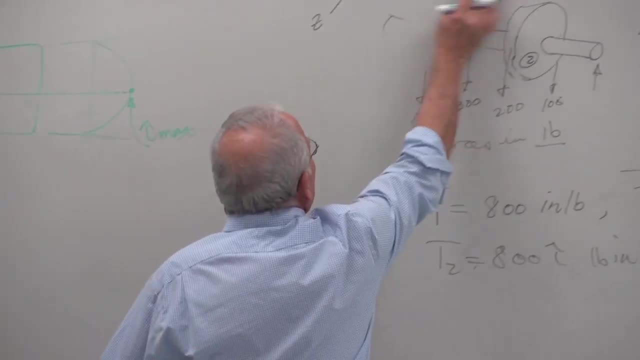 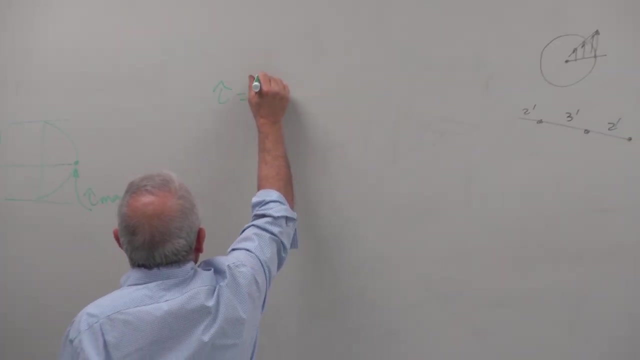 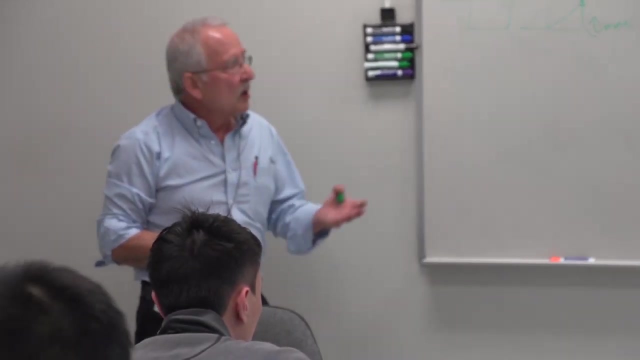 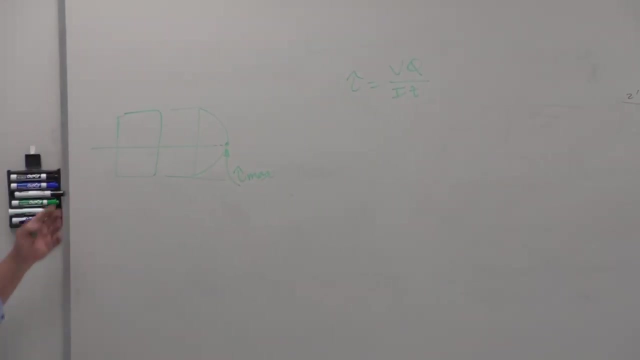 Its value is found using this equation: V is the shear force, I is the moment of inertia of the cross section about the neutral axis. T is the thickness of the cross section, wherever you want to find this cross. Now, if the thickness varies here, 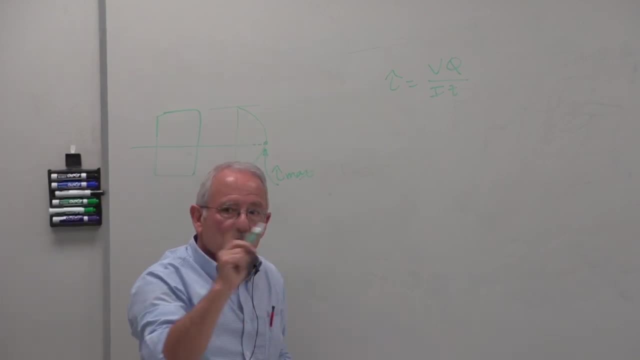 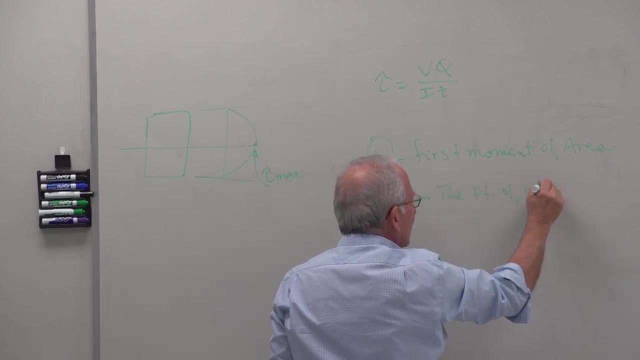 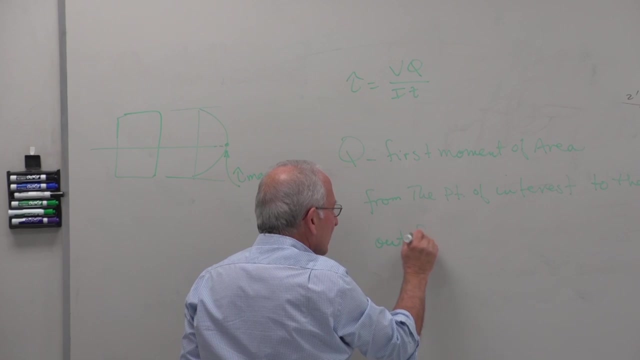 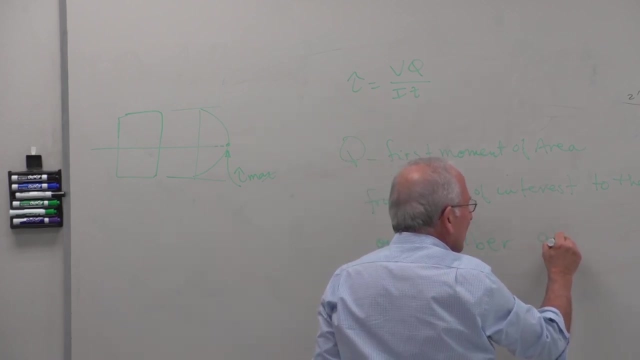 of course this shape will change too. Students have most problem with the value of Q. This is first moment of area from the point of interest to the outer fiber. Any outer fiber Doesn't have to be the closest About the neutral axis. 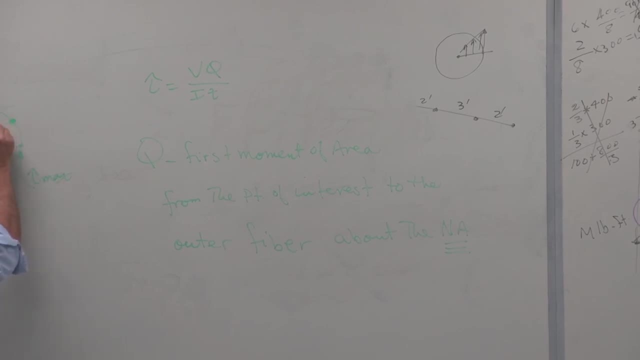 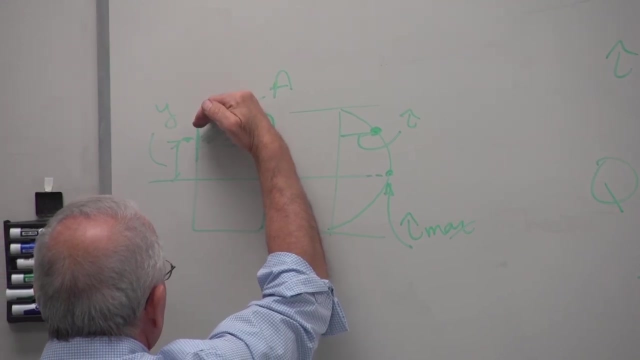 So, for example, if you want to find this shear stress, this tau Q will be. we'll call that A times that distance, Y Moment of the area from the point of interest to the outer fiber, Either this outer fiber or this outer fiber. 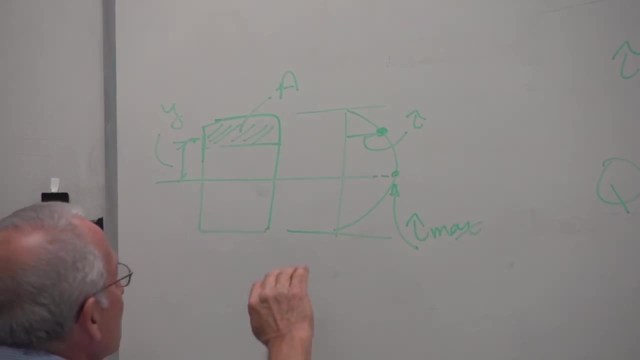 Doesn't matter, You can go up and down exactly the same time. About the neutral axis, Therefore, in this case, Q is equal to A Y, Whatever the value of Y is, Which you can find Just using simple geometry. Okay,